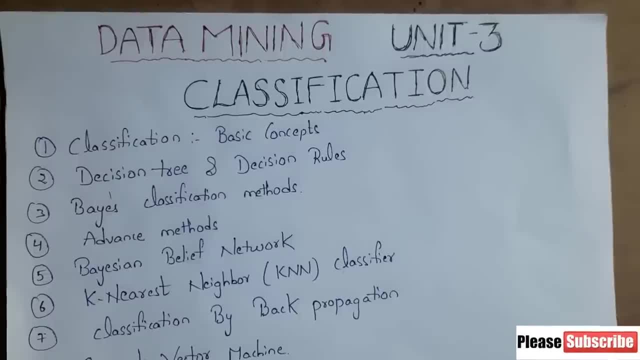 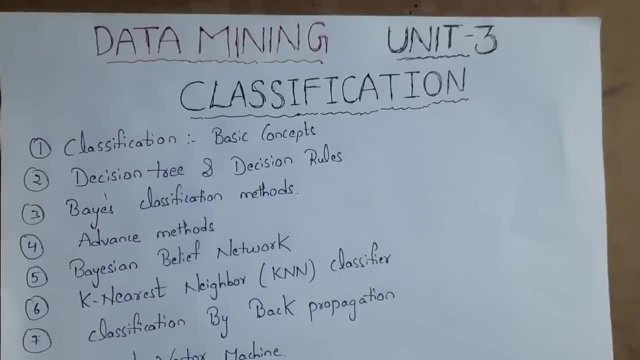 dresses are arranged in various categories, like sheds in boy's section are arranged in one side and dresses in girl's section are arranged in another side and kids section one side, and so on, so that I can easily find out my required dress, so that searching becomes easier and I can save my 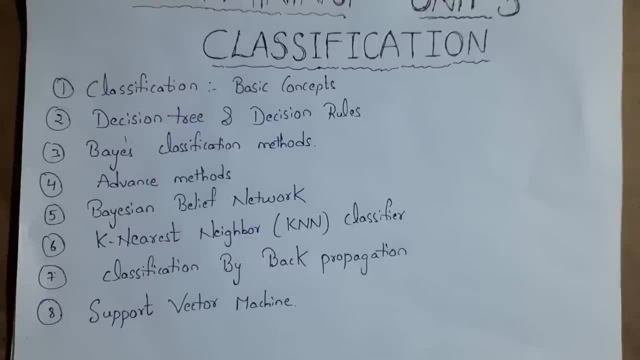 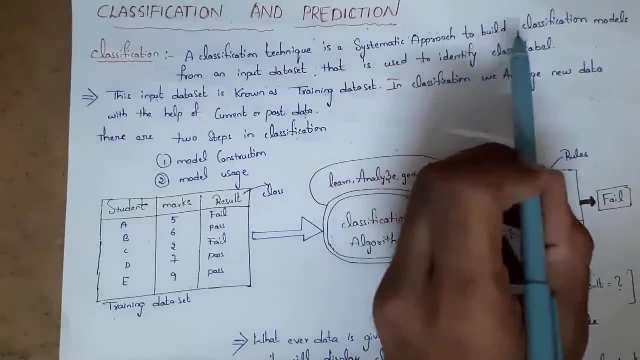 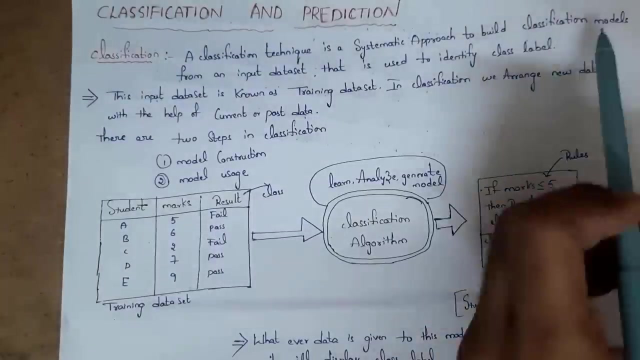 time. Similarly, in data mining also, we classify data into various categories so that searching data becomes easier. A classification technique is a systematic approach to build classification models from an input data. By using classification technique, we can build classification models, We can create classification. 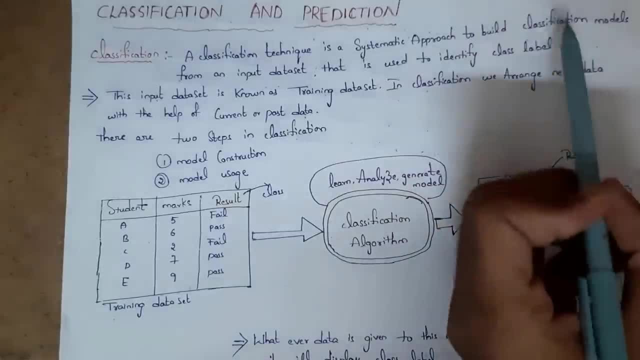 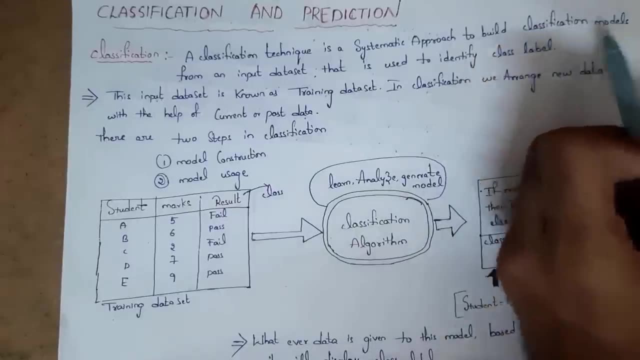 models by using classification technique. How we create this classification models. By using input data set, we create classification models and this classification model is used to identify class label. I will give an example so that you can clearly understand this definition. There are two. 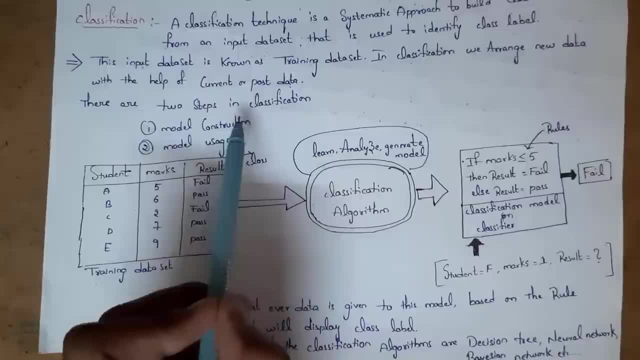 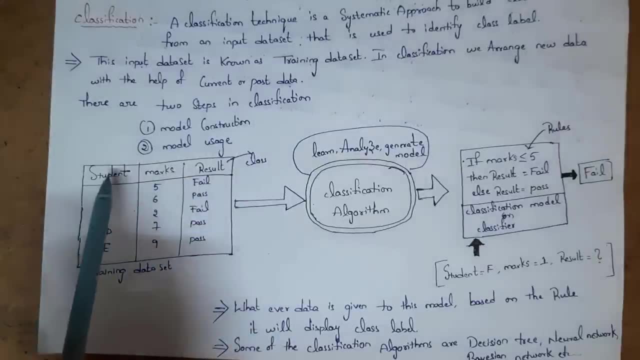 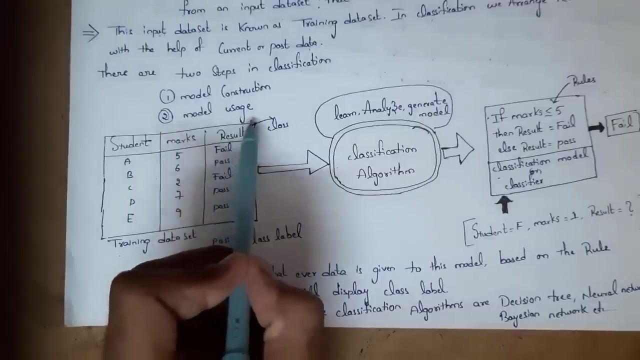 steps in classification. First step is model construction and second step is model usage. I took one input data set. That input data set contains three attributes. They are student marks and result. In any input data set we call last attribute as class. In this last attribute is result. So I call this result as. 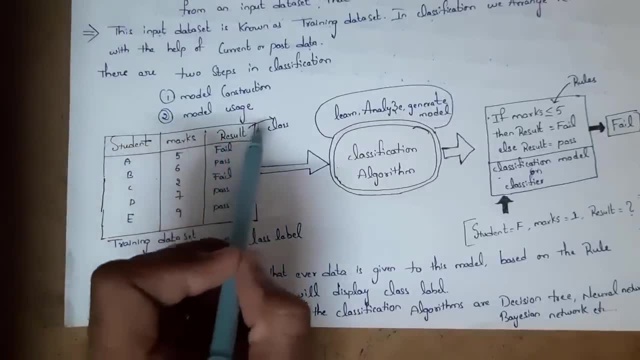 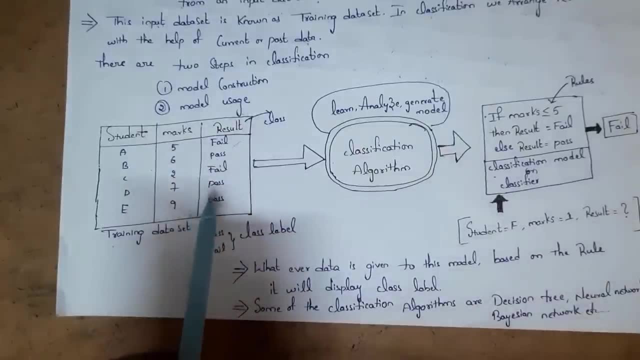 class and whatever the data that is present inside this class, we call this data as class label. How many class labels are present inside this class? There are two class labels present inside this class. They are fail and pass. Fail and pass. These are the two class labels. Now we need to send this input data set into this. 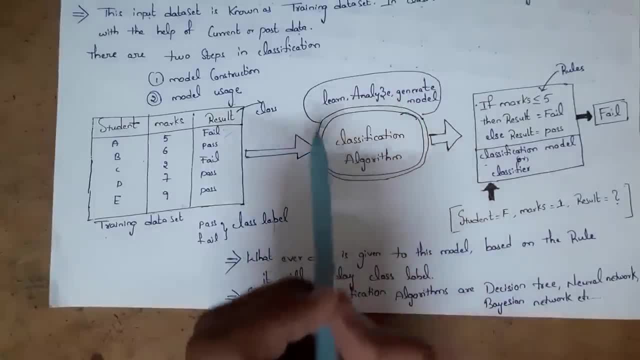 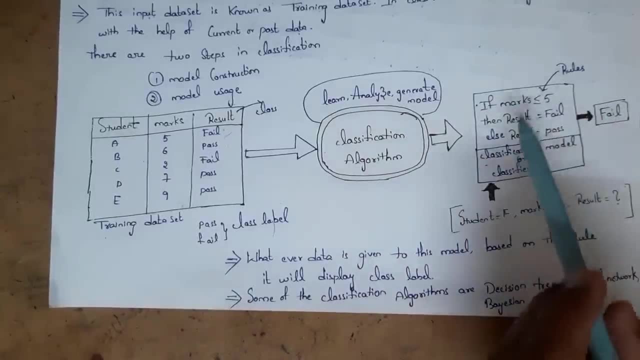 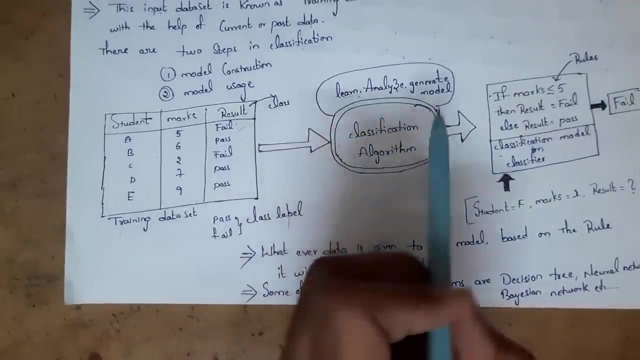 classification algorithm, so that classification algorithm will create classification model. We also call this classification model as classifier. Basically, this classifier contains some rules. Whenever we send this data set into this classification algorithm, classification algorithm will learn this data set first. How it will learn this data set? It will check each and every object. 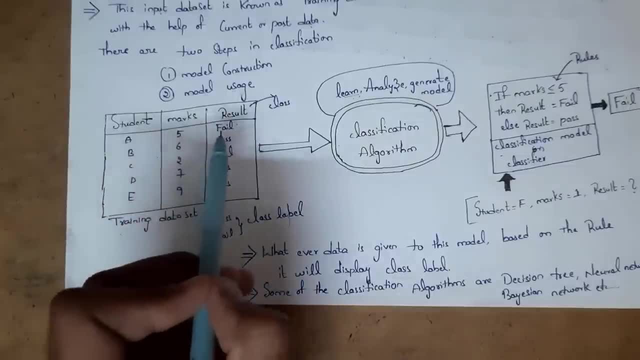 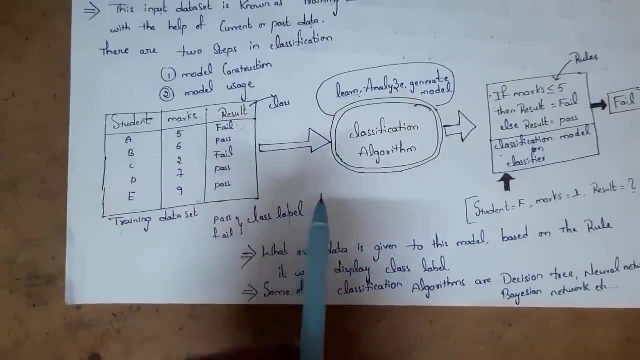 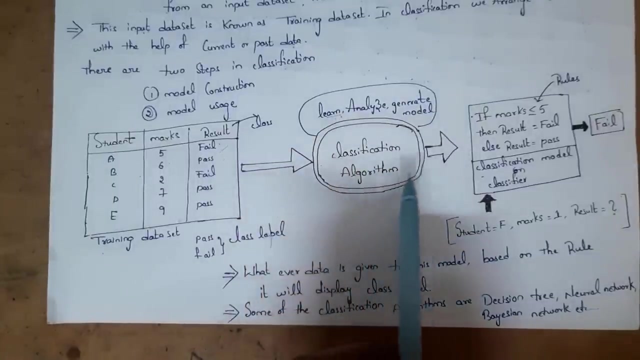 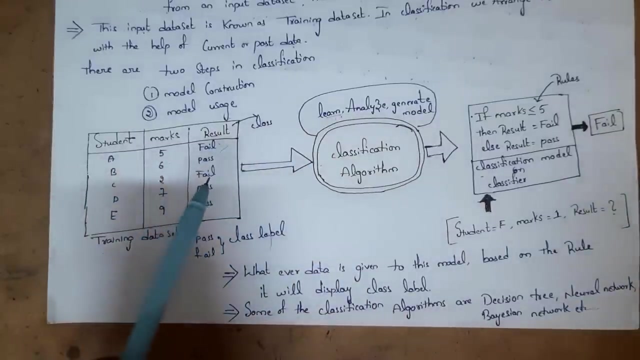 that is presented. For example, let's say we have small object which if we need to disperse and then write, if we need to disperse faculty, we need to set them down. They will write the name and click on any days of the day. 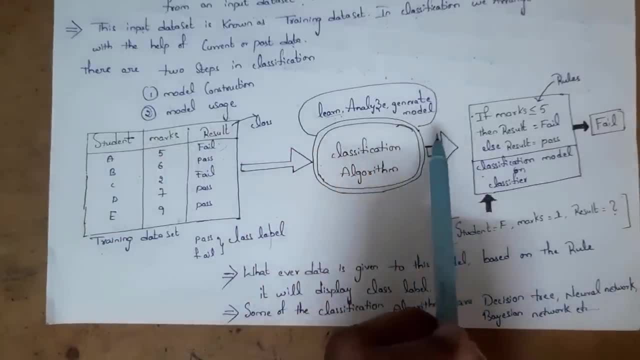 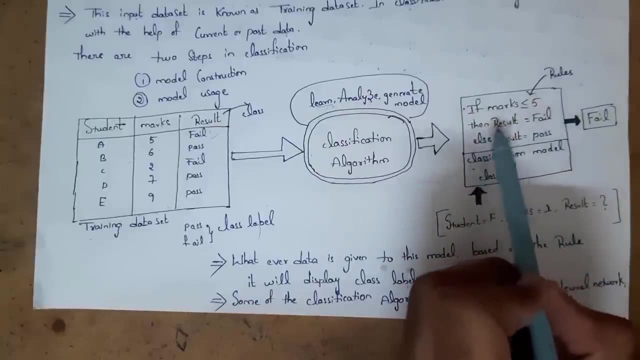 Like and libUI classification algorithm will create model for this. This model contain rules. Rule is nothing, but if max is less than or equal to 5, then result equal to fail. else result is equal to pass. We call this model as classification model or all. we can also call this model as classifier. This is 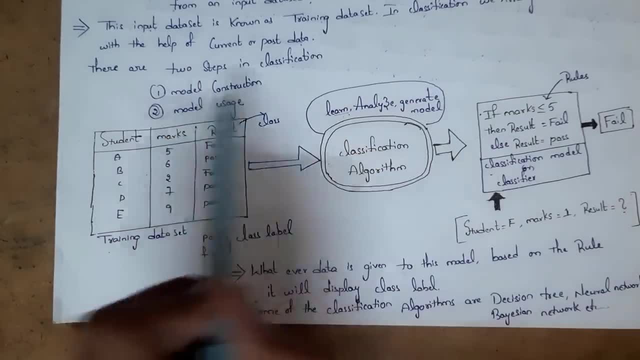 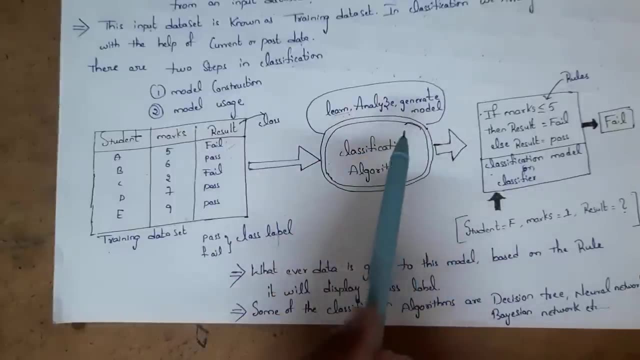 how we constructed model. This is first step, that is, model construction. We call this input data set as training data set because we are training this classification algorithm in order to generate model, So we call this input data set as training data set. After model construction, next step is: 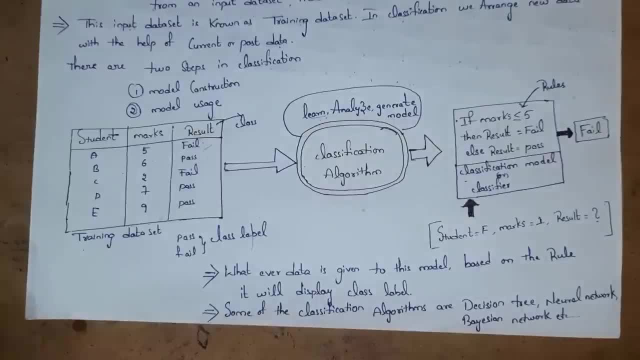 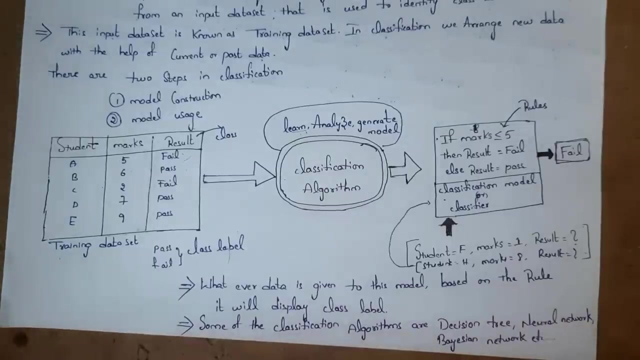 model usage- How we will use this model now. For example, I want to know result of one student. that student name is F. He got one mark. I want to know his result. Whenever I send this information into this classification model, this classification model will check the rule. What is the rule? 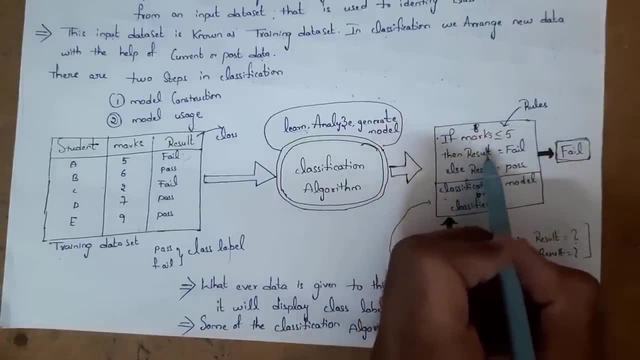 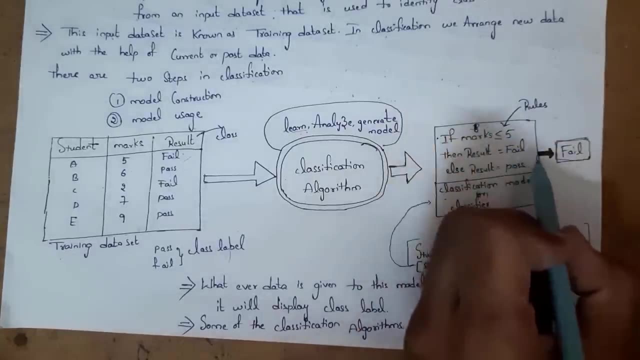 If marks are less than or equal to 5, then result is equal to fail. else result is equal to pass. Here student have got one mark, One is less than 5.. So result is fail. It will display result as fail. For example, there is another student, The. 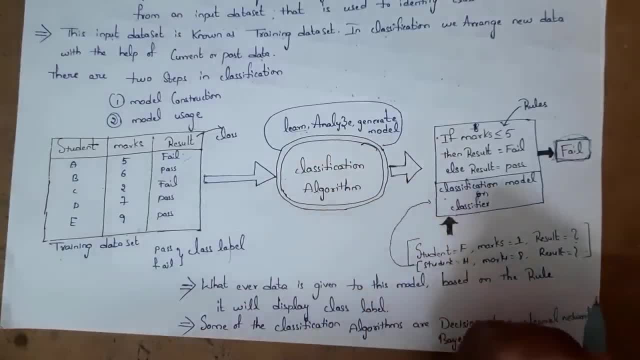 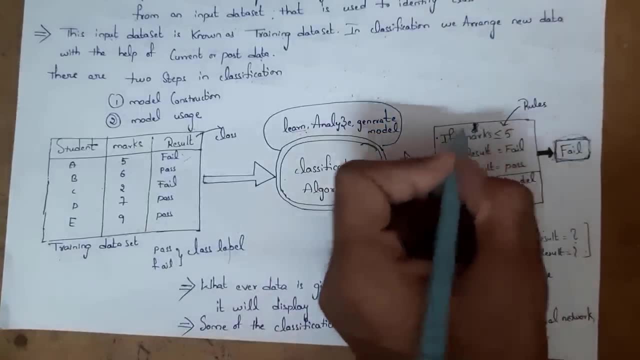 student name is H. He got 8 marks. I want to know his result Whenever I send this information into this classifier, this classifier will check that is. student got 8 marks. 8 is not less than or equal to 5.. 8 is greater than 5.. So result is pass. 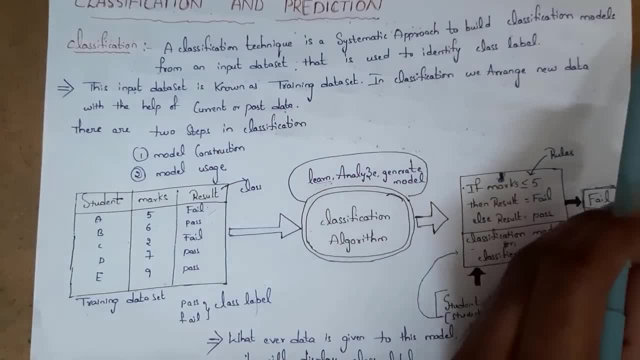 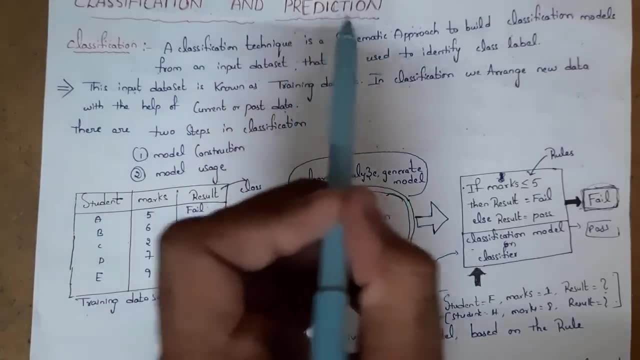 Classification technique is a systematic approach to build classification model from an input data set. We are building this classification model by using this input data set that is used to identify class label. Fail and pass- this are the class label. By using this, we can find class label. 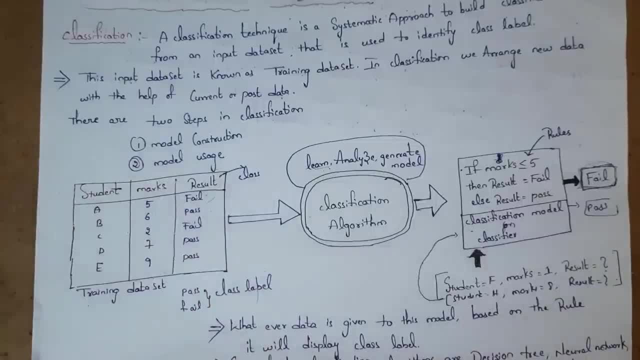 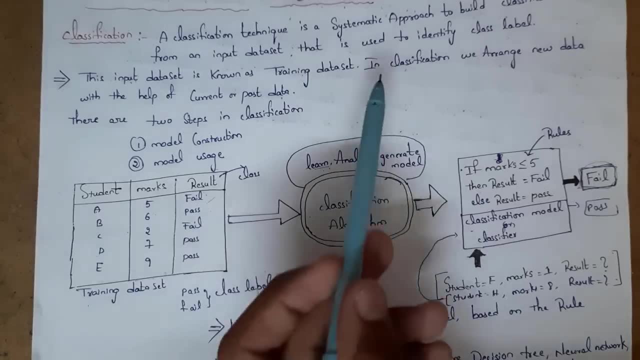 This input data set is known as training data set. I already said before, This classification algorithm will learn from this input data set, So we call this as training data set. We are finding this new result with the help of current or past data. We are finding this new. 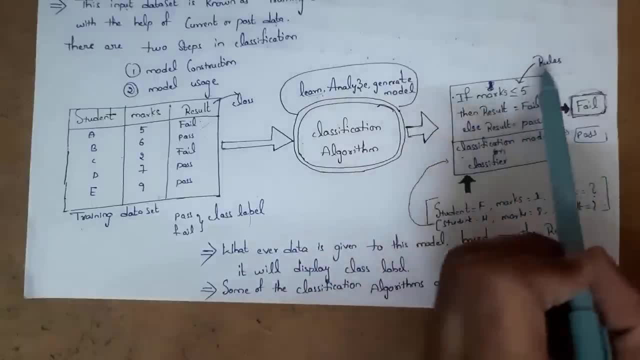 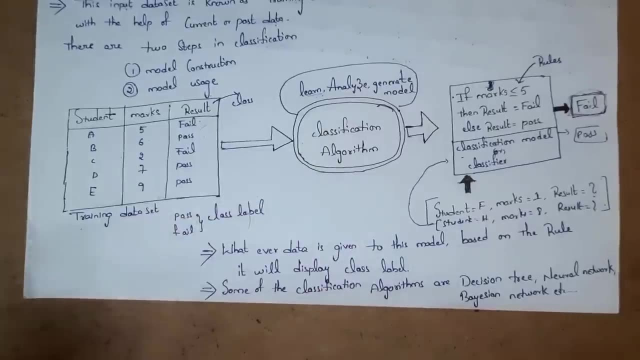 result, with the help of past result And whatever the data that is given to this model, based on the rule it will generate class label. Class label is nothing but result. Some of the classification algorithms are decision tree, neural networks, etc. Next topic is prediction. Prediction is a. 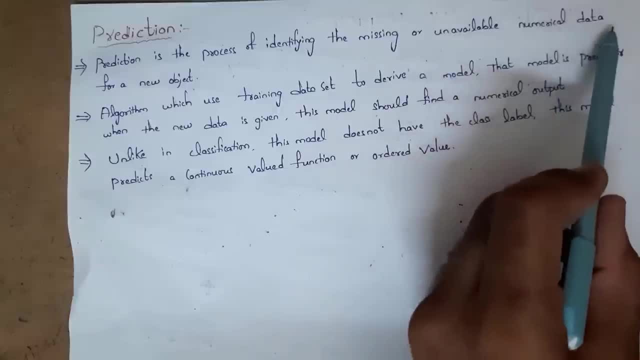 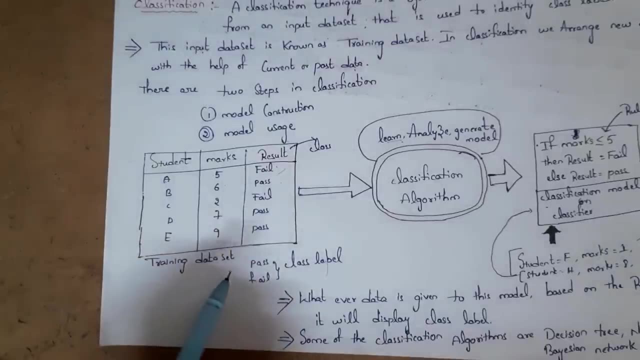 process of identifying missing or unavailable numeric data for a new object, Whereas in classification we are finding class label That is nothing but result. So we are finding class label That is nothing but true or false or pass or fail, Yes or no. Like that, These all are known as class. 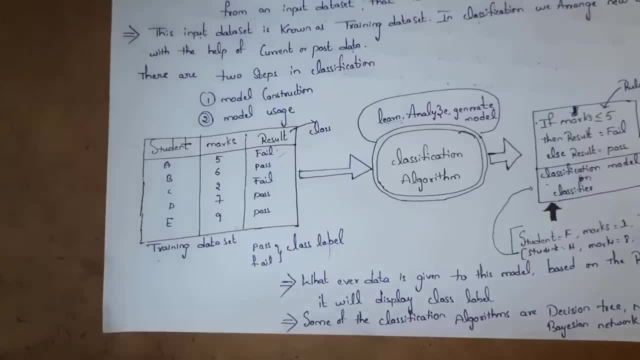 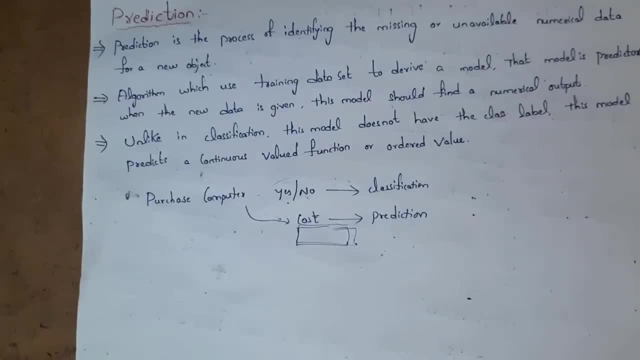 labels. We are finding this, But whereas in prediction we are finding missing values or unavailable numeric data. For example, if person want to purchase computer, whether he will purchase computer or not- that is either yes or no- is known as classification. We are finding. 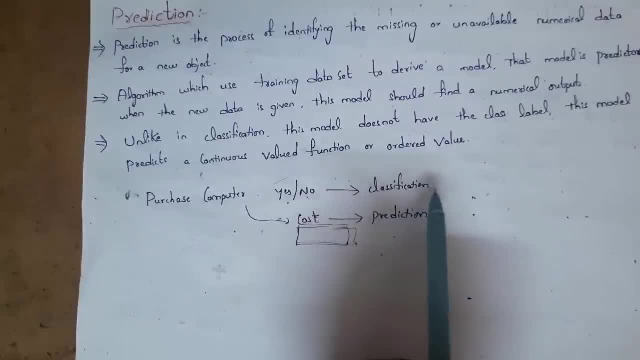 class label. That is yes or no. It is known as classification. But how do we know that it is true or false? We are finding class label. We are finding class label- How much cost that person is going to spend in order to purchase this computer. This is known as. 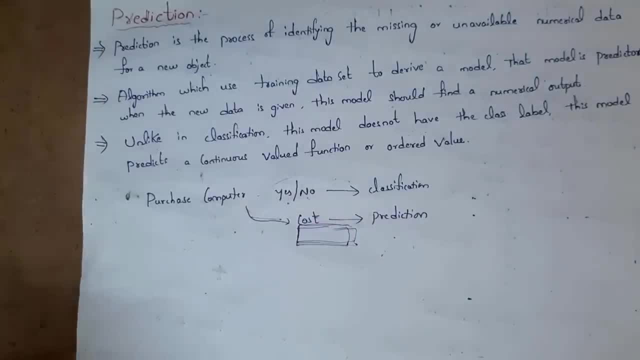 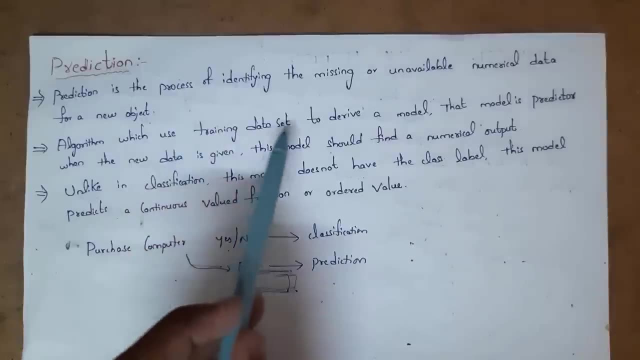 prediction, Because we are predicting the cost. We don't know what is the cost, So cost is missing value. We are finding this, This is known as prediction Algorithm, which use training data set to derive a model That is predictor In classification, whatever the input data set. 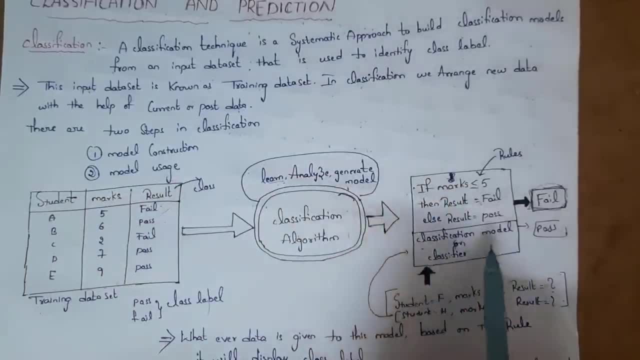 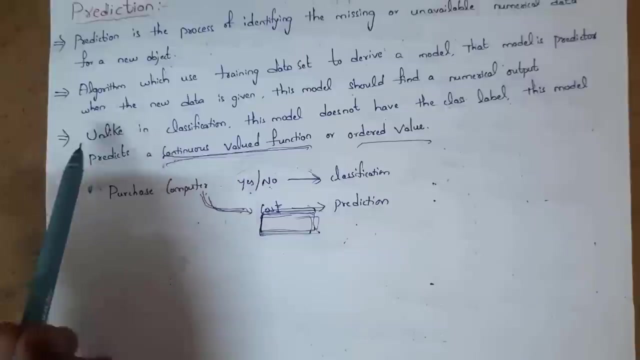 that is used in order to create model. We call this model as classification model or classifier. But in prediction we call this model as predictor Because it is predicting the value. And whatever the new data that is given to this predictor, it should find a numeric output, Unlike in. 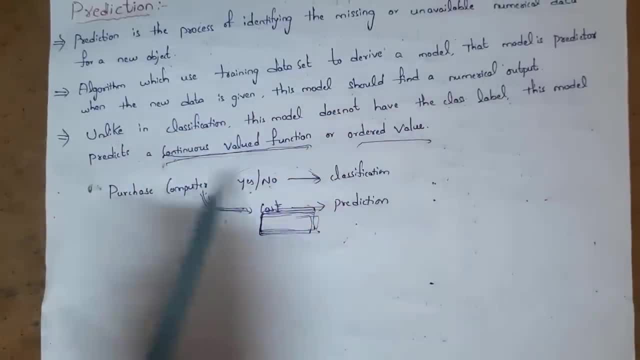 classification. this model does not have any class label. I already said in this example, prediction contain class label. That is either yes or no, true or false, like that. But prediction do not contains any class label And this model predicts continuous valued function or 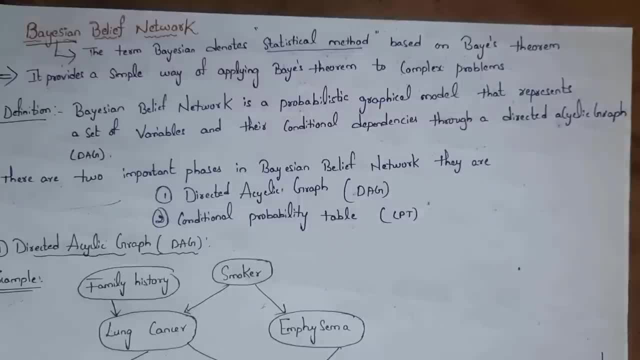 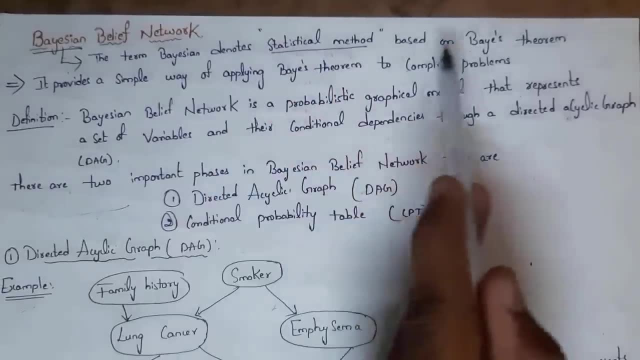 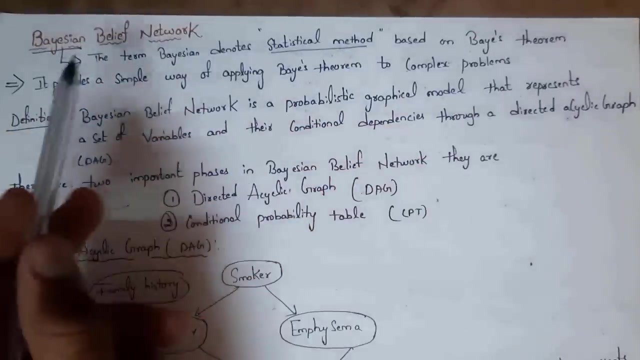 ordered value. Next topic is Bayesian belief network. The term Bayesian denotes statistical method. In statistical method we represent complex data in simple format and is based on Bayesian theorem. This Bayesian belief network provides a simple way of applying Bayesian theorem to complex problem In Bayesian. 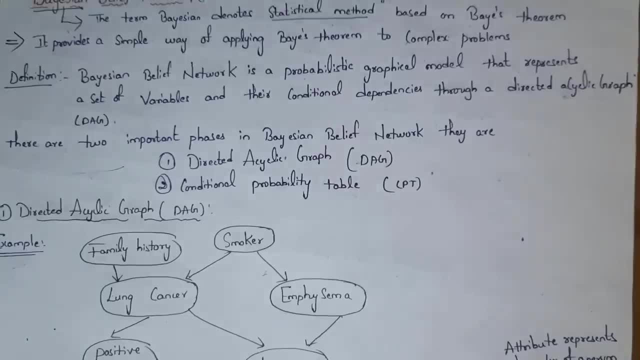 belief network. we apply Bayesian theorem to complex problems. Before explaining definition, I will explain phases of Bayesian belief network Totally. there are two phases in Bayesian belief network. They are: first: one is directed acyclic graph- Shortly we call it as DAG- And next one 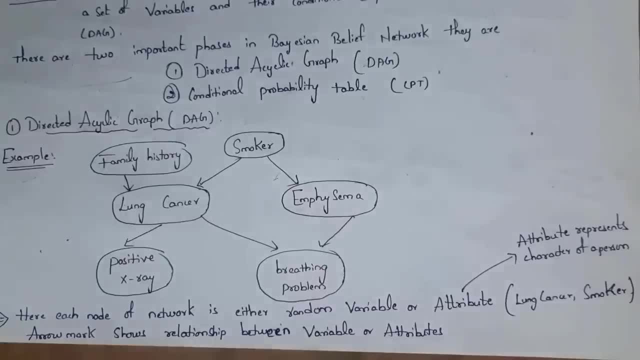 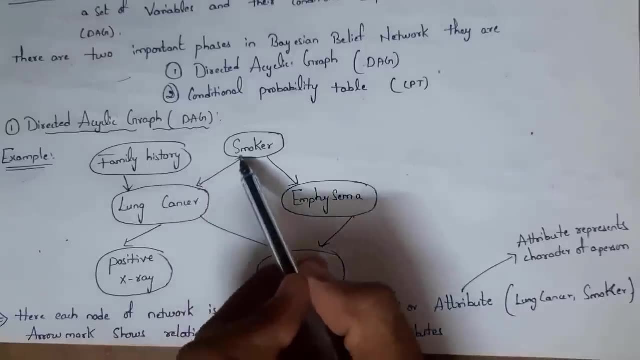 is directional probability table. We call it as CPT. At first I will explain what is directed acyclic graph, that is DAG. Directed graph mean graph which contain directions. That is nothing but graph which contain arrow marks is known as directed graph. And acyclic mean graph which do. 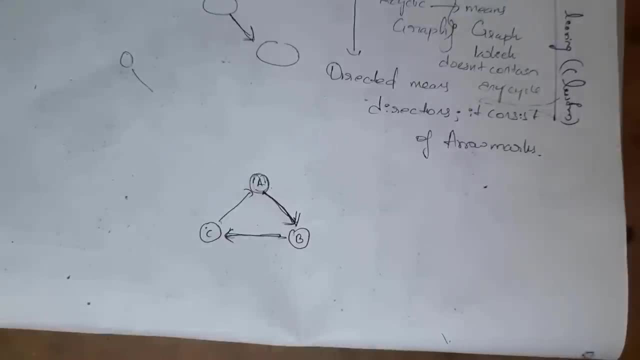 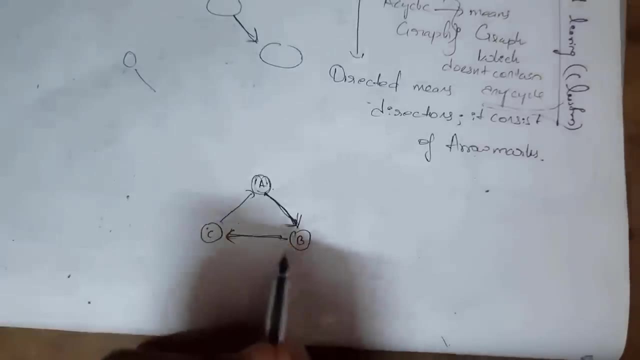 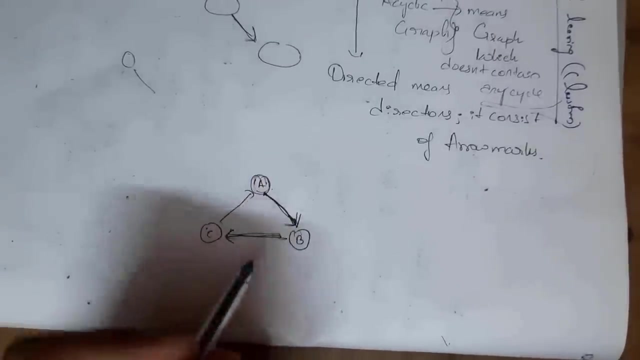 not contains any cycle. For example, this is cyclic graph: Total. there are three nodes, that is, node A, node B and node C. Node A is directed to node B and node B is directed to node C and node C is directed to node A And again node A is directed to node B. That mean graph is repeating again and 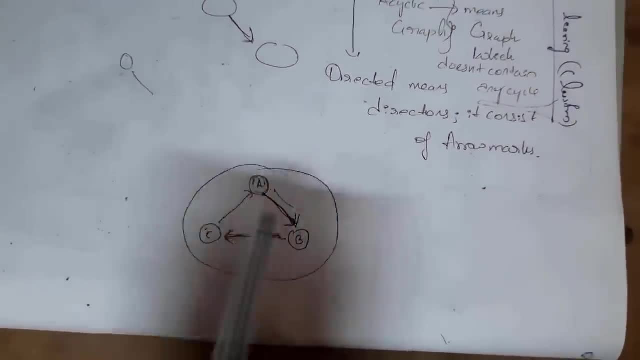 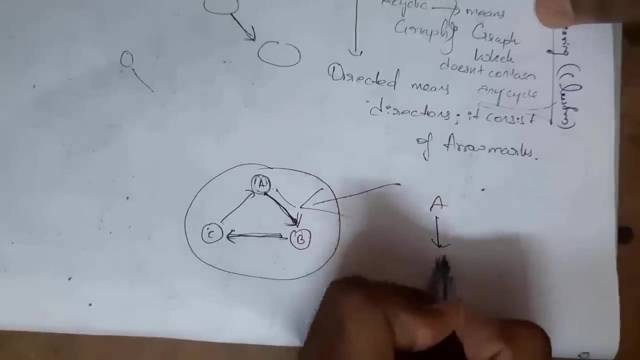 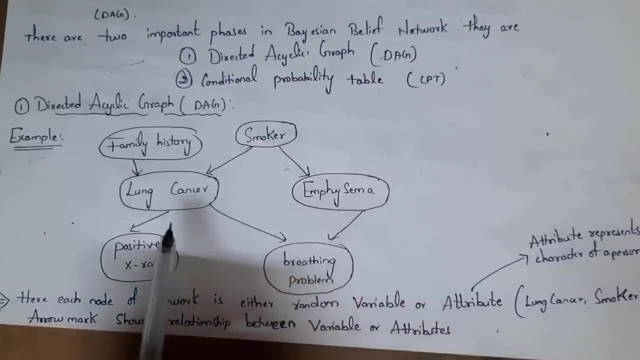 again, There is no end for this, So it is known as cyclic graph. But acyclic mean graph which do not form any cycle. For example, node A is passing to node B and node B is passing to node C. In this there is no cycle, So it is known as acyclic graph. This is directed acyclic graph. 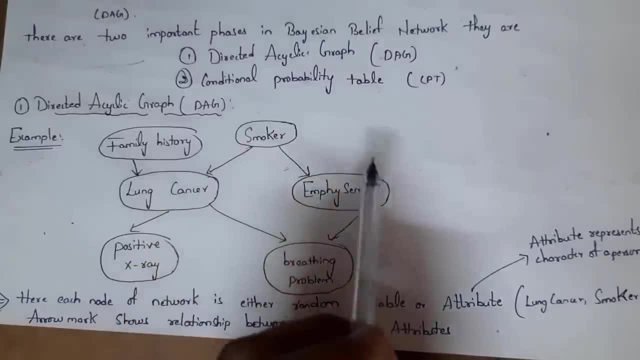 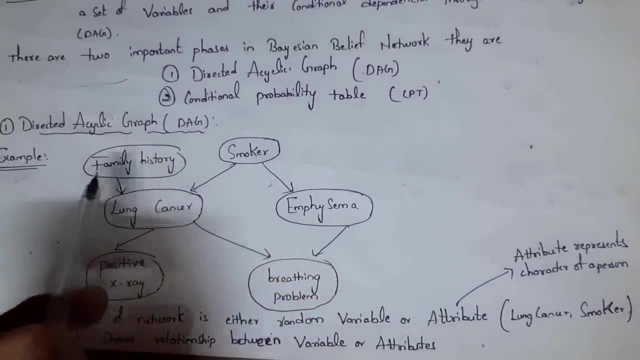 because this graph do not contains any cycle and it is directed Now. I am taking an example of lung cancer Total. there are two possibilities of getting lung cancer. They are: first, one is family history and next one is smoker And person- those who smoke. they can also get. 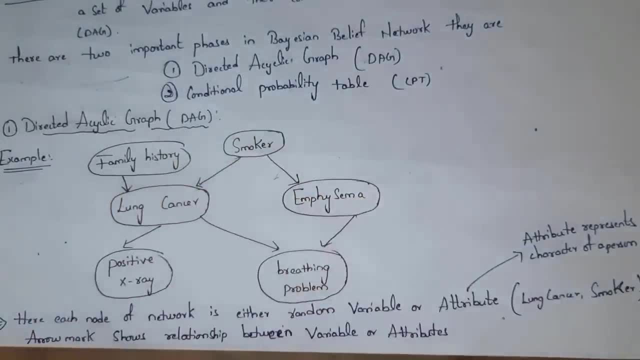 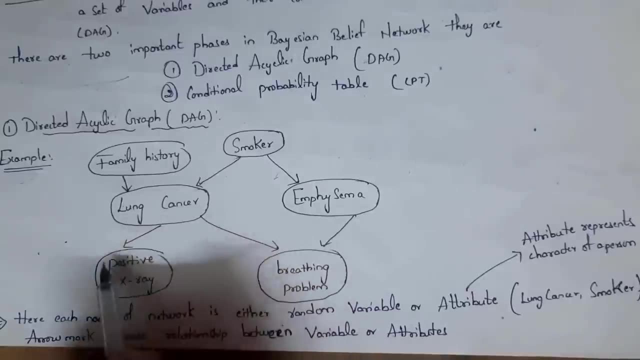 another disease like emphysema. Emphysema is also one of the disease Person: those who get lung cancer. they will get positive x-ray and they will get breathing problem. So I am connecting this lung cancer to positive x-ray and breathing problem. And person: those who suffer from. 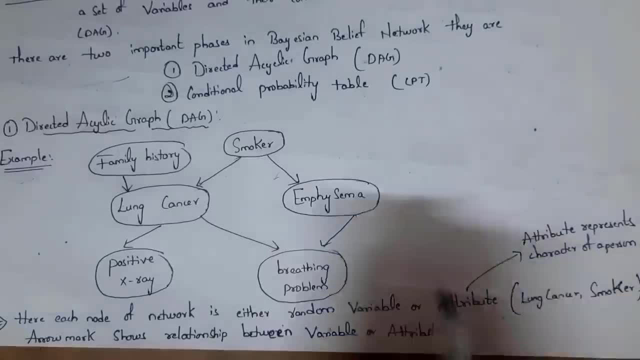 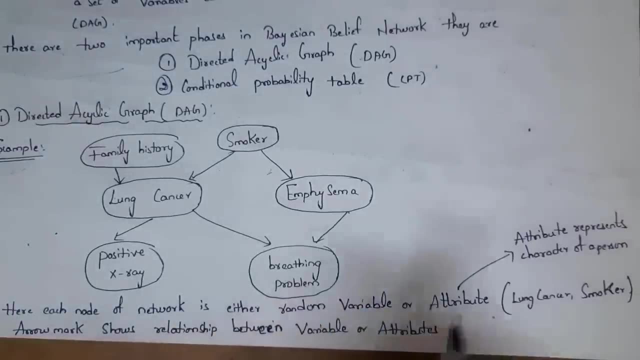 emphysema, they will not get positive x-ray, but they will get breathing problem. So I am connecting emphysema to breathing problem Here. each node of network is either random, variable or attribute. That means whatever the data that is present inside this node. we call this data as variable. 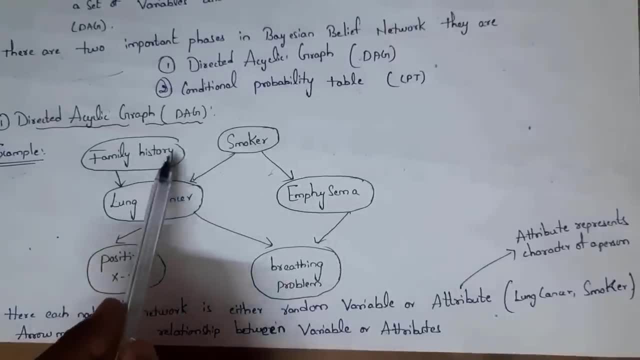 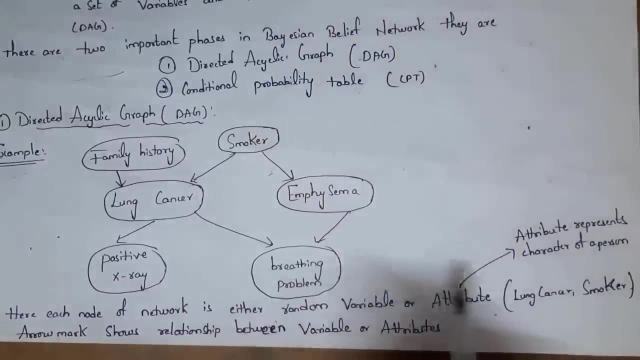 For example, here lung cancer is variable. Here family history is variable. Smoker is variable. We can also call this smoker as attribute. Attribute means character. Attribute represents character of a person. Smoker is character, So we can also call this variable as attribute. 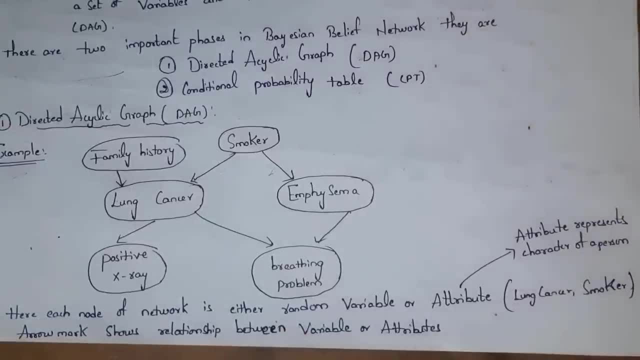 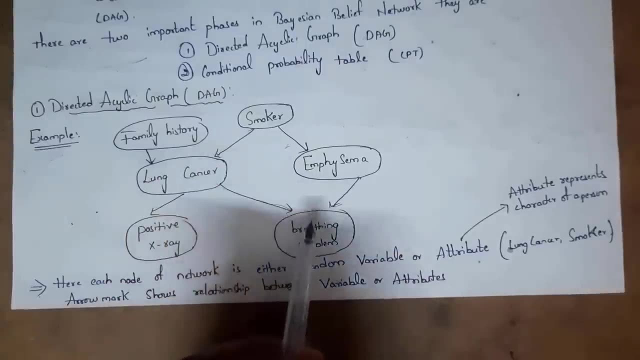 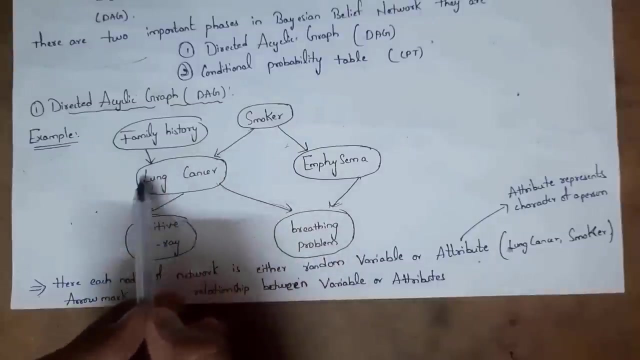 And arrow mark shows relationship between variables. For example, if you consider this variable, that is breathing problem, person with lung cancer will get breathing problem and person with emphysema disease also will get breathing problem. So parents of this breathing problem are: first one is lung cancer and next one. 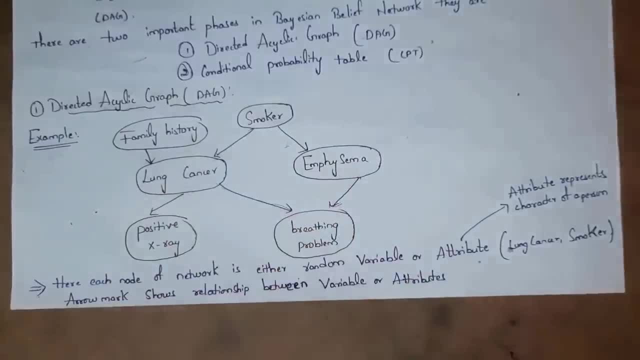 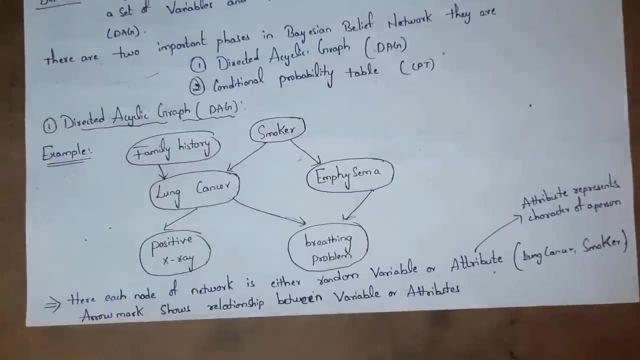 is emphysema. These both are parents to this breathing problem. For example, if you consider variable that is lung cancer, lung cancer depends on family history and smoker. So parent variable of this lung cancer are family history and smoker. these both are parents to this lung cancer, called dependent variables as parent. 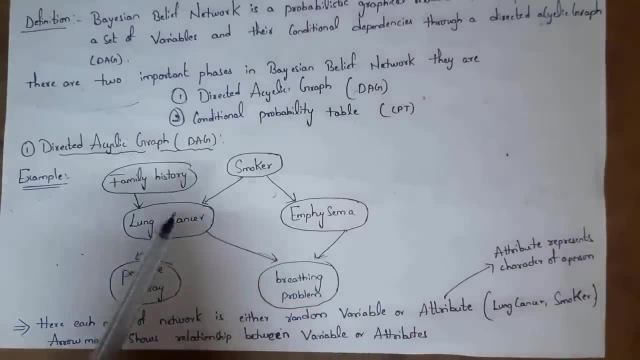 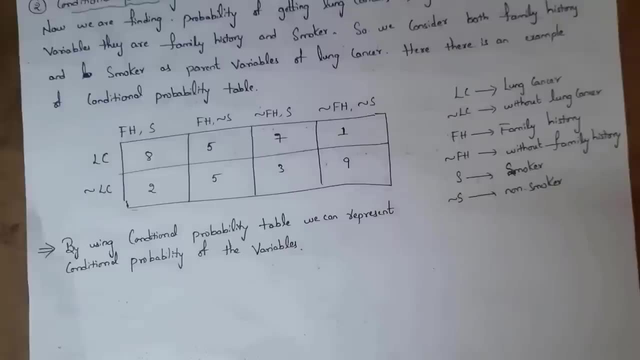 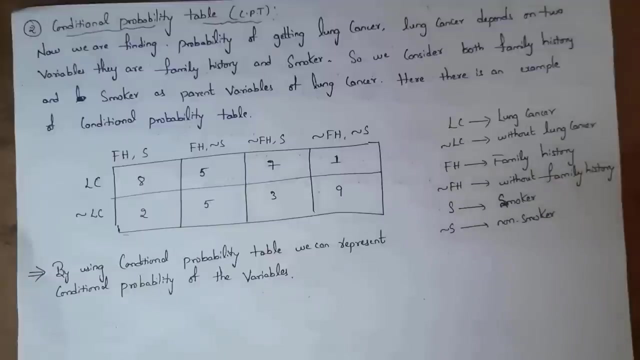 variables. now i want to find probability of getting lung cancer. we can find probability of particular variable by using conditional probability table. this is conditional probability table of lung cancer, where lc represent lung cancer and negation lc represent not getting lung cancer. and lung cancer depends on two variables. they are family history and smoker. 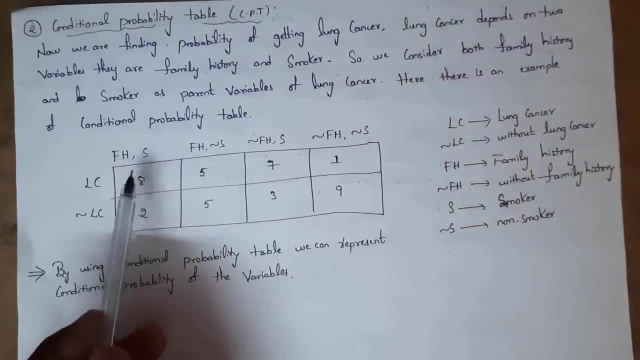 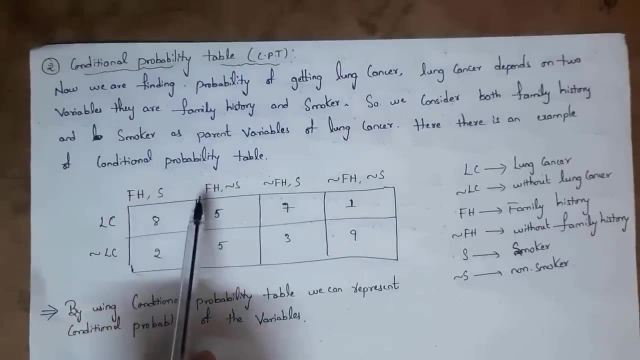 so we consider both family history and smoker as parent variables. so we need to take only parent variables. so what are possibilities here? first one is family history and smoker. next one is family history and non-smoker, and third one is no family history and smoker and last one is no family. 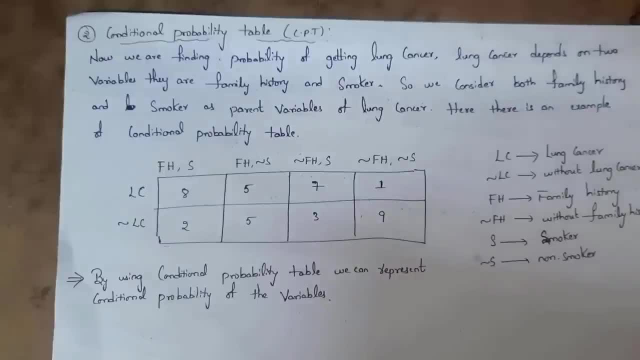 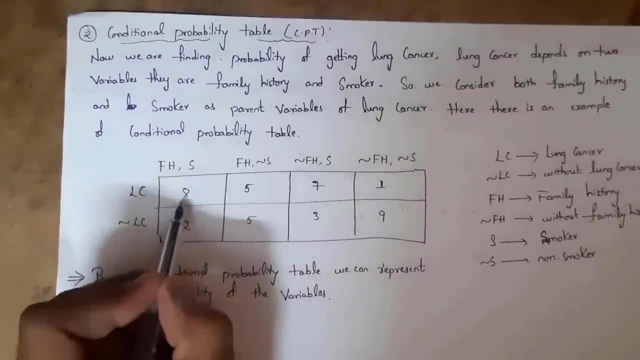 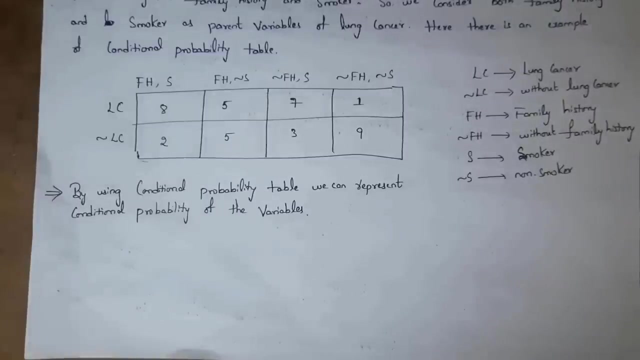 history and non-smoker. these are four possibilities. for example, if a person is having both family history and smoking habit, then out of 10% there is 8% of chance to get lung cancer and remaining 2% percent chance of not getting lung cancer. If a person is having family history but he don't have 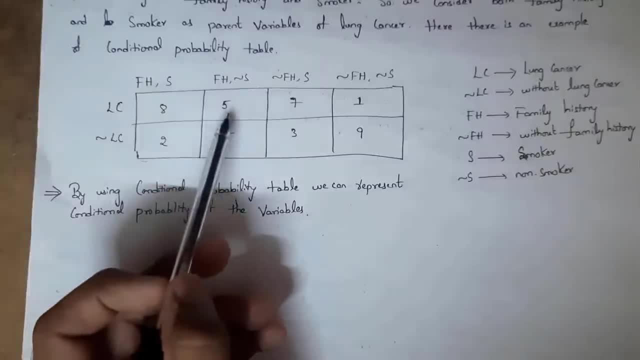 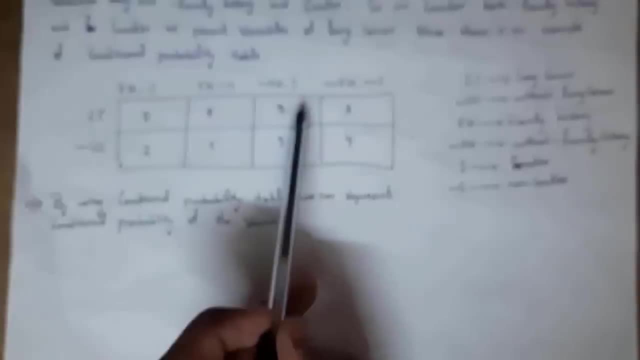 smoking habit, then out of 10 percent he has five percent chance to get lung cancer and remaining five percent chance of not getting lung cancer. Person don't have family history but he has habit of smoking, then out of 10 percent he has seven percent chance to get lung cancer and remaining. 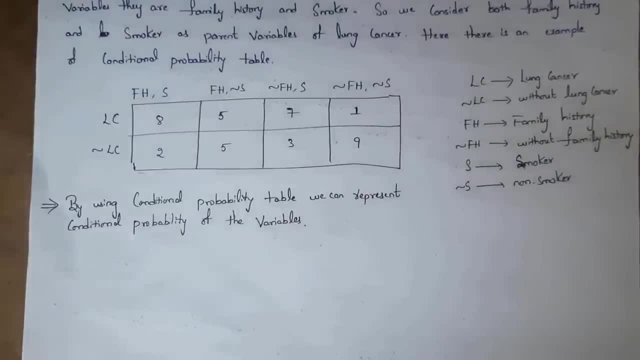 three percent chance of not getting lung cancer Person don't have family history and as well as smoking habit, then out of 10 percent he has only one percent chance to get lung cancer and remaining nine percent chance of not getting lung cancer. This is conditional probability table By using 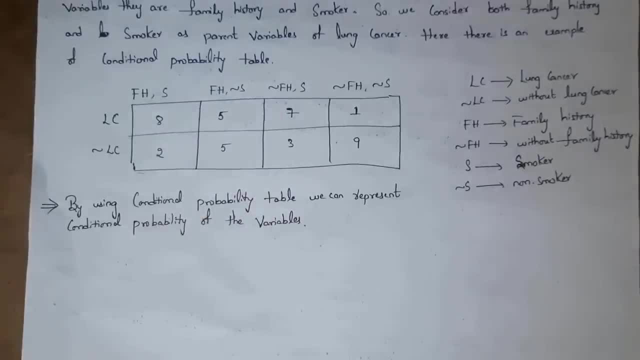 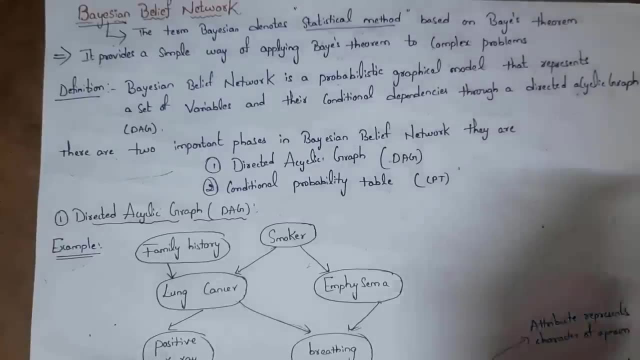 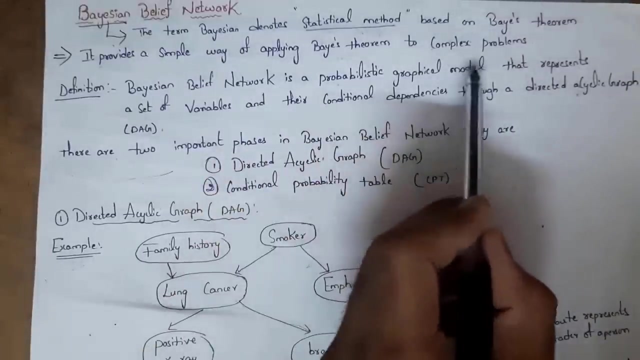 this conditional probability table we can represent conditional probability of variable. Now I will explain. definition of Bayesian belief network. Bayesian belief network is a probabilistic graphical model that represents set of variables and their conditional dependencies. Throw a directed acyclic graph. Bayesian belief network is a probabilistic graphical model. 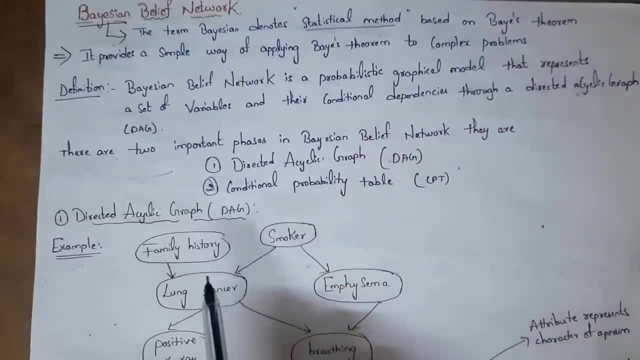 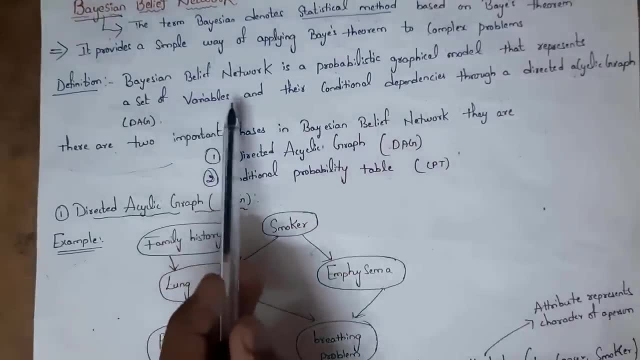 That mean graphical model mean we use graph that is directed acyclic graph and it is used to find probability. So it is probabilistic graphical model that represents a set of variables and their conditional dependencies through a directed acyclic graph. That mean by using directed acyclic 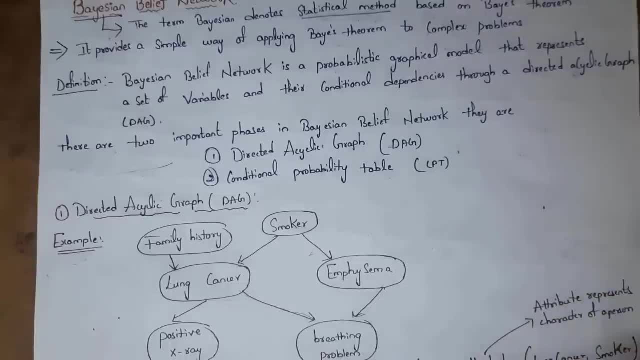 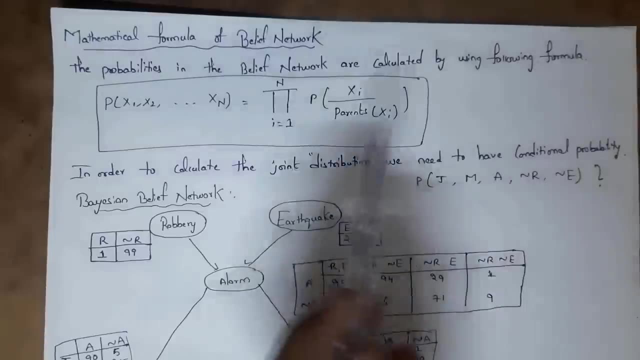 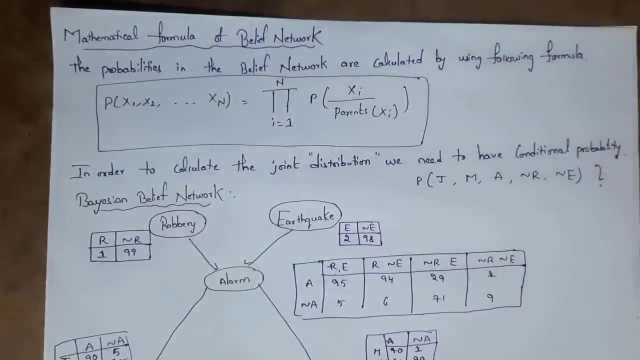 graph. this Bayesian belief network will show relationship between variables. That is, how one variable is depend on another variable, based on the condition. I already explained this in this example. This is mathematical formula of Bayesian belief network. In order to find probability in Bayesian belief network, we use this formula. Meaning of this formula is probability of. 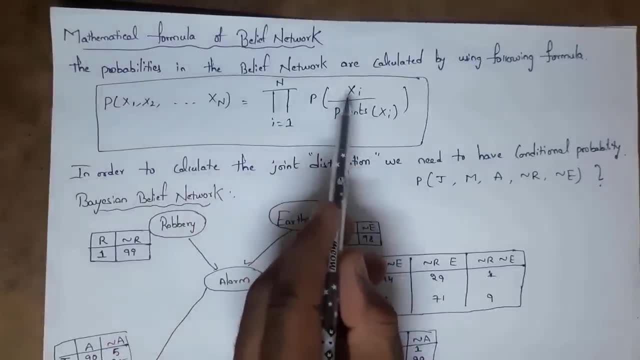 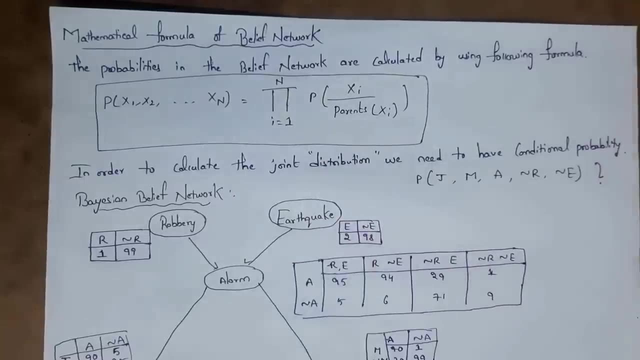 attribute is equal to probability of that particular attribute by its parent attribute. This is meaning of this formula. We use this formula in order to calculate joint distribution. I will explain joint distribution problem with an example. This is Bayesian belief network, As we know. 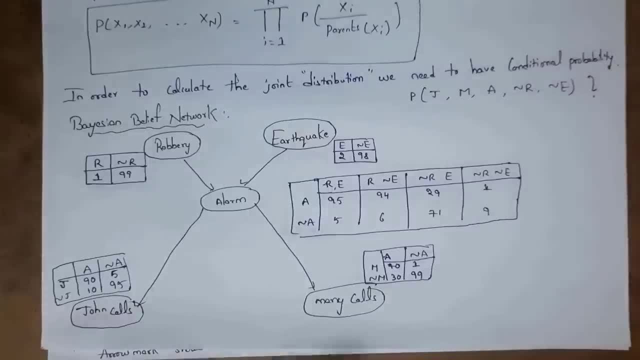 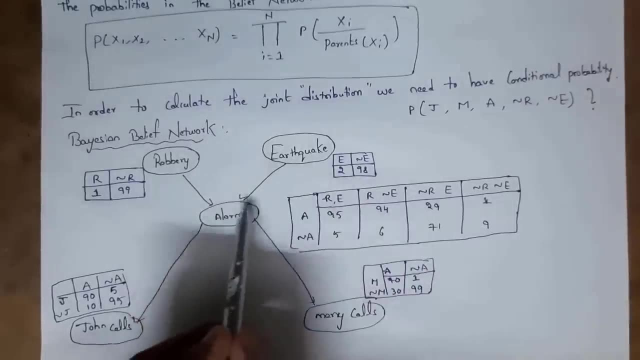 Bayesian belief network contains directed acyclic graph and conditional probability table. This is directed acyclic graph. Meaning of this graph is: whenever robbery or earthquake occurs, this alarm will ring. When alarm rings, John and Mary calls to police. This is meaning of this graph. 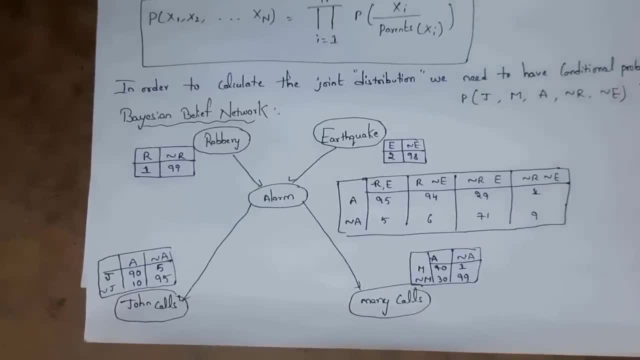 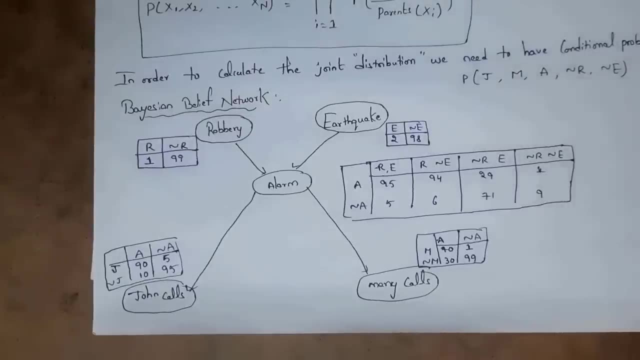 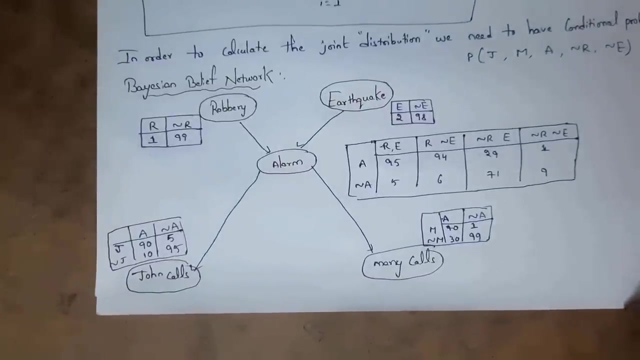 Now we need to write conditional probability table for each and every variable. This conditional probability table will provide information about how much chance is there that particular event will occur or will not occur. It will provide information about that. If we consider this variable, that is robbery, How much chance is there that robbery will occur and robbery will not? 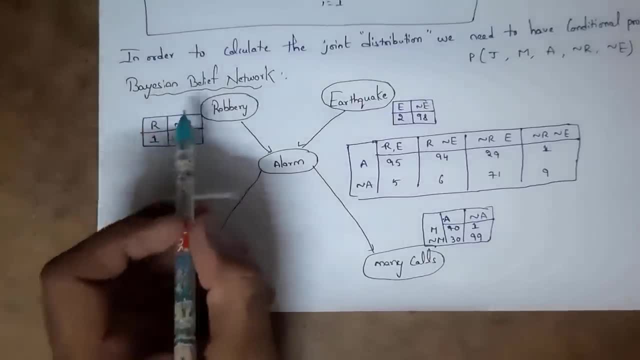 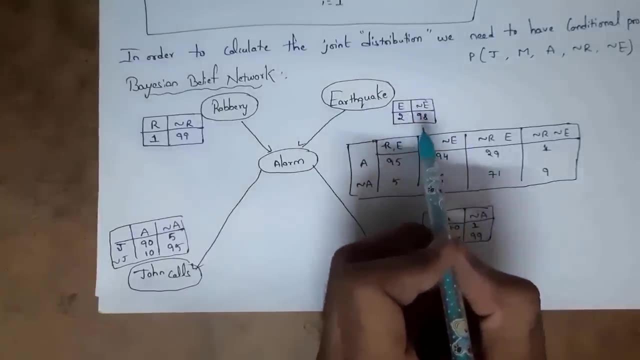 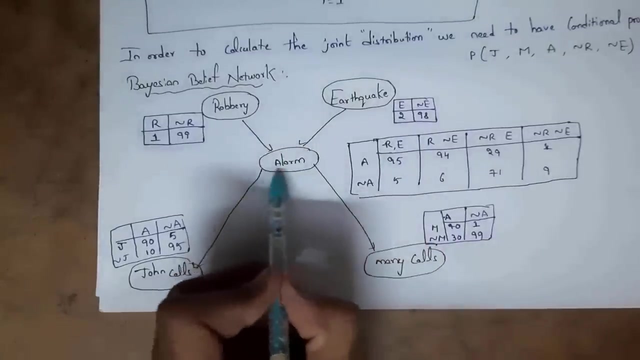 occur. There is one percent chance that robbery will occur and there is 99 percent chance that robbery will not occur. And similarly, earthquake: There is two percent chance that earthquake will occur and remaining ninety percent chance that earthquake will not occur. Next, we need to write probability table for this alarm. We need to write conditional. 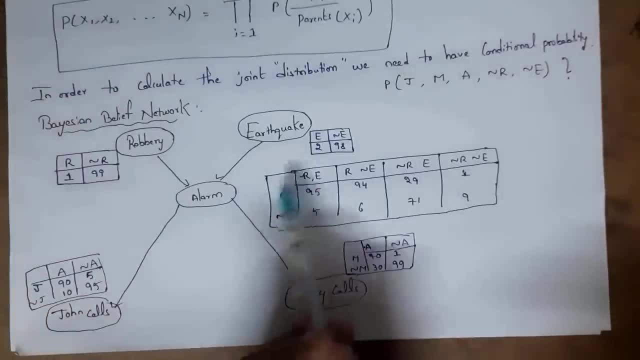 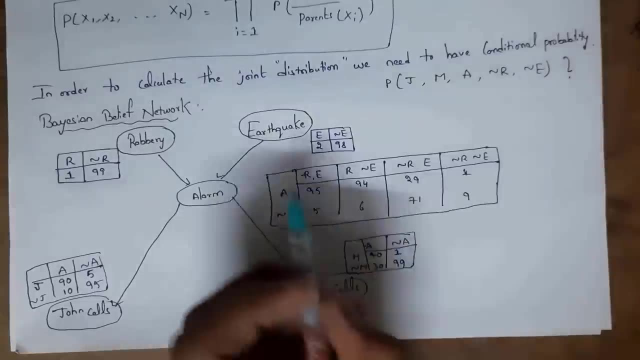 probability table based on the variable and its parent variables. What are parent variables for this alarm? robbery and earthquake. These two are parents. There are two chances for alarm, That is, alarm will ring and alarm will not ring, And there are four chances. that is, robbery and earthquake. 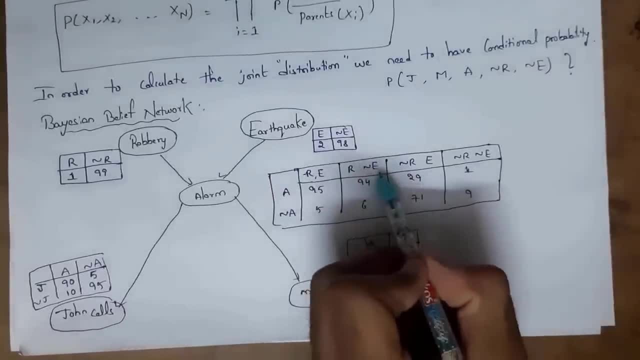 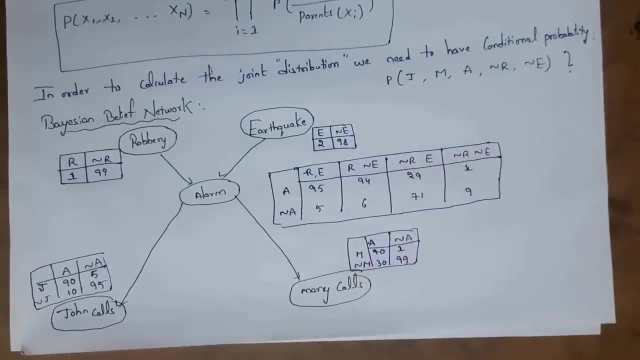 Robbery will occur and earthquake will occur. Robbery will occur, but earthquake will not occur. And robbery will not occur, but earthquake will occur. And robbery and earthquake will not occur. These are the four chances. When robbery and as well as earthquake occurs, then there is 95 percent. 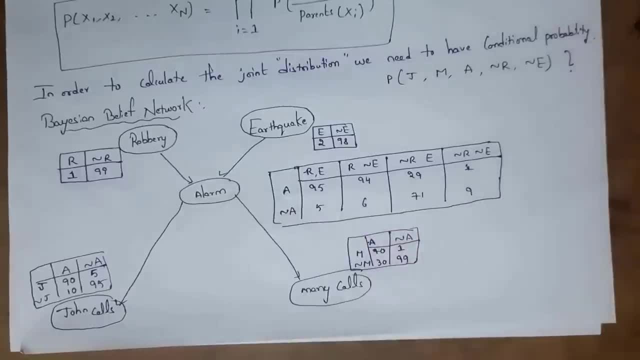 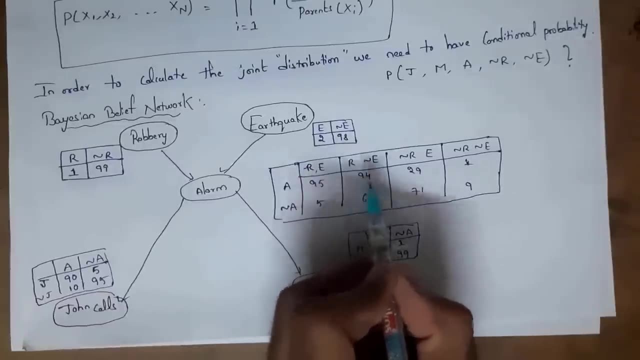 chance that alarm will ring And rest of the five percent chance that alarm will not ring. Similarly, robbery will occur, but earthquake will not occur. In this case, there is 94 percent chance that alarm will ring and there is six percent chance that alarm will not ring. And when robbery? 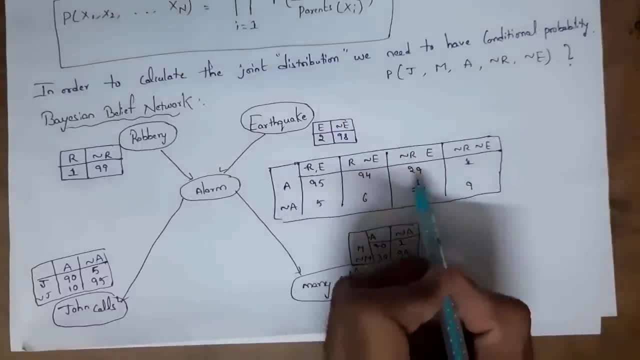 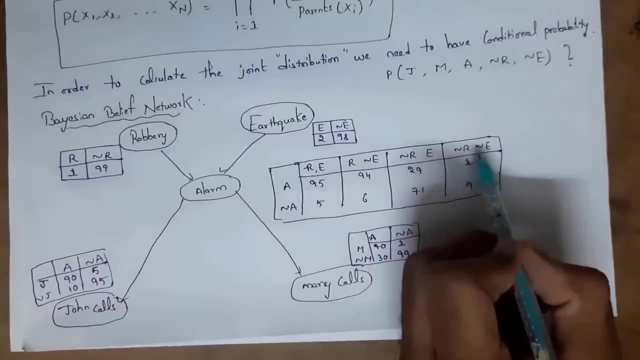 will not occur, but earthquake will occur. In this situation, there is 29 percent chance that alarm will ring and seventy five, seventy one percent chance that alarm will not ring. And when robbery will not occur and earthquake will not occur, In that situation there is one percent chance that 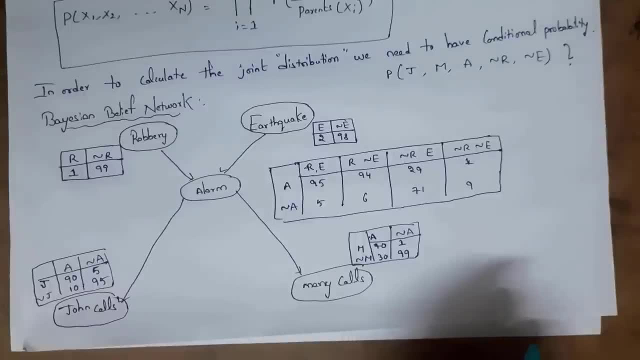 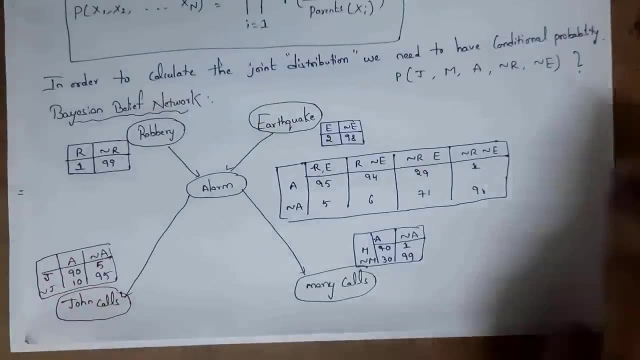 alarm will ring because there is no robbery and no earthquake. So in that situation there is only one percent chance that alarm will ring. Ninety one percent chance that alarm will not ring. This is the conditional probability table for alarm Guys. you should remember one important thing, that is: 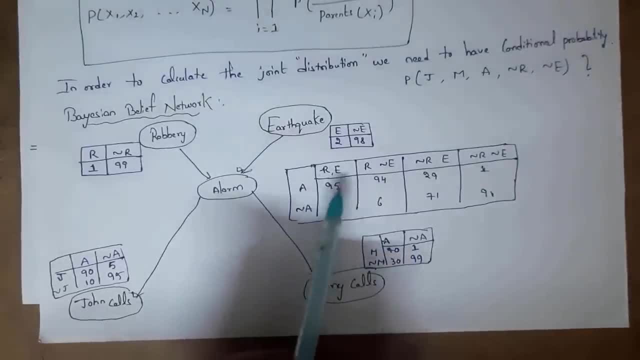 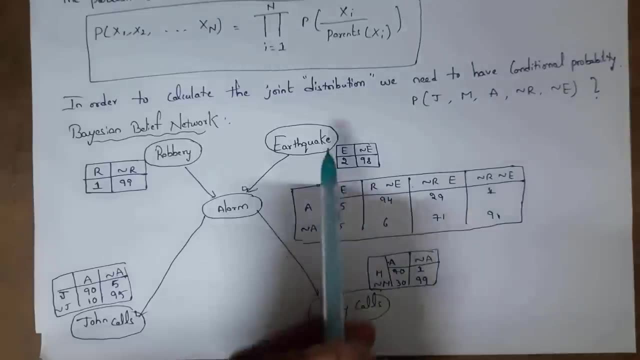 you need to write probability of particular variable by comparing it with parent variable. Here parent of alarm are robbery and earthquake. So in this table I took robbery and earthquake. Robbery and earthquake do not have any parent variable, So I directly written table. Now I 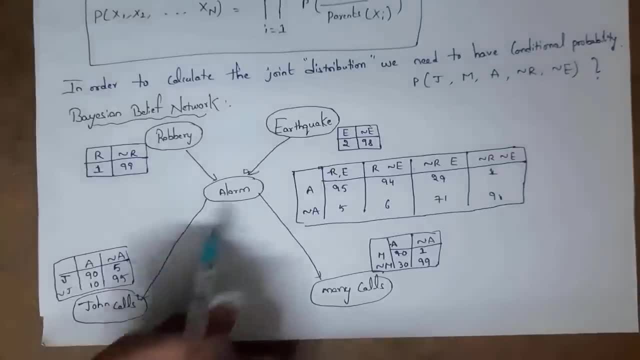 am writing. conditional probability for John Calls. Parent of John Calls is alarm, So here I took alarm. Varyage stands for alarm. Whenever alarm rings, there is 90 percent chance that John will call to police And there is 10 percent chance that John will not call. 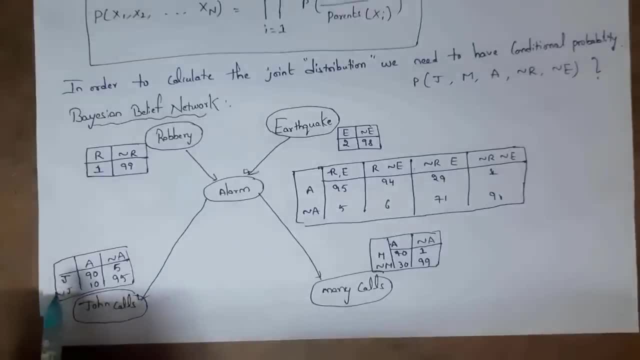 And whenever alarm do not ring, there is five percent chance that John will call to police and the rest 95 percent chance that John will not call to police. Next, I written conditional probability table for Mary calls Parent of Mary is alarm, So I written alarm. here Varies stands: 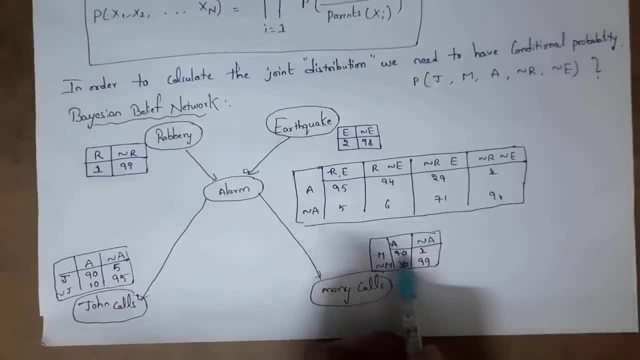 for alarm. Whenever alarm rings, there is 70 percent chance that Mary will call to police and rest of the thirty percent chance that Mary will not call to the police. And whenever alarm not ring, In that situation there is 1% chance that Mary will call to police and 99% chance. 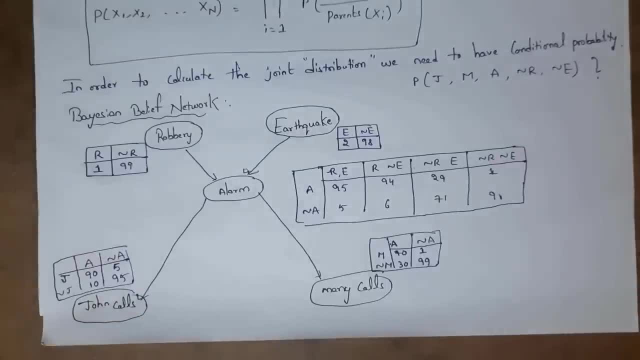 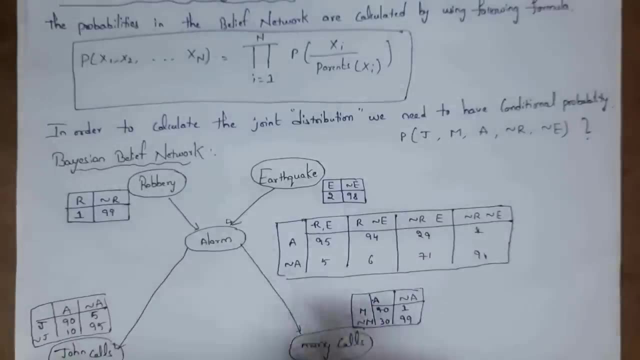 that Mary will not call to police. This is conditional probability tables for each and every variable. In order to calculate joint distribution, we need to have conditional probabilities. We already written conditional probabilities by using conditional probability table. Joint distribution is nothing, but we need to calculate probabilities for multiple events. 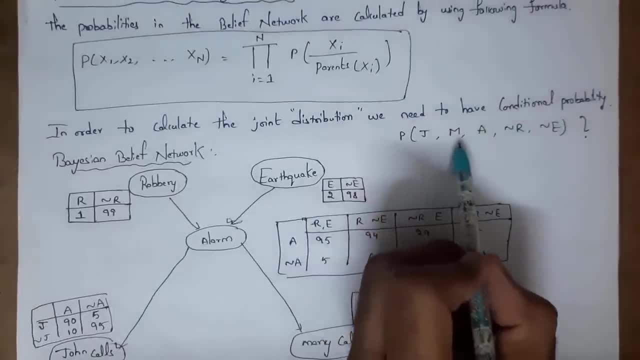 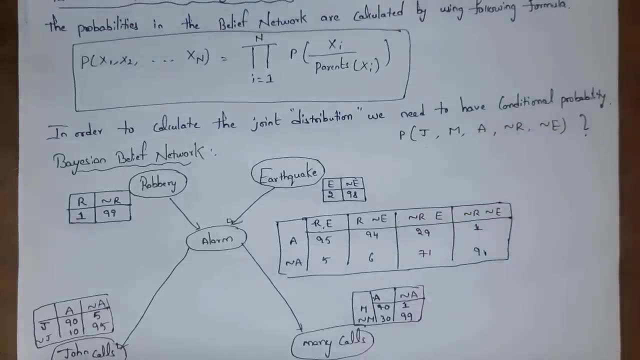 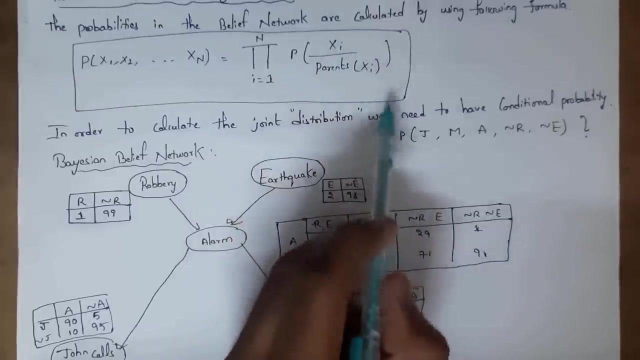 Here we need to calculate probability for John calls, Mary calls, alarm rings and robbery not occurred and earthquake not occurred. For this we need to calculate probability by using this formula. Formula is: probability of variable is equal to probability of that variable by its parent variable. Now I am calculating probability of John calls by using this formula, that is: 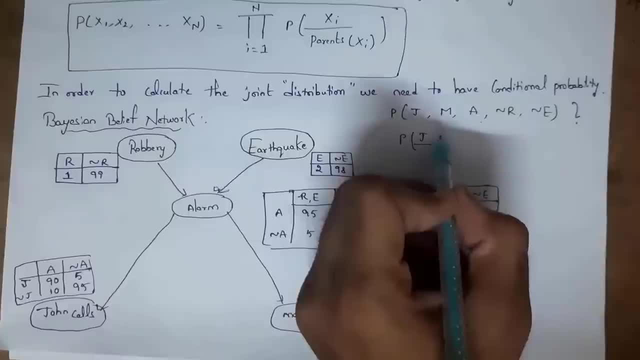 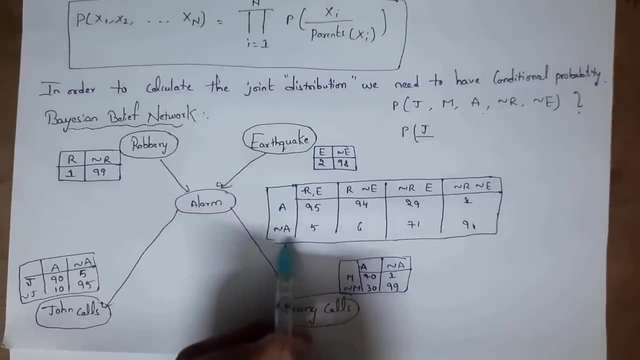 probability of John calls is equal to probability of John calls by its parent. Who is parent of John calls? that is alarm. But here, what should I write? Alarm rings or alarm do not rings. Which one I need to consider? I need to consider. 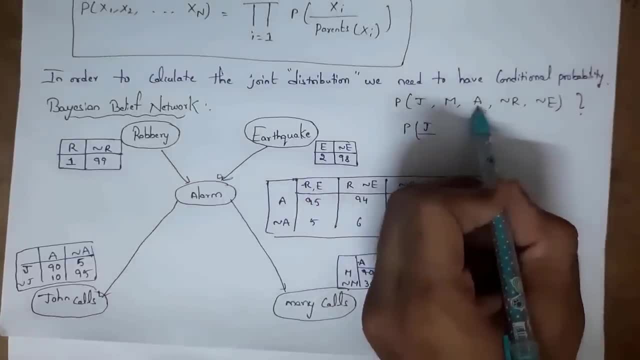 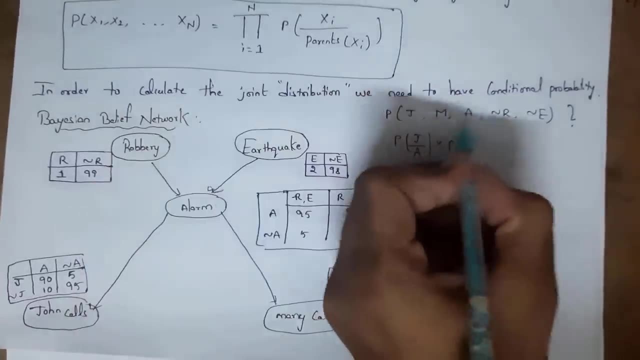 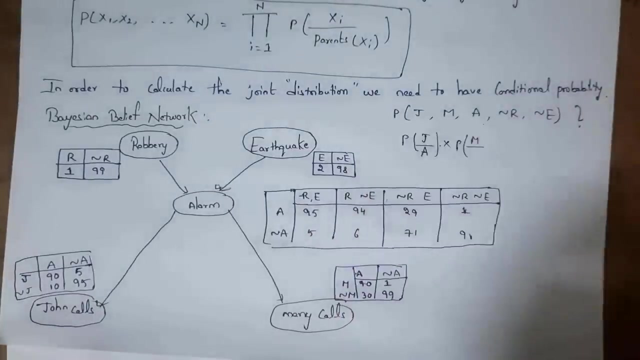 Alarm rings because in question the given alarm will ring. So here I need to consider alarm rings. that is, A into probability of Mary. Probability of Mary is equal to probability of Mary by its parent. Who is parent of Mary? Alarm: Here also we need to consider alarm rings, because in question. 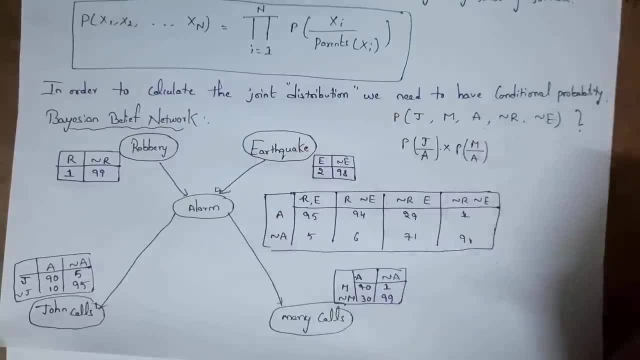 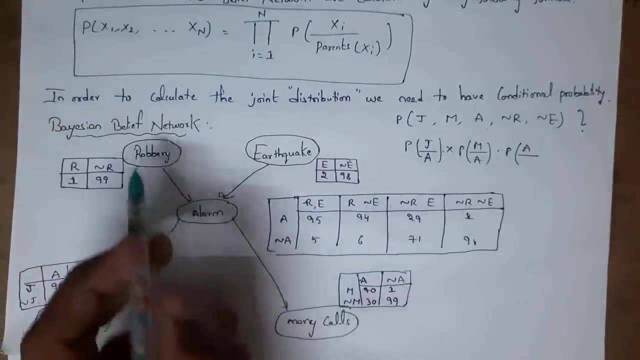 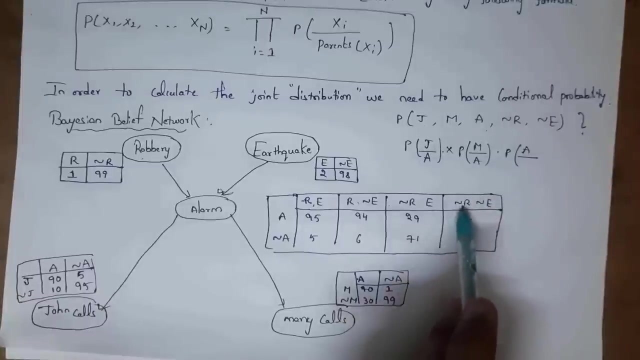 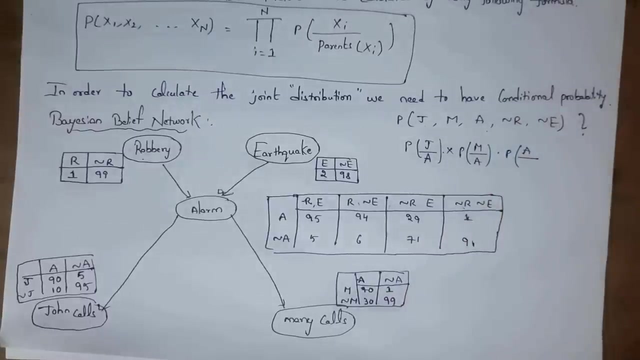 the given alarm will ring. So I written A here. that is alarm will ring. and probability of A. that is probability of A by its parent Who is parents of A. That is robbery and earthquake. But in out of this four, which one I need to consider? I need to consider: robbery will not occur and earthquake will not occur because in question they given that robbery will not occur and earthquake will not occur. 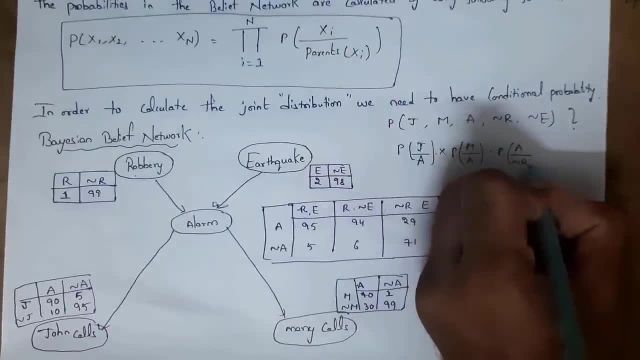 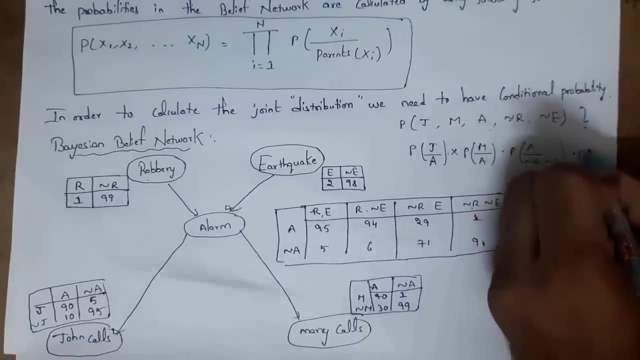 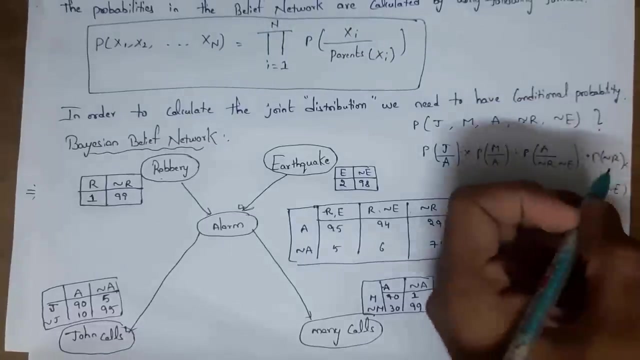 So I need to consider this, that is, robbery will not occur and earthquake will not occur And, at last, probability of robbery will not occur. That is directly. we need to write, because there is no parents for this robbery into probability of earthquake not occur, because there is no parents for earthquake also. 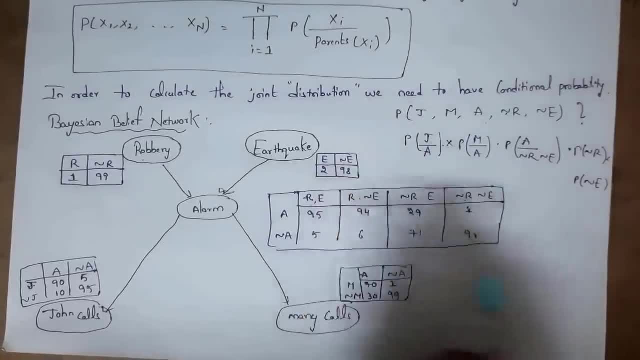 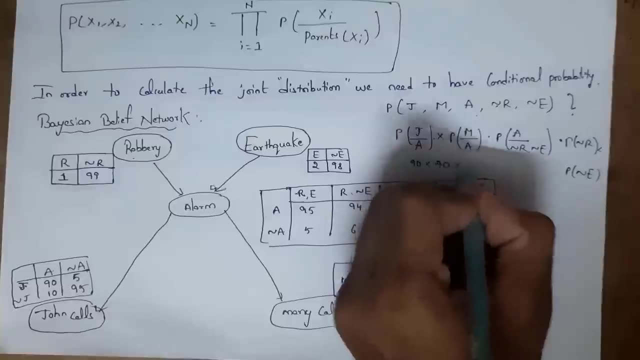 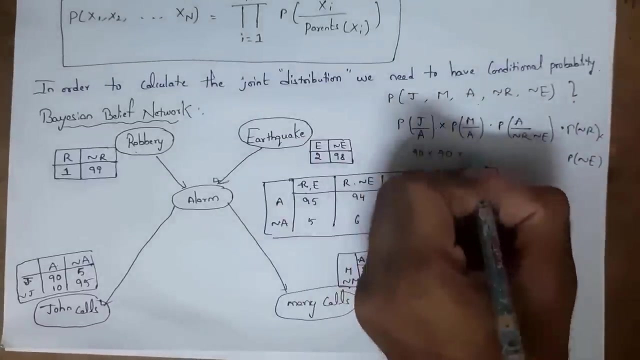 What is probability of John calls and alarm rings? That is, J is 90 into probability of M by A, that is, Mary calls and alarm rings, 70 into probability of alarm rings and robbery do not occur and earthquake not occur. Correct? But this probability is 1 into probability of robbery do not occur and that is 99 into probability of earthquake not occurred. 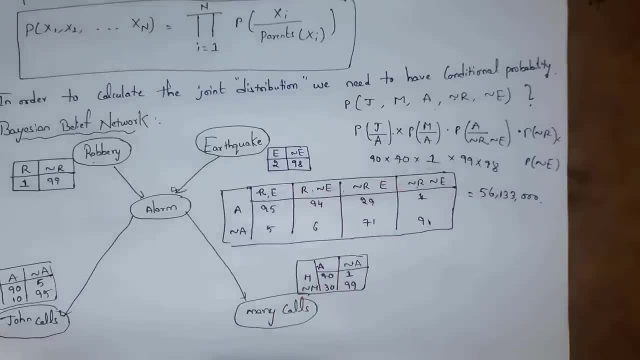 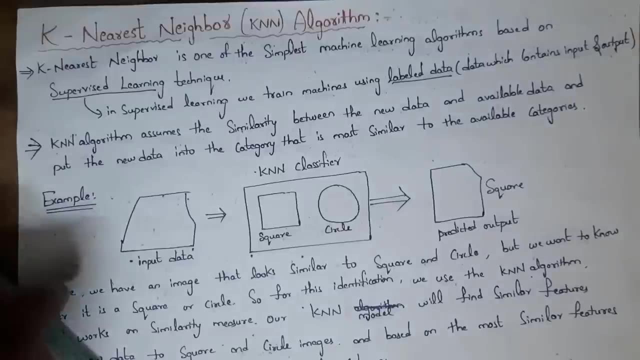 That is 98.. We need to multiply all this. after multiplying all these values, we will get result as 56 comma 133 comma 000.. This is final result. Next topic is K nearest neighbor algorithm. Shortly we call it as KNN algorithm. 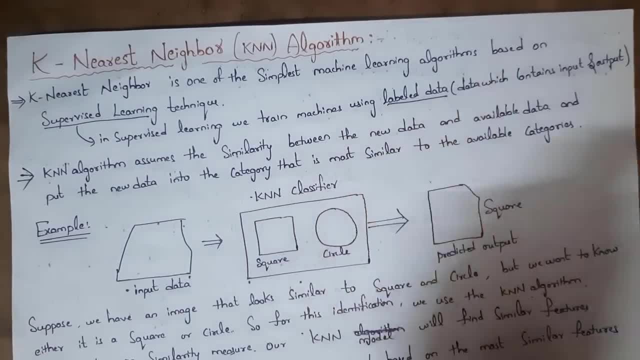 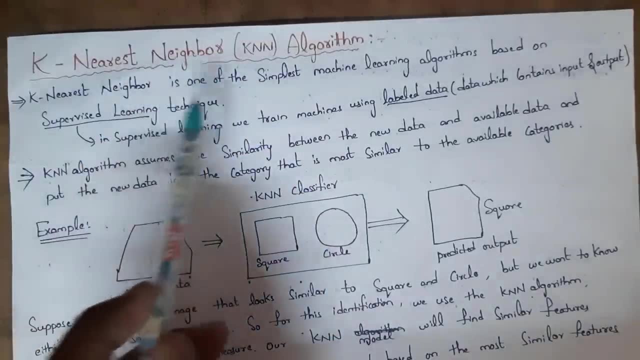 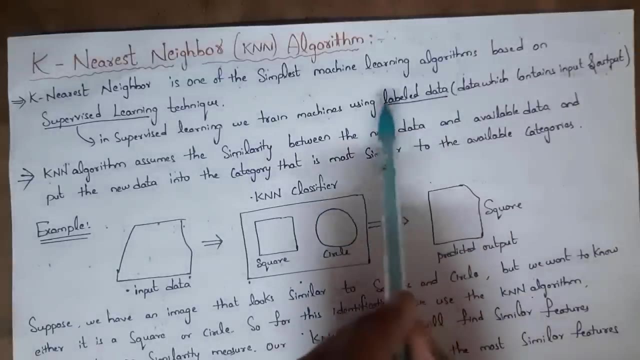 K nearest neighbor is one of the simplest machine learning algorithm based on supervisor learning technique. This KNN is machine learning algorithm And this KNN is based on supervisor learning technique. Supervisor learning technique mean: in supervisor learning technique, we train machines by using labeled data. labeled data mean data which contains input and output. 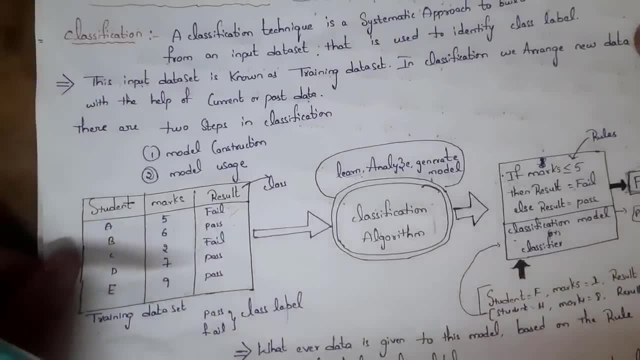 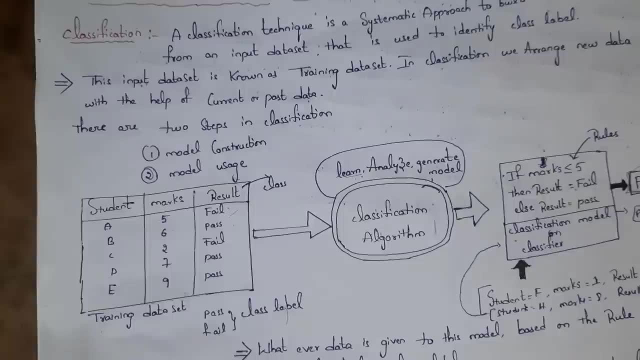 For example, if you consider classification in classification, we are training this classification algorithm by using labeled data. labeled data is nothing but data, which contains both input and output. For example, in this, student and marks are considered as input And whereas result Is considered as output. 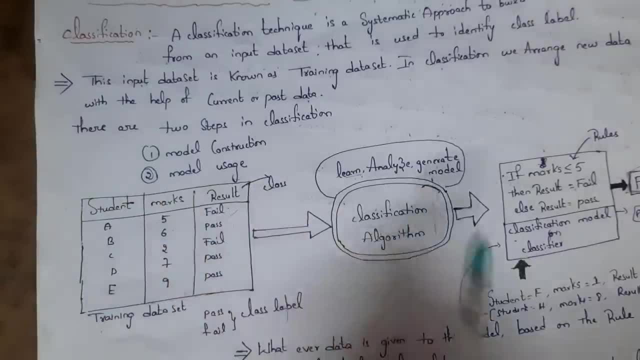 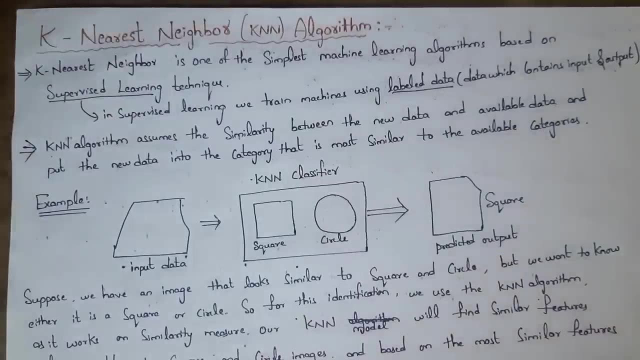 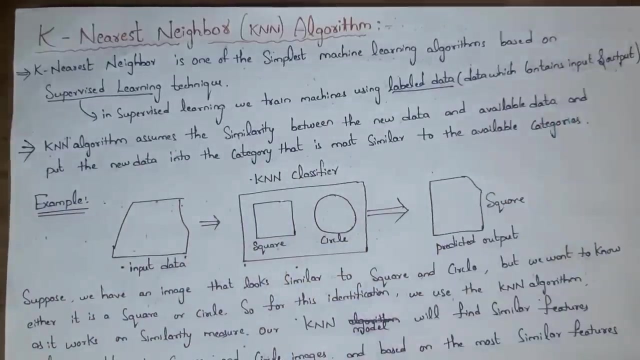 So this is labeled data. by using this labeled data we are training this algorithm. So classification is also a supervisor learning technique. So KNN is supervisor learning technique. that mean we train machines by using labeled data. KNN algorithm assumes a similarity between new data and available data and then put the new data into a category that is more similar to available category. 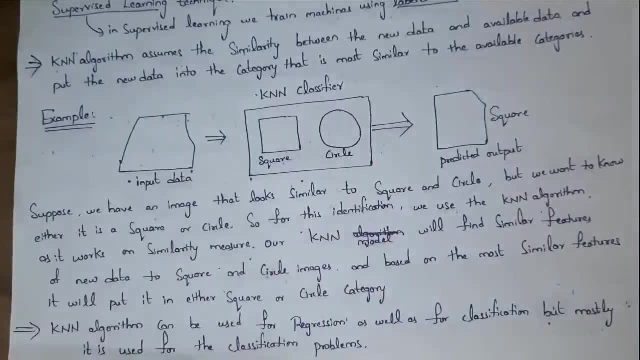 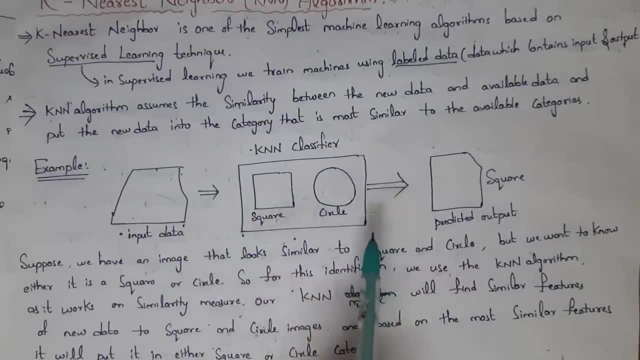 I will give one example so that you can clearly understand this definition. For example, I have one input data. Input data is Nothing, But it is new data. This is available data Total. there are two categories of data available with me. One is square category and another one is circle category. 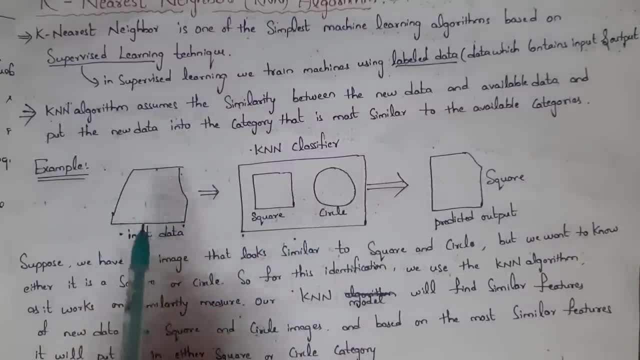 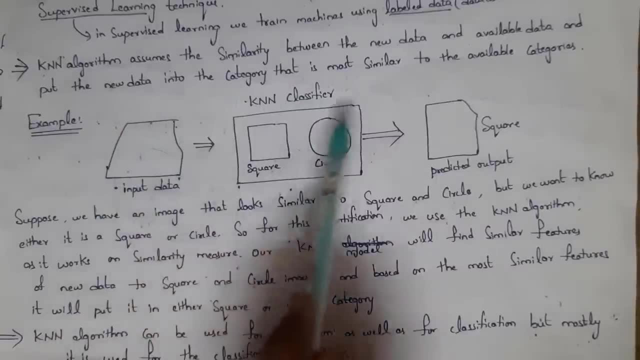 Now I want to place this input data, that is, new data, in any of these categories. How I will place? By using KNN classifier, we can place this input data in any of these available category, But how it will place? It will place based on the similarity. 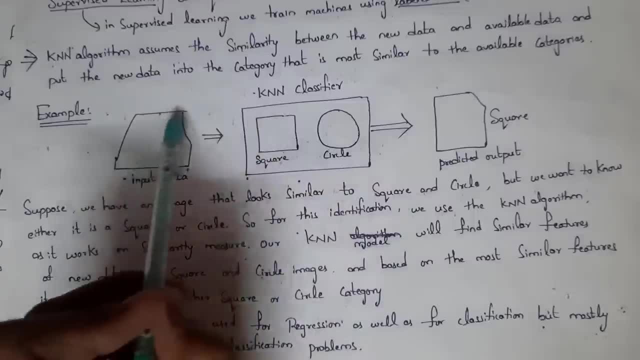 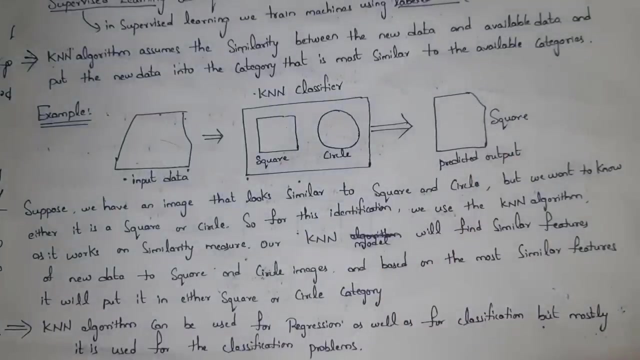 For example, this input data is similar to square because it is looking like square, So this input data is similar to square category. So KNN classifier will place this input data in square category. So output is: this data belongs to square category. I hope you have understood what is KNN algorithm. 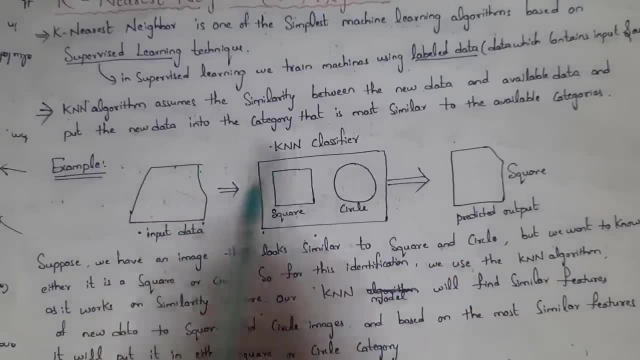 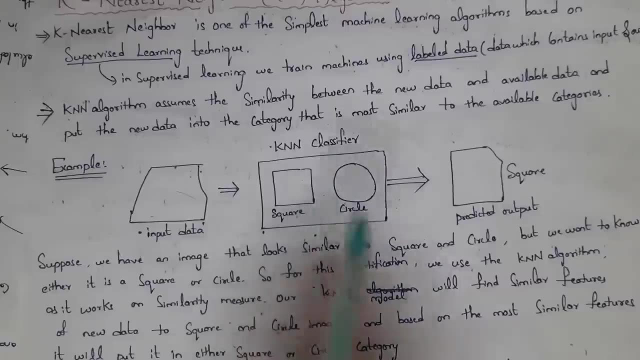 KNN algorithm assumes a similarity between new data and available data and then put the new data in the category which is similar to the available category. I hope you have understood this definition. For example, I have an image that looks similar to square And circle. 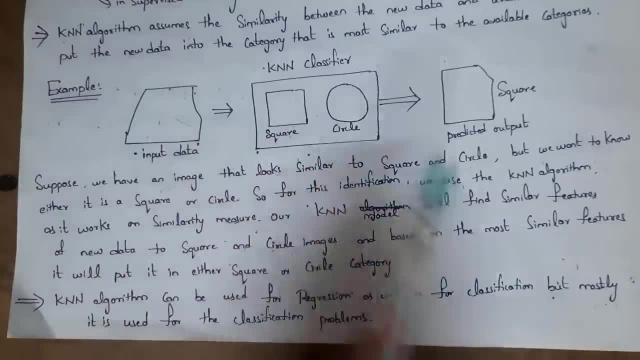 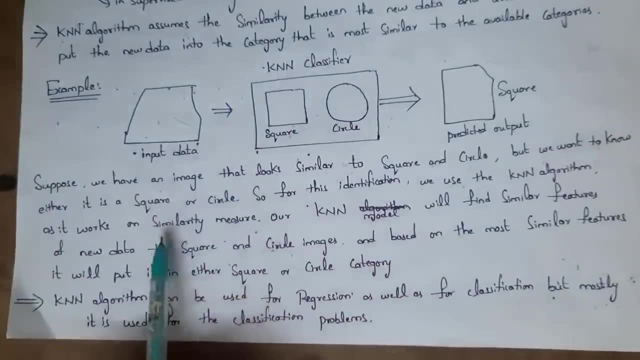 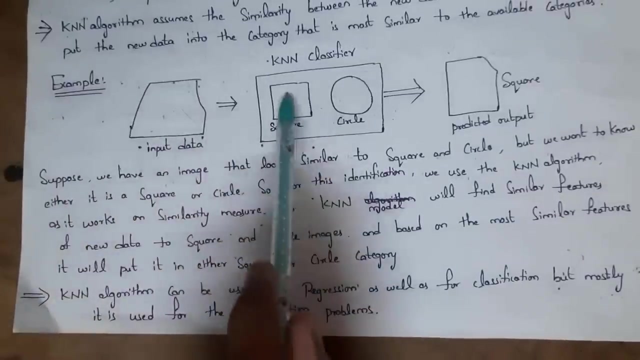 But I want to know either this image belongs to square or circle In order to identify that. I use KNN classifier And this KNN algorithm works based on the similarity measures, That is, KNN algorithm will find similar features between this new data with respect to square and circle. 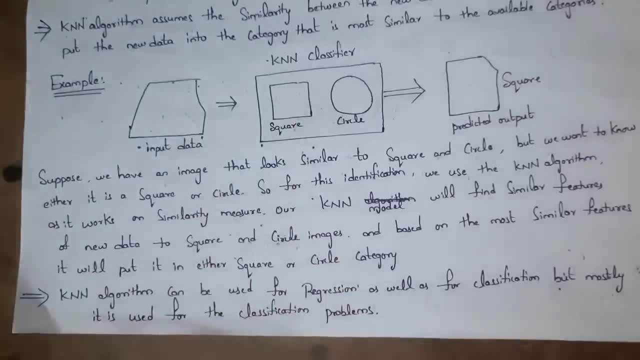 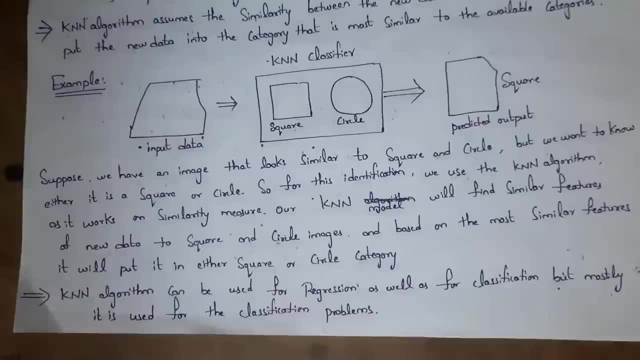 And based on the most similarity features, it will be placed. This new data will be placed either in square or circle, So this input data is much similar to square, So it is placed in square, And this KNN algorithm can be used for recreation and as well as for classification. 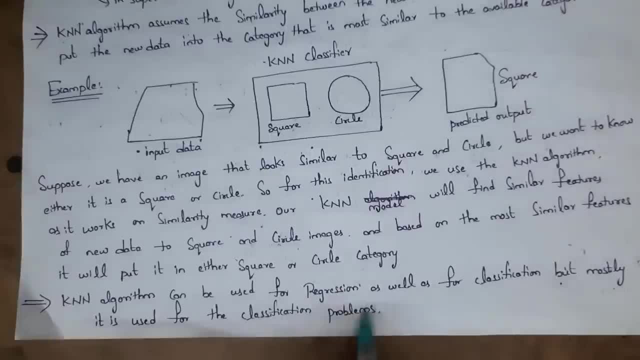 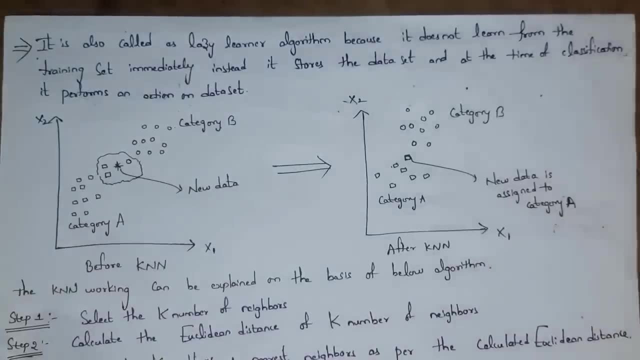 But mostly we use this KNN algorithm for classification, So we can also call this KNN algorithm as KNN classifier. We also call this KNN algorithm as lazy learner algorithm. The name itself says it is lazy in learning. We call this KNN algorithm as lazy learner algorithm because whatever the training data set that we give to this KNN algorithm, 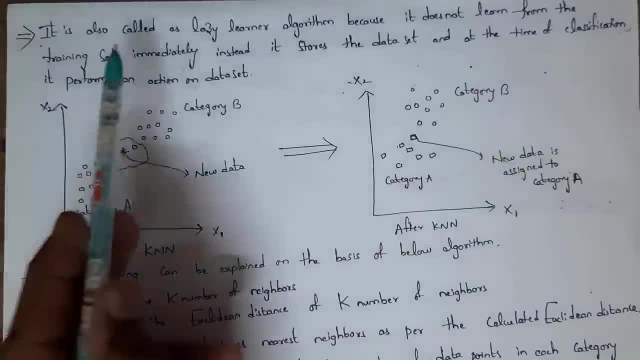 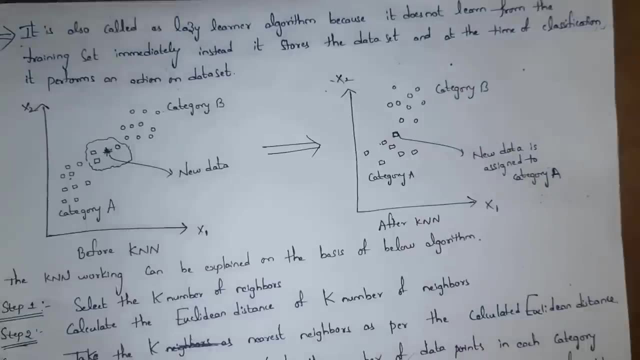 It will not learn that training data set. Instead, what it will do is it will store the training data set And then, at the time of classification, it performs some actions on that data set. This is an example of how KNN algorithm will work. 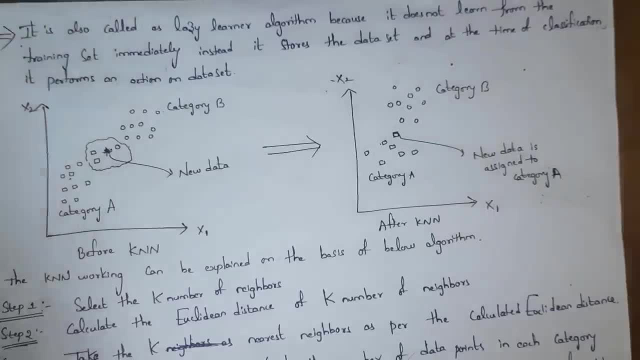 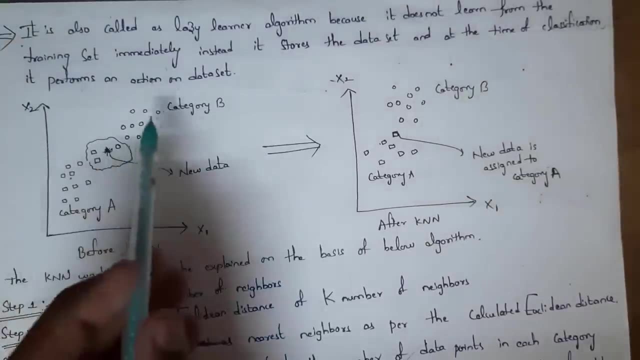 Total. there are two categories of data available with me. One is category A and another one is category B. Category A contains square data, That is, all the data is in square form, And whereas category B contains circular data, All the data is in circular form. 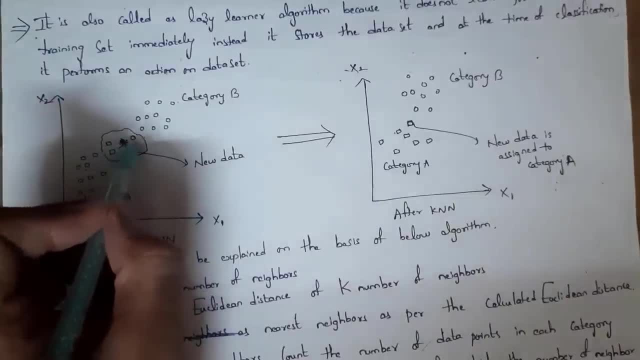 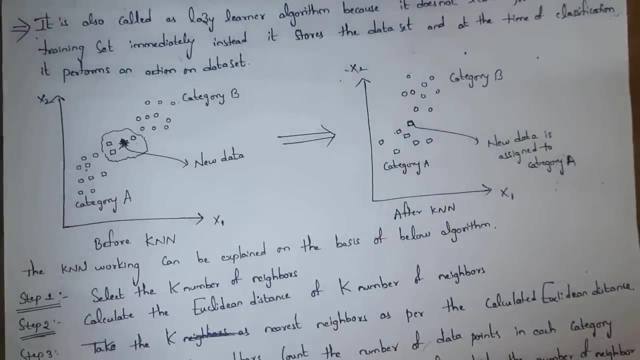 There is new data available with me. I want to place this new data either in category A or in category B by using KNN algorithm. What KNN algorithm will do is: at first, KNN algorithm will find some nearest neighbors. What are the objects near to this new data? 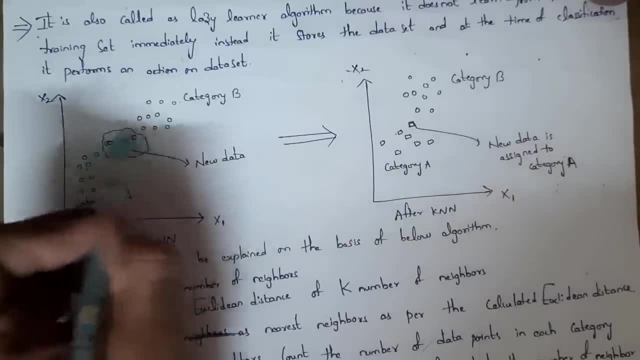 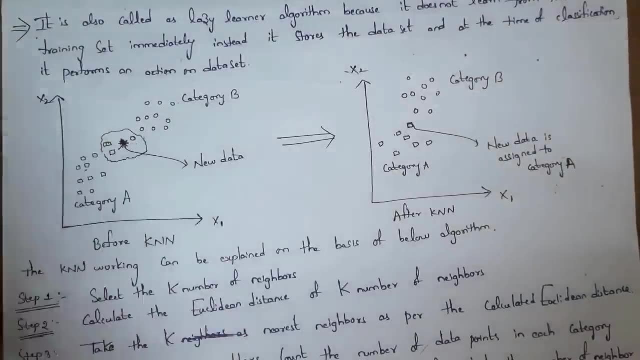 That is square, two squares and one circle- is near to this new data. Among these three nearest neighbors, two are square and one is circle, So majority is square because there are two squares and whereas only one circle. So we will place this new data based on majority. 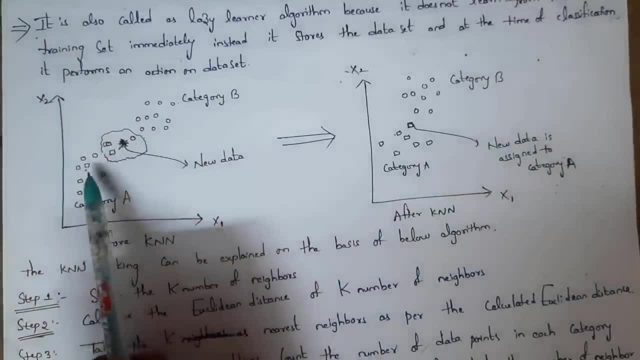 So majority is square now, so we will place this new data in this category A. We will place new data based on the nearest neighbors, So we call this as K- nearest neighbor algorithm. After placing this new object in this category A, this is how output looks like. 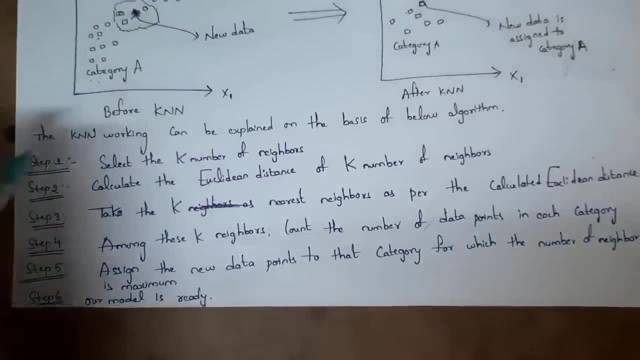 We placed this new object in category A. These are the steps, how KNN will work. This is KNN algorithm. At first I will explain KNN example. We will solve one problem and then we will go for algorithm so that you can easily remember. 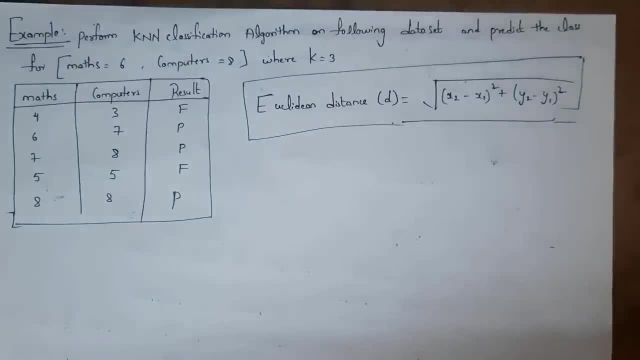 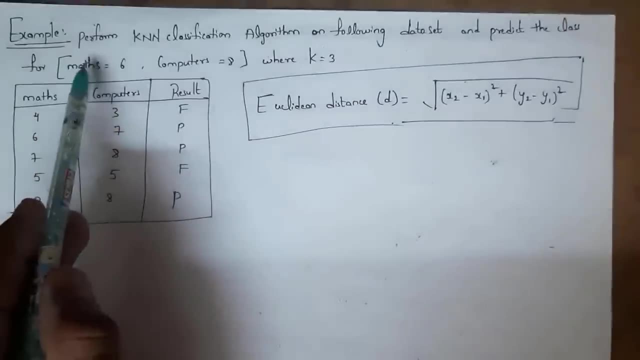 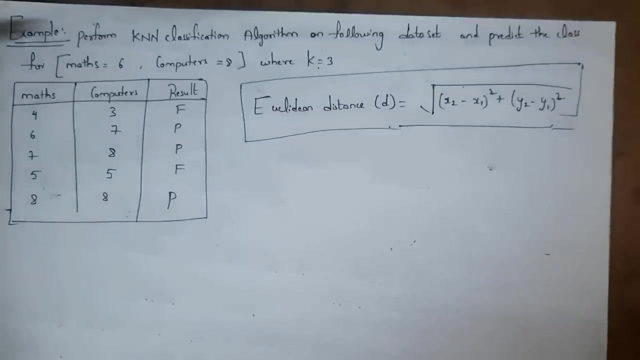 this algorithm. Here is an example which we need to solve: Perform KNN classification algorithm on following data set and predict. the class for mass is equal to 6 and computer is equal to 8, where k equal to 3.. Here given table contains three attributes: here marks of mathematics, marks of computers. 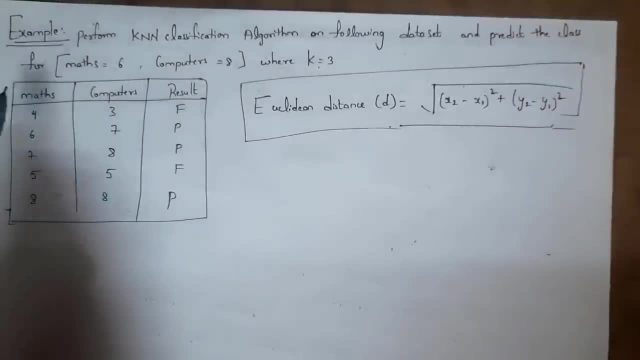 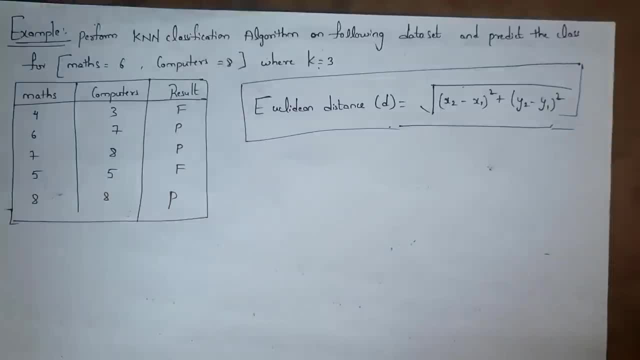 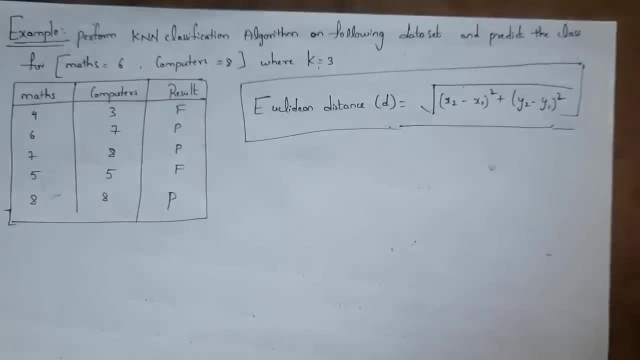 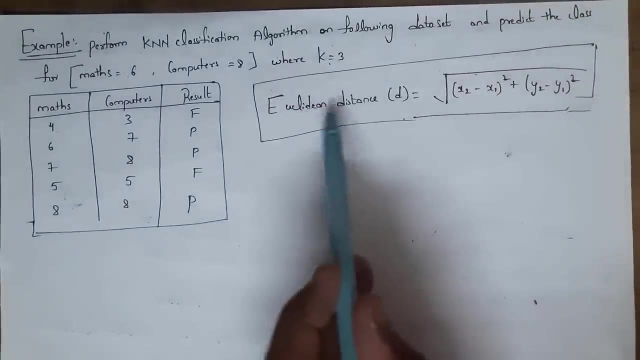 k equal to 3 means we need to consider 3 nearest neighbors in order to find results. In order to find nearest neighbors, we use this formula, that is, Euclidean distance. formula of Euclidean distance: isון ay, root of x- 2, minus x- 1 whole square plus y, y, 1 whole square. 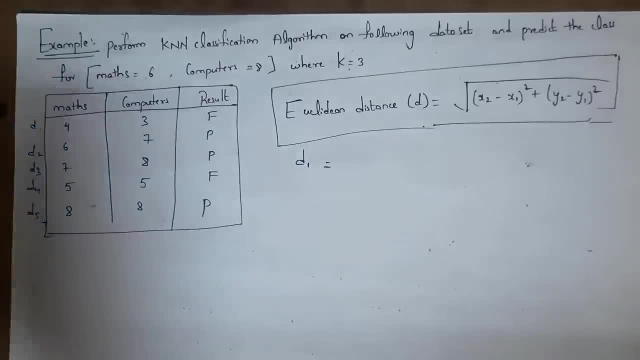 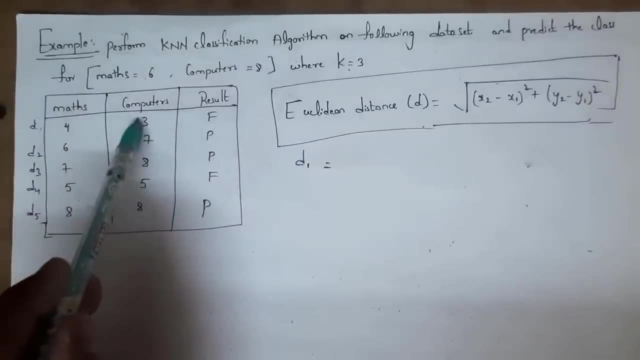 We need to find Euclidean distance for all these data. for example, these are the marks of students. For example, this data- one is marks of students- should be 0. one got four marks in maths, three marks in computers and his result is failed. Similarly, 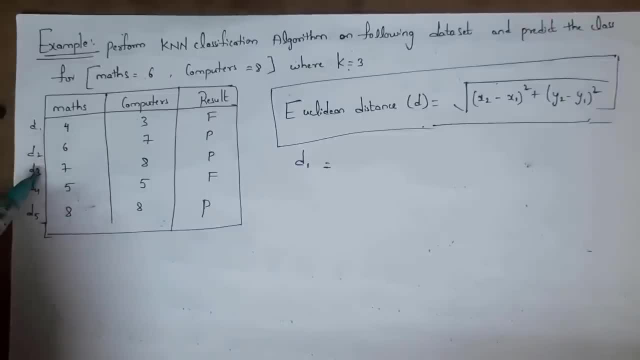 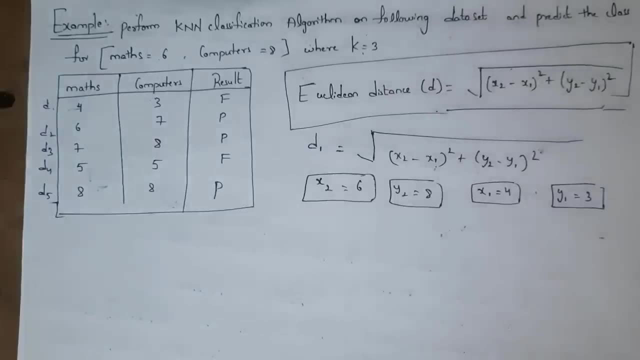 student two. I am considering student two as data two, student three as data three, student four as data four and student five as data five. These are the marks that students got. Now I am calculating distance for this d one data one. This is Euclidean distance formula that. 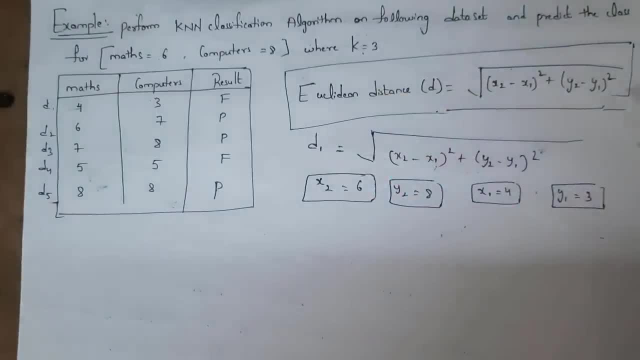 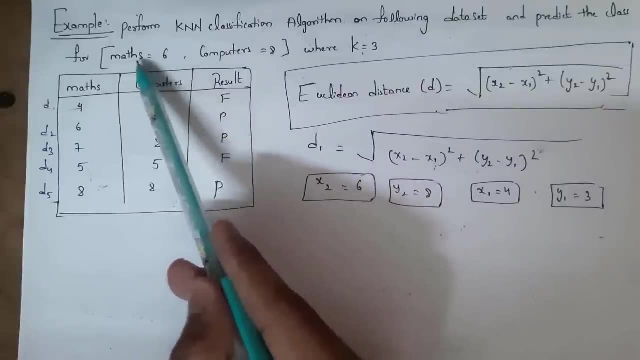 is under root of x two minus x one whole square plus y two minus y one whole square. Here, x two and y two are these values, which is given in question, which we need to find result. This is x two, mass equal to six, where six is x two and y eight is y two. And similarly with respect to 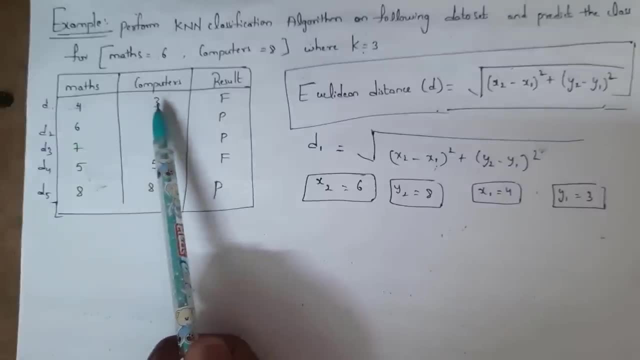 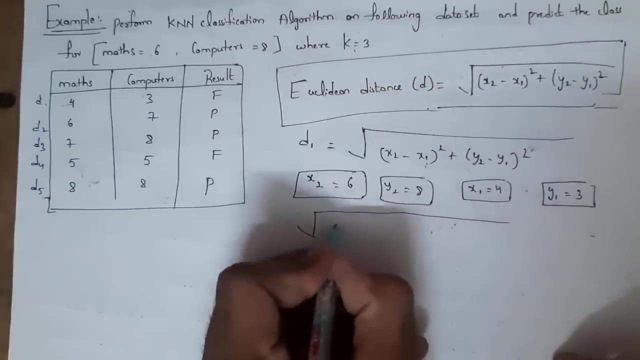 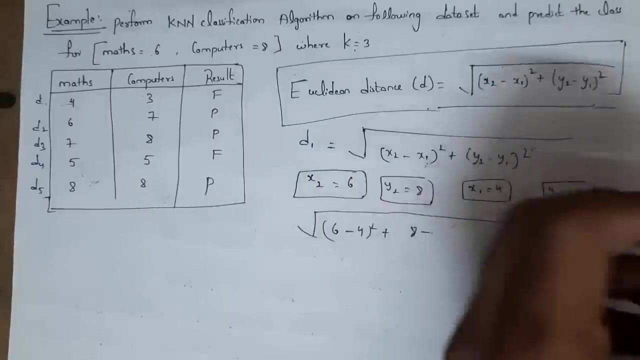 data: one here, x one is four and y one is three. Now we need to substitute these values in this formula that is under root of x. two is six, six minus x. one is four, six minus four whole square, plus y two is y eight, y eight minus three whole square. So result is under root of two square. 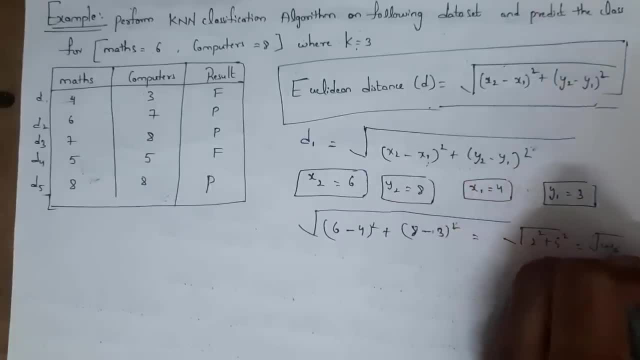 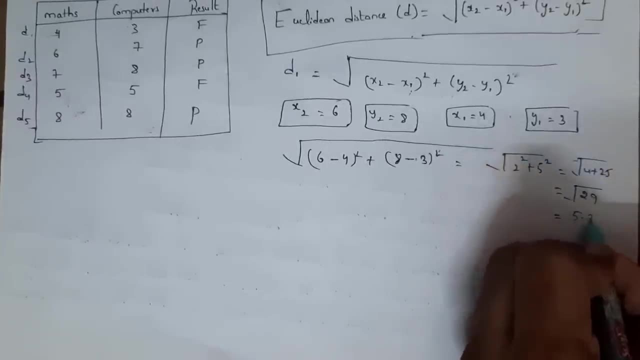 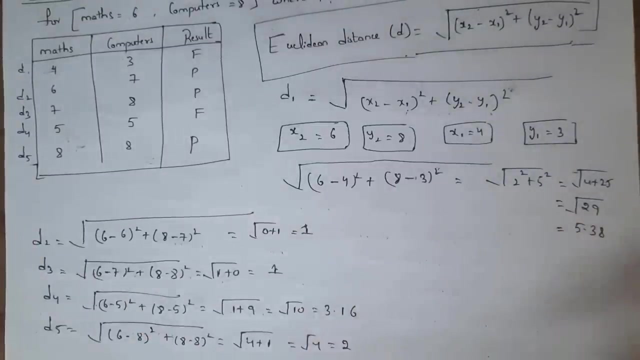 plus five, square, that is six. This is under root of four plus twenty five, equal to under root twenty nine. If you calculate this under root twenty nine, you will get this value. that is five point three, eight. We found distance for d one. Similarly, we need to find Euclidean distance for d two, d three, d four and d five. 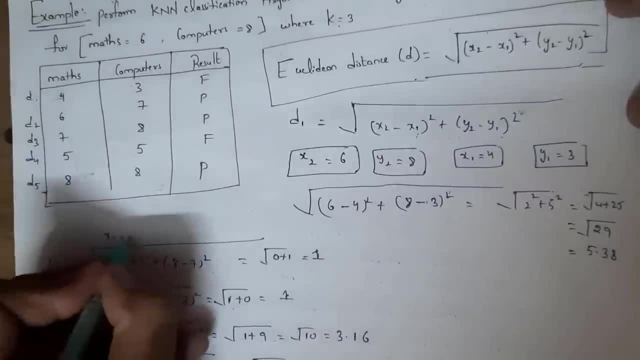 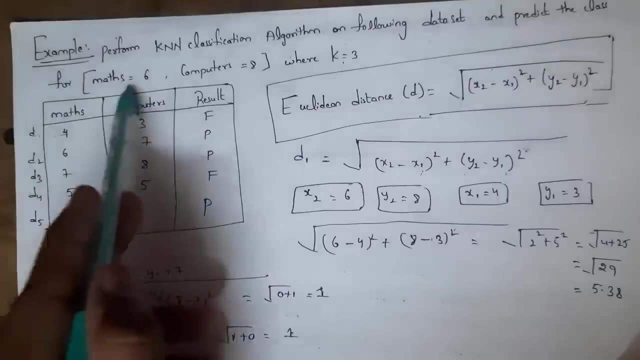 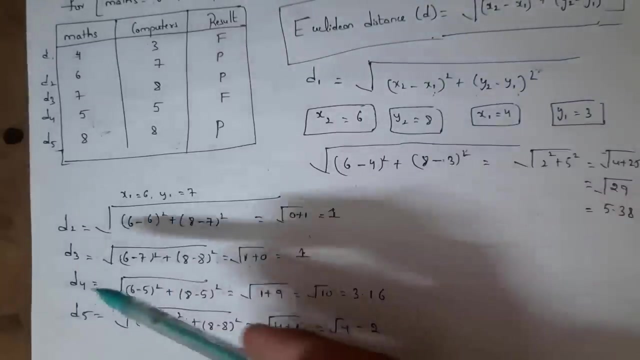 Here in d two, x one is six and y one is seven, six and seven, And whereas x two and y two is same. for all this, that is, x two is six and y two is eight. After substituting these values in this formula, I will get result as one. Similarly, for d three, result is one, and for 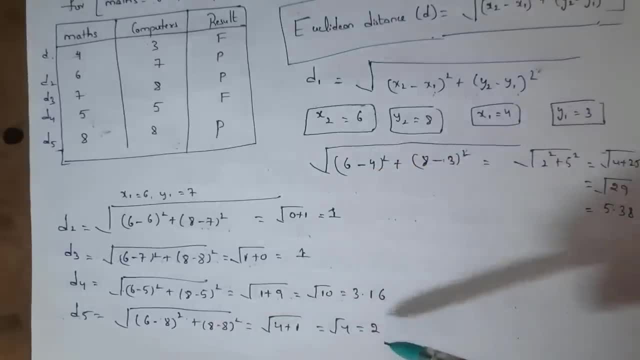 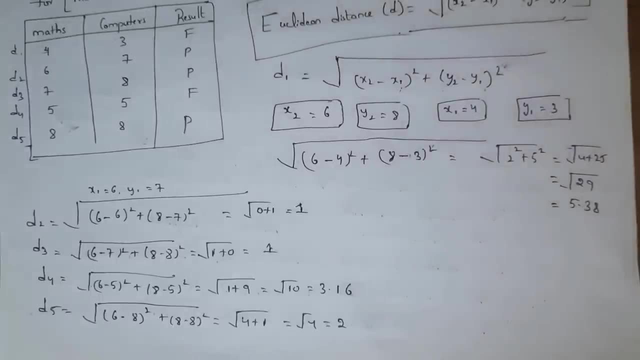 d four, result is three point one six and for d five, result is two. Here in question they given k equal to three. That means we need to consider three nearest neighbors. That is, we need to consider three smallest values from this: data one, data two, data three, data four and data five. 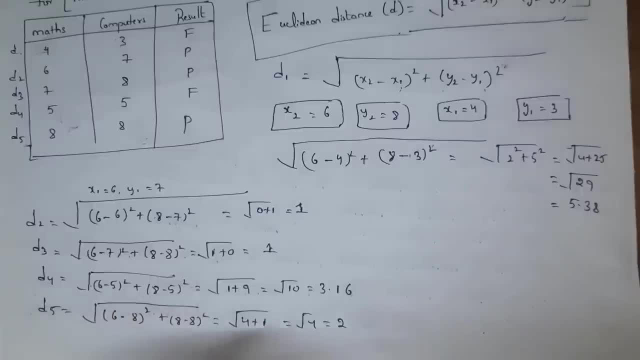 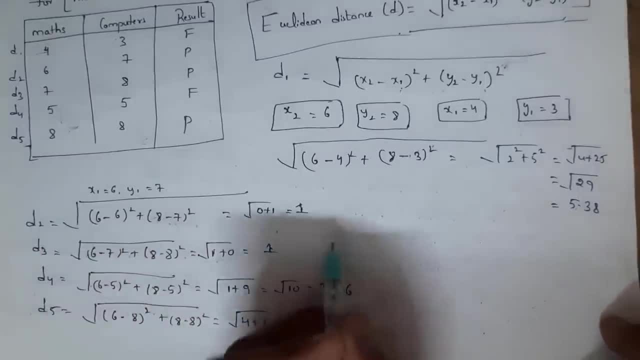 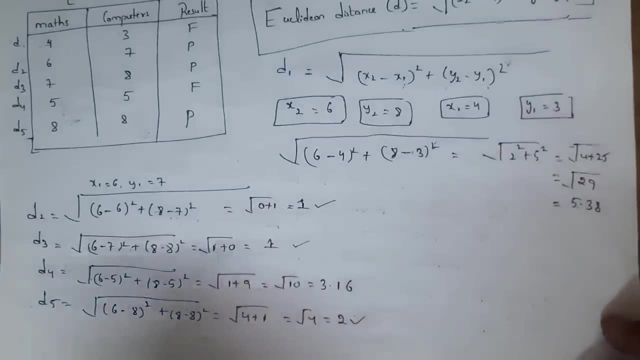 four is three and whereas d five is two. Out of this, d two is first smallest value, after that the d three is smallest, after that d five is smallest. These are the three smallest values I considered, because here in question they given k equal to three. So we need to consider. 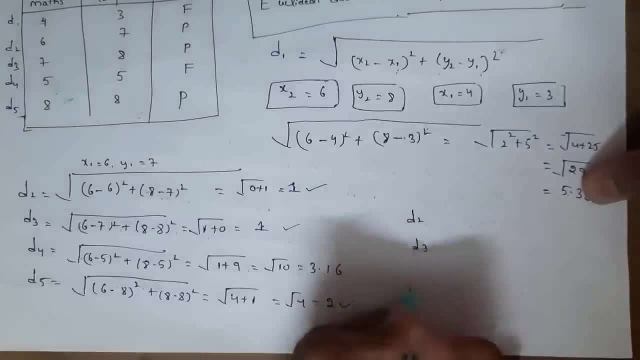 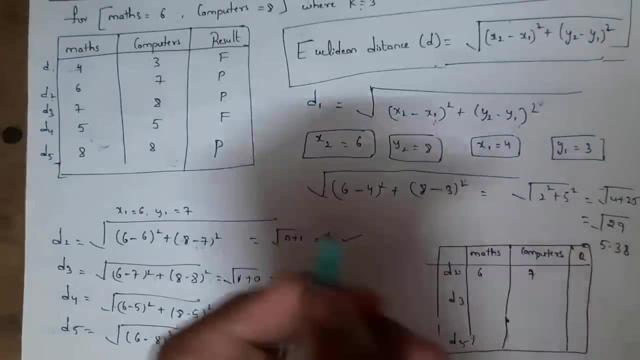 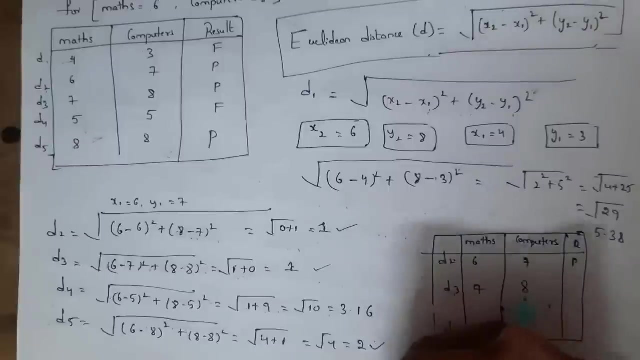 three smallest values Here I considered d two and d three and d five. Here d two is nothing but person two. Person two got six marks in maths and seven marks in computers, and his result is pass. Similarly d three- Person three got seven marks in maths and eight marks in computers, and his result is pass. 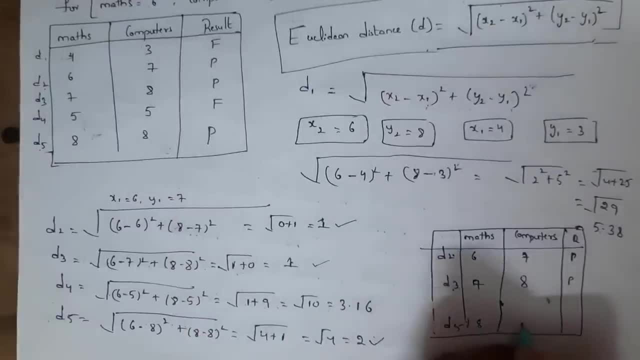 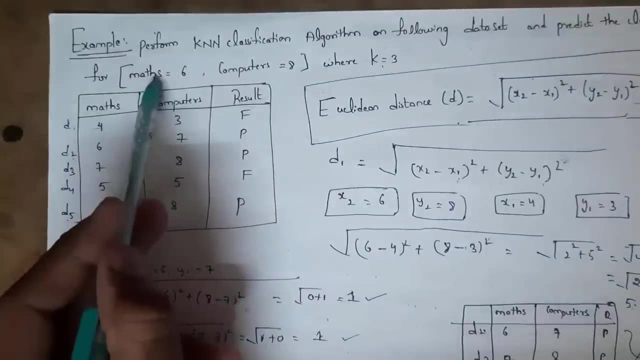 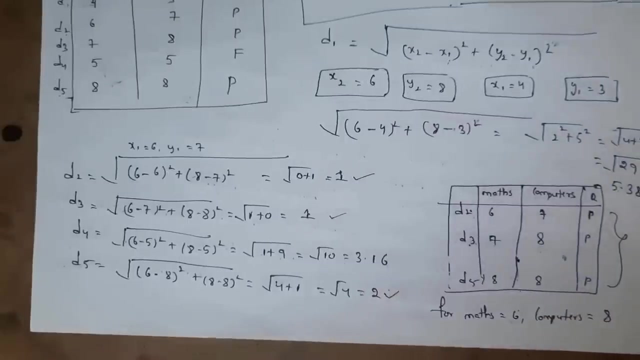 And similarly d five. d five got eight marks in maths and eight marks in computers and his result is pass. Majority of the result is pass. So for this new data, for this new student who got six marks in maths and eight marks in computers, his result is pass. So for maths is equal to six and for computers is: 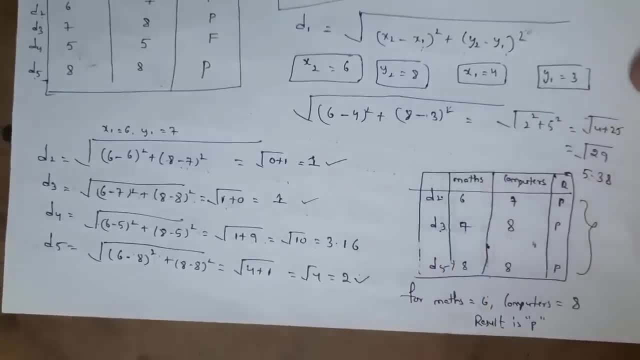 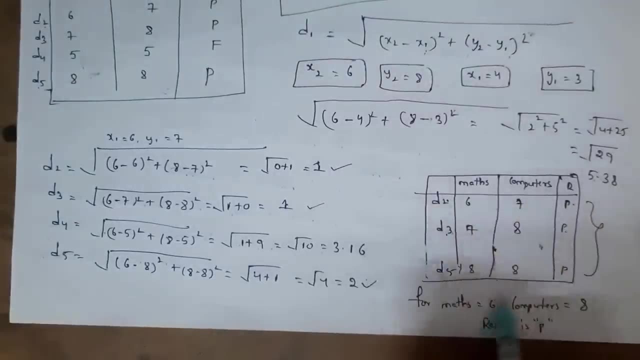 equal to eight, result is pass. This is final result of the new data. We need to consider result based on the majority. here majority of the student got pass mark. so here for new data, result is pass. for example, here for student 2, result is fail. even though result is fail, we need to. 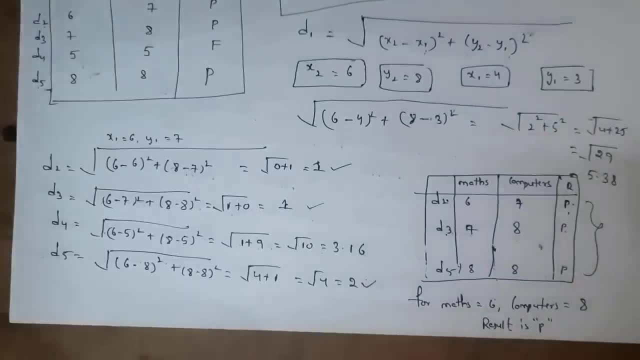 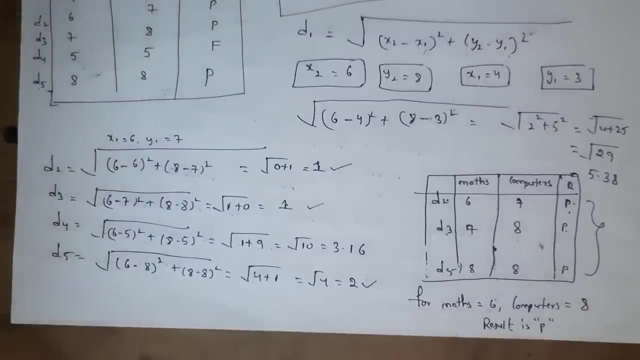 consider majority. one fail, two pass, so we need to consider pass. for example, all these three student. result is fail, so in that situation we need to consider majority. all are failed, so result is fail. for new data also, result is fail. i hope you have understood, guys. if you get this k in n algorithm. 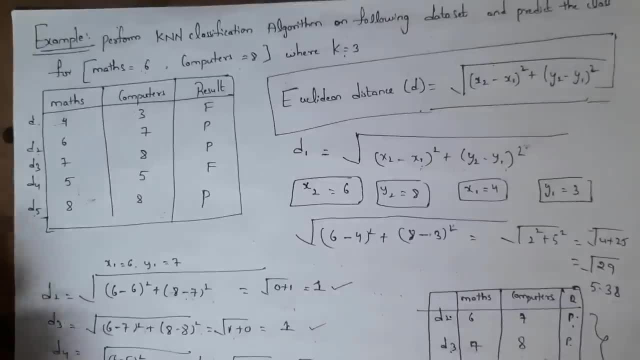 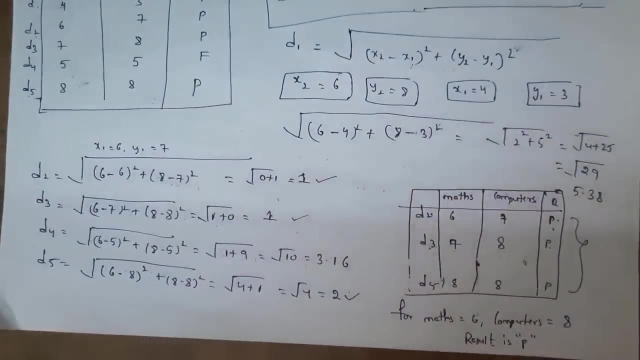 question in exam. definitely you need to write this example, otherwise you will not get marks. so definitely write this example in examination. based on these three nearest neighbors, we decided result of new data. now i will explain k in n algorithm. in step one we will select k- number of neighbors. 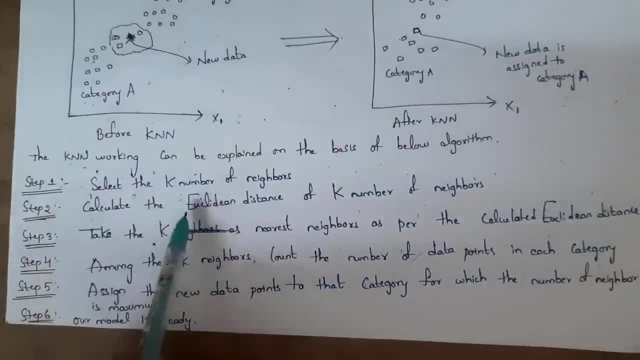 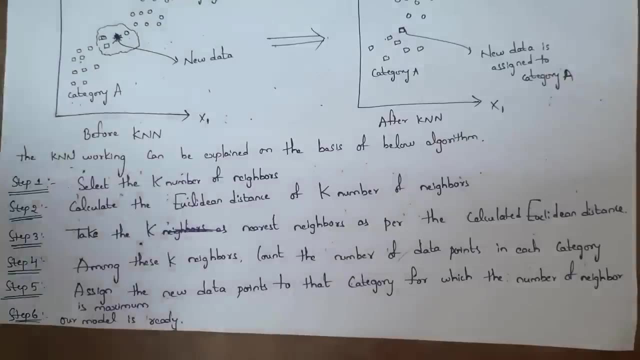 and after selecting k number of neighbors, we need to calculate euclidean distance for this neighbor. here we selected k neighbors. we calculated Euclidean distance for these neighbours. After that, in step 3, we need to select nearest neighbours based on the condition if they given k equal to 3, then we need to select. 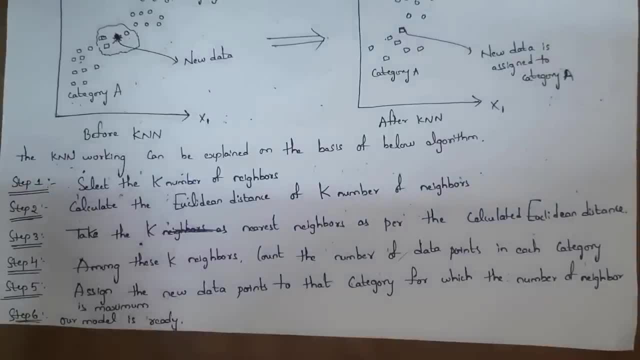 3 nearest neighbours. if they given k equal to 2, then we need to select 2 nearest neighbours Based on the condition. we need to select nearest neighbours as per Euclidean distance and in step 5, we need to assign our new data to any of the category based on the majority and at last, in 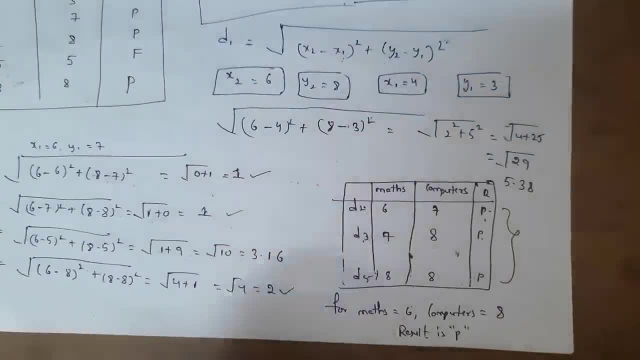 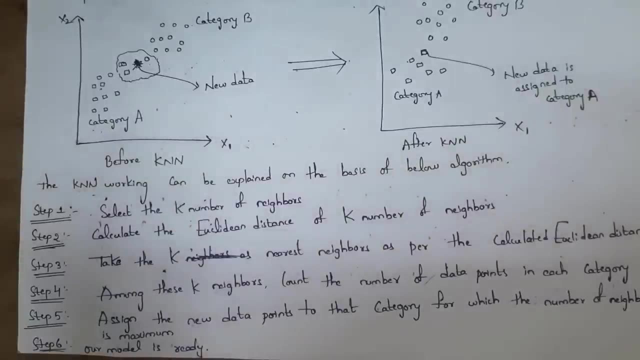 in step 6: our model is ready. in step 5, we assigned value based on the majority. here, majority is pass, so i assigned value as pass and it lost. in step 6: our model is ready. this is knn algorithm. next topic is navbase classifier algorithm. navbase algorithm is a supervisor learning algorithm. 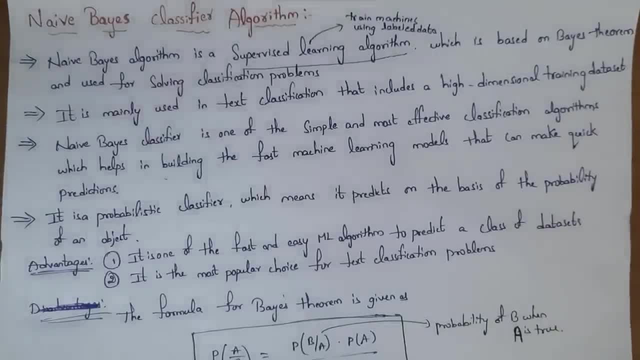 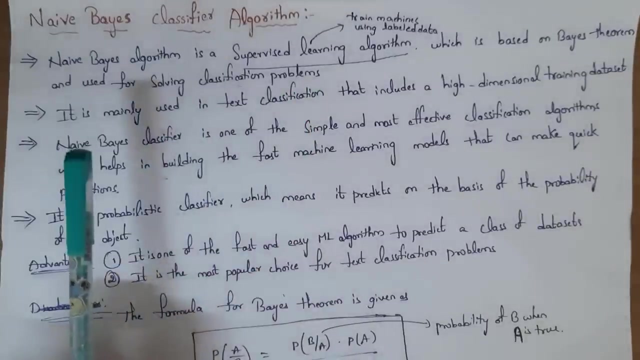 supervisor learning algorithm. in algorithm which uses labeled data to train machines. labeled data mean data which contains both input and as well as output, and navbase classifier algorithm is based on base theorem and user for solving classification problems. the name itself says navbase classifier algorithm. that mean this algorithm uses base theorem in order to solve. 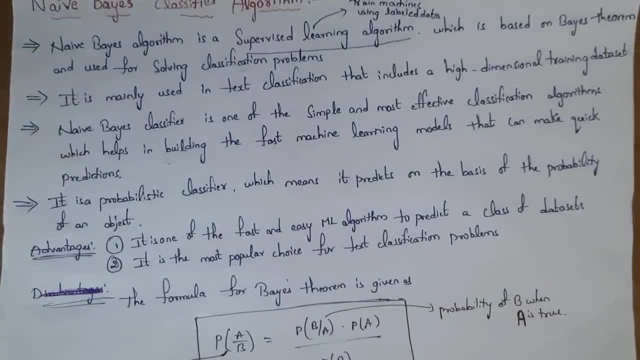 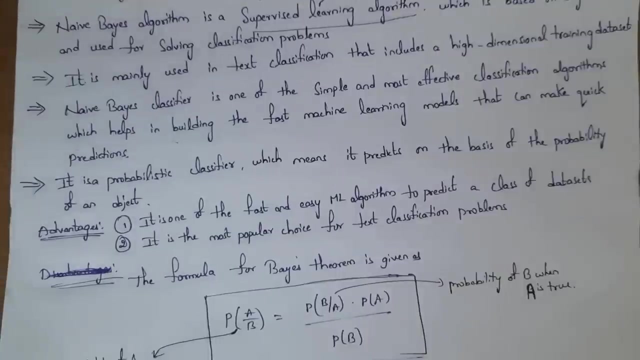 classification problems. this algorithm will solve classification problems, but mainly it is used to solve text classification problems which contains high dimensional training, data set and navbase. classifier is one of the simple and most efficient classification algorithm- most efficient mean which will give correct output. by using this algorithm, we can build fast machine learning models which will make quick predictions. 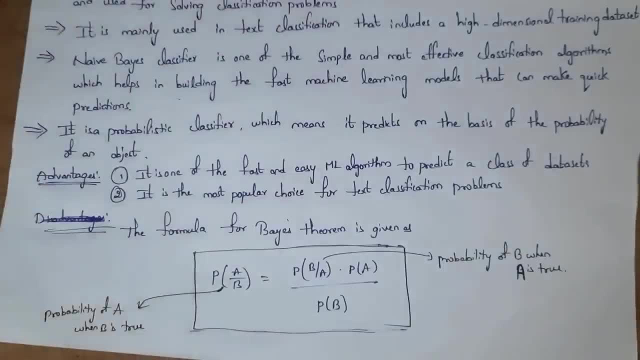 we can call this navbase classifier as probabilistic classifier, because it can predict probability of an object. these are the two advantages of navbase classifier. one is it is fast and easy machine learning algorithm. this is one of the advantage. it is fast and as well as. 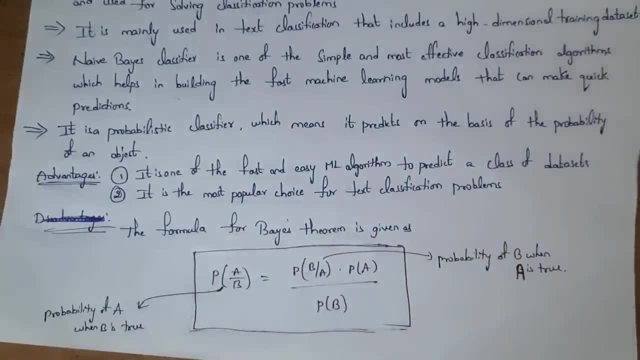 easy machine learning algorithm to predict class of a data set. class is nothing, but it can predict output easily. and second advantage is if you want to solve text based classification problem, then this algorithm is best choice. this is second advantage. but how can we solve this navbase? 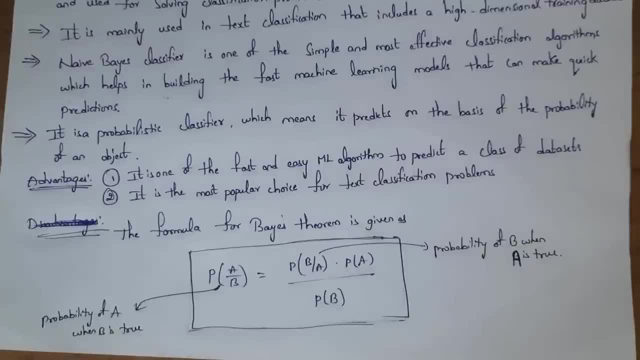 classifier problems, that is, by using base theorem. by using base theorem we can solve navbase classifier problems. this is formula of base theorem that is, probability of a by b is equal to probability of b by a into probability of a by probability of b. what is meaning of this probability of a by b? 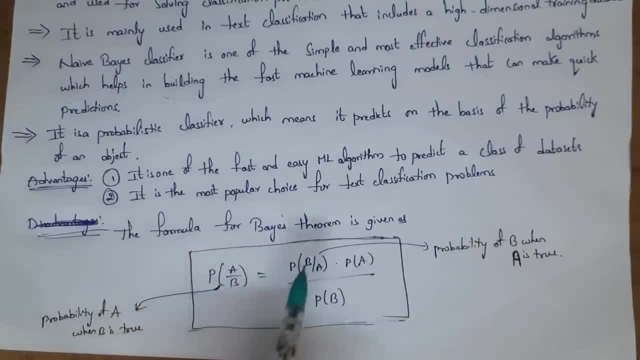 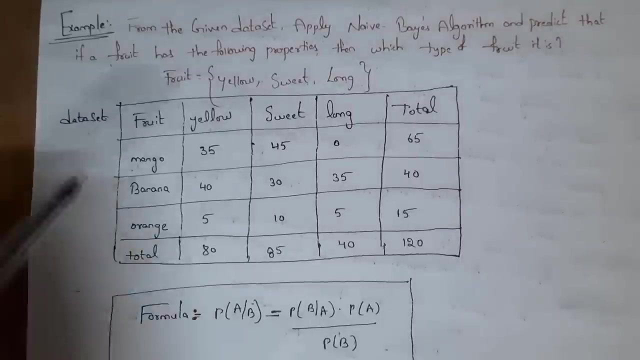 a by b: mean probability of a when b is true. b by a: mean probability of b when a is true. we can solve this problem by using this formula. i will explain one problem. this is a problem which we need to solve now. here, the given table. in table there are total three types of fruits. they are: 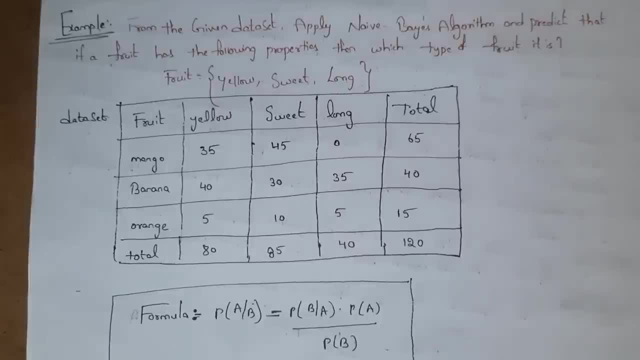 mango, banana and orange. total there are 65 mangoes out of 65 mangoes, 35 mangoes are yellow in color, 45 mangoes are sweet and 0 long and similarly total. there are 40 bananas. out of 40 bananas, 40 are yellow in color, 30 are sweet. 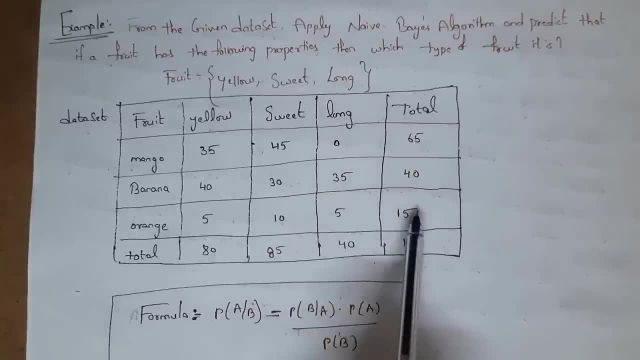 35 are sweet and 35 are long. similarly total, there are 15 oranges. out of 15 oranges, five oranges are yellow in color and 10 oranges are sweet and five oranges are long. total, how many fruits are yellow in color? 35 plus 40 plus 5, total 80. 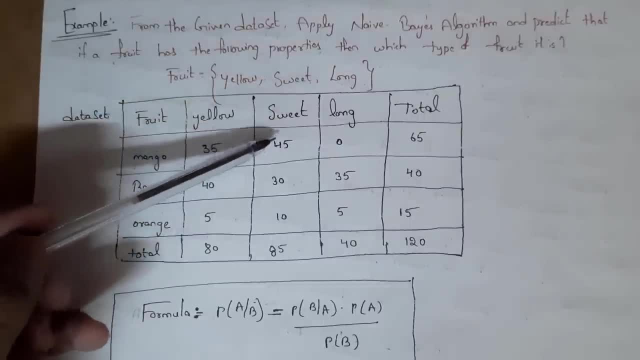 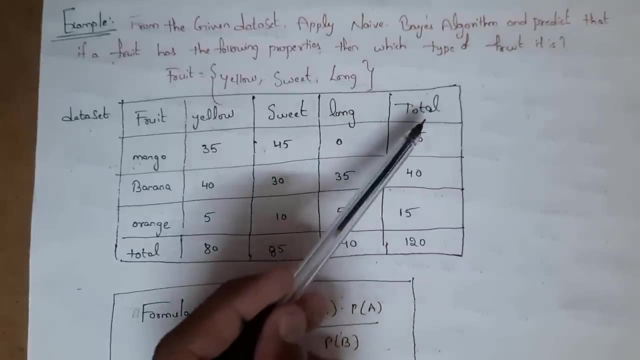 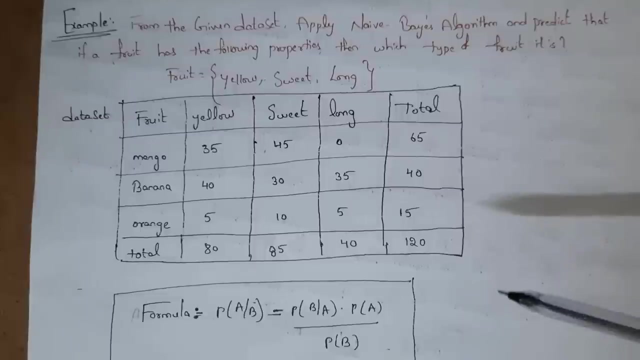 similarly, how many fruits are sweet: 45 plus 30 plus 10, that is 85. and how many fruits are long: 35 plus 5, that is 40. now we need to calculate total of all this fruits, that is 65 mangoes plus 40 bananas plus 15 total, 120 total. there are 120 fruits out of 120 fruits. 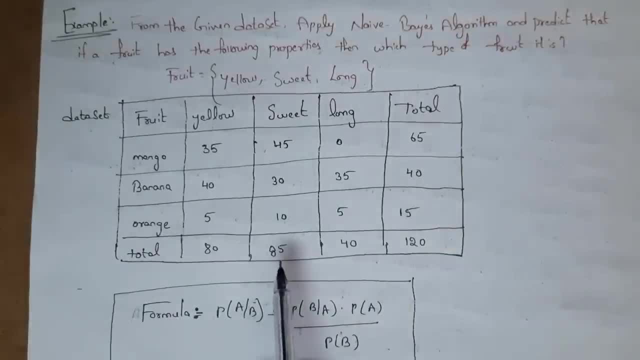 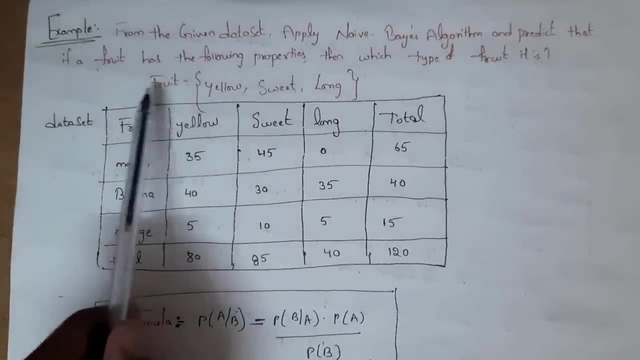 the 80 fruits are yellow in color and the 85 fruits are sweet and 40 fruits are long. this is stable. here in question, they given one new fruit. this fruit has following properties, that is, this fruit is yellow in color, this fruit is sweet and, as well as it is long. now we need to. 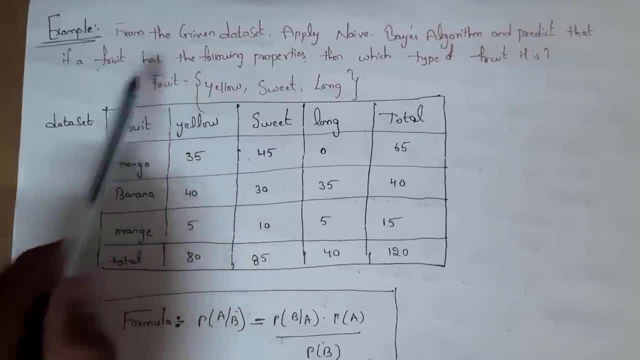 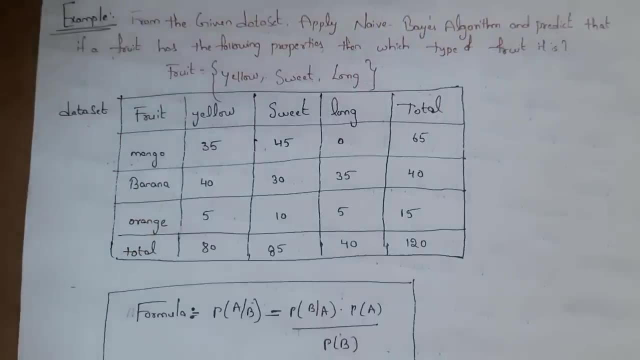 find to which category this fruit belongs to. either this fruit belongs to mango, or this fruit belongs to banana, or this fruit belongs to orange. we need to find this by using navibase algorithm. I need to find this. for this, I use Bayes theorem formula. this is Bayes theorem formula, that is. 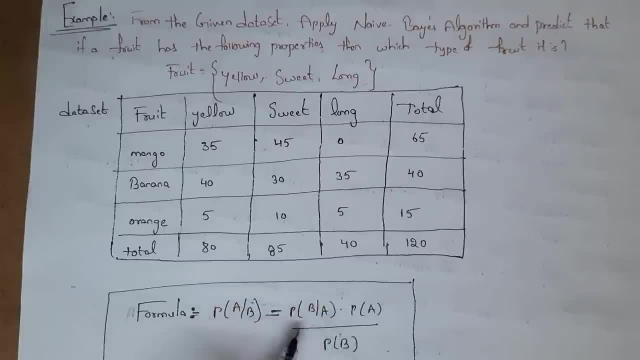 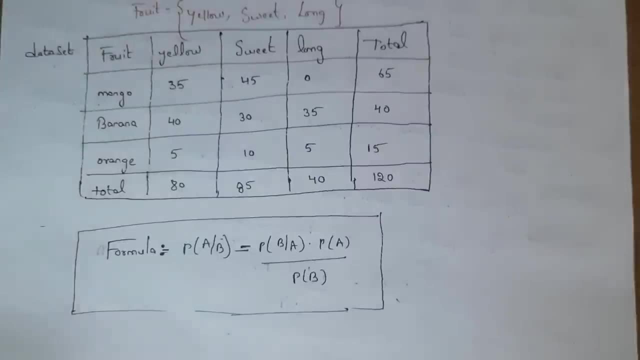 probability of a by b is equal to probability of b by a into probability of a by probability of b. this is main formula which we need to remember to solve this problem. here in question, they given three fruits. they are mango, banana and orange. so we need to calculate probability for mango. 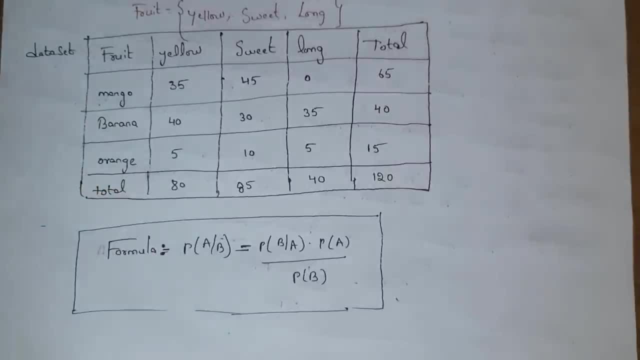 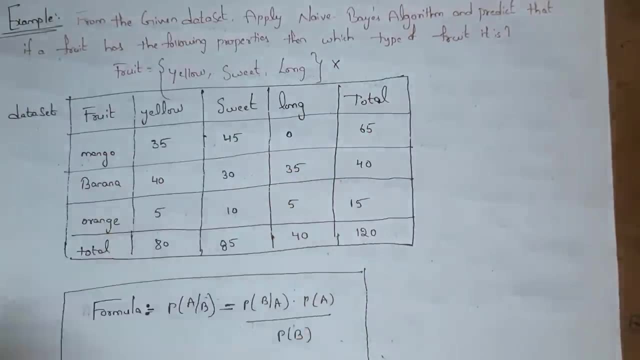 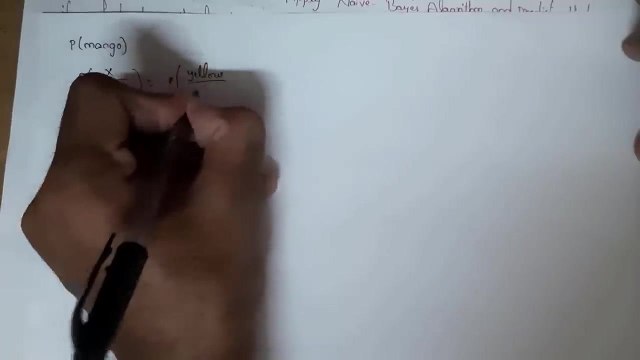 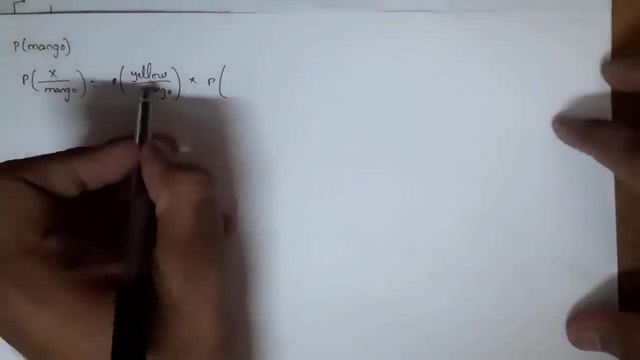 and probability for banana and probability for orange. let first I'm calculating probability for mango. let this new fruit be x. I'm considering this new fruit as x. so here probability of x by mango is equal to probability of lo by mango into probability of here there are three properties. now loi, sweet, long. so here probability of lo by mango into 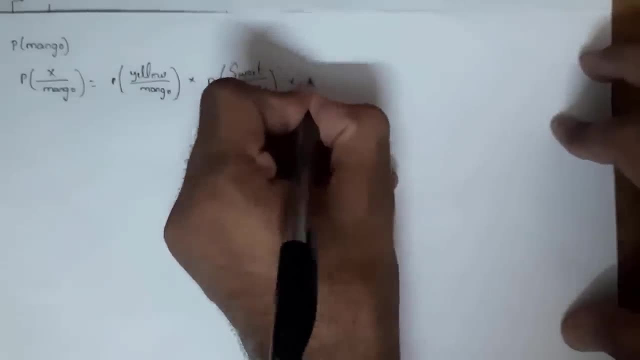 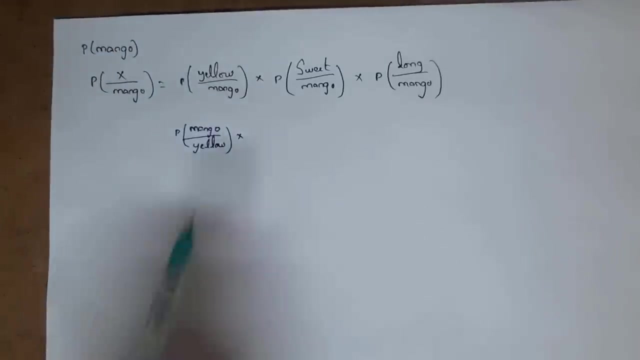 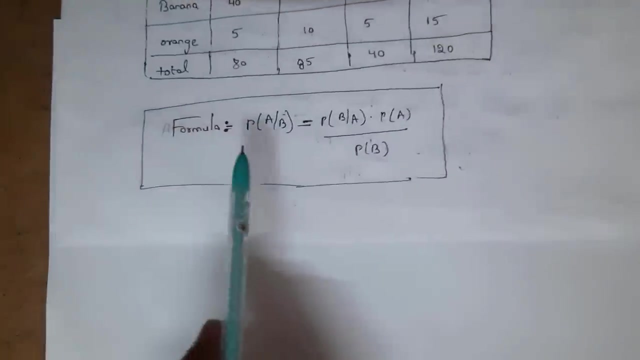 probability of sweet by mango into probability of what is taught property. that is long probability of long by mango. Now I am applying Bayes theorem formula for these three. First I am applying Bayes theorem for this probability of yellow by mango. What is Bayes theorem formula? That is probability of a by b. 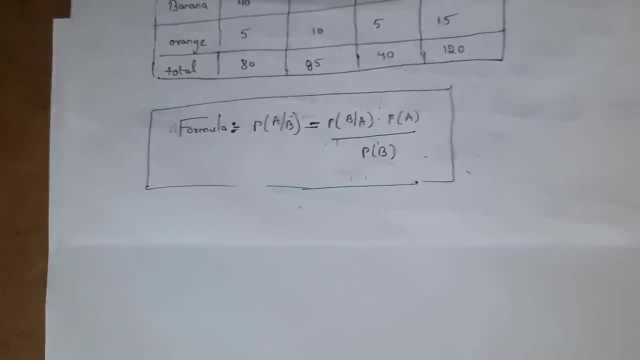 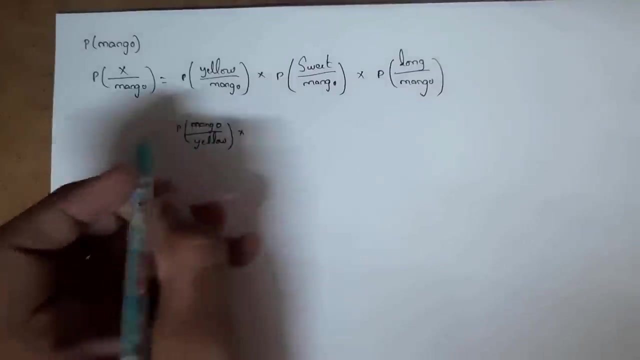 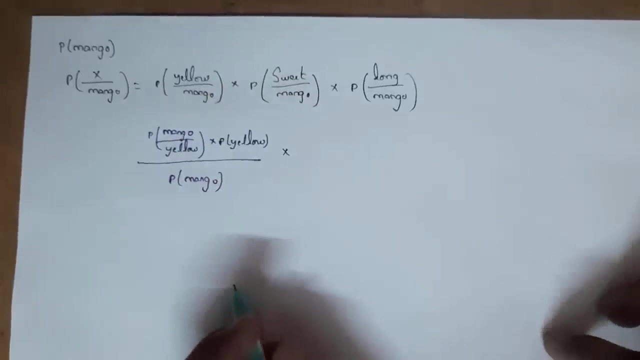 is equal to probability of b by a into probability a by probability b. That is, probability of yellow by mango is equal to probability of mango by yellow into probability of yellow by probability of mango. Similarly, now I am applying Bayes theorem for this probability of sweet by mango. 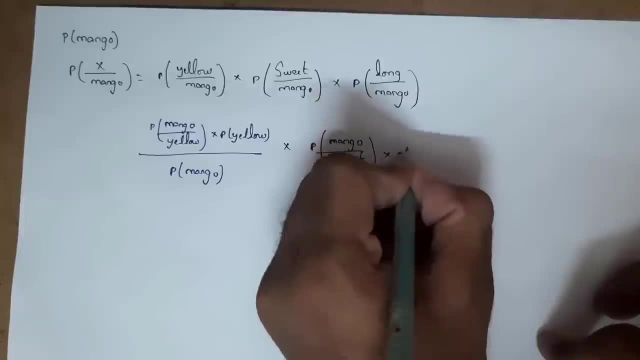 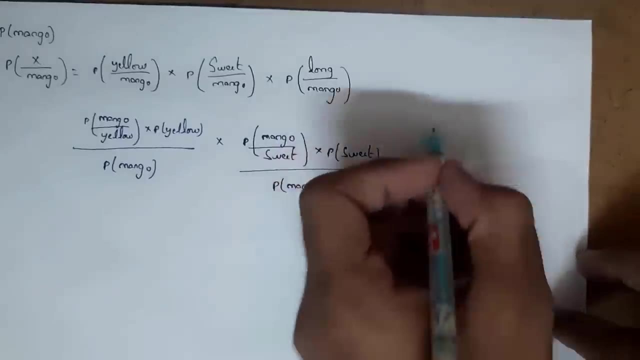 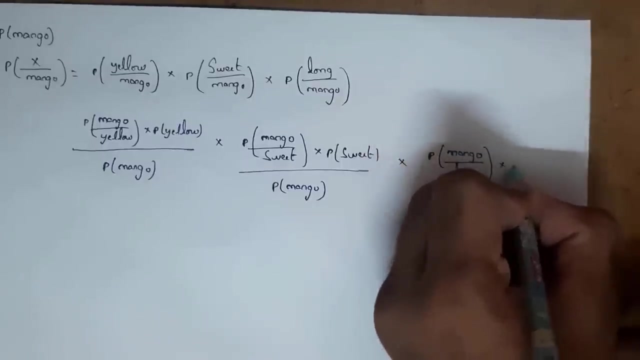 Formal is probability of mango by sweet into probability of sweet by probability of mango. Again, we need to apply Bayes theorem formula for this probability of long by mango. Probability of long by mango is equal to probability of mango by long. long into probability of long. 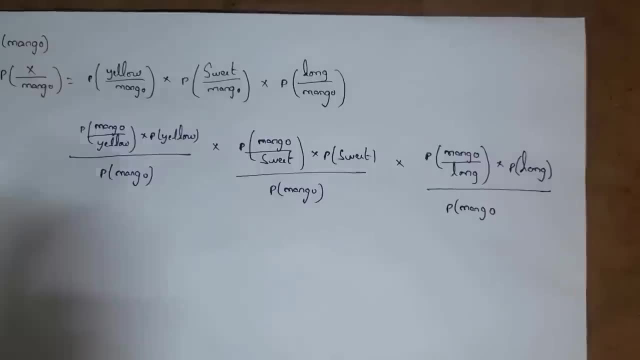 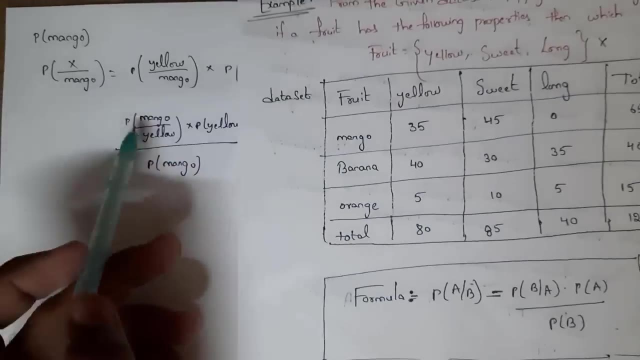 by probability of mango. I applied Bayes theorem formula for these three. Now we need to write values for this. What is value of probability of mango by yellow by seeing this table? What is probability of mango by yellow? What is probability of mango by yellow? 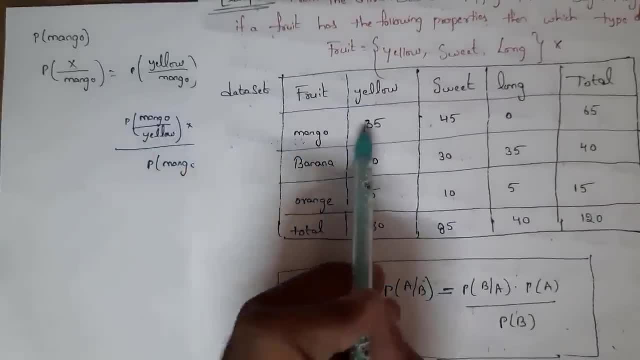 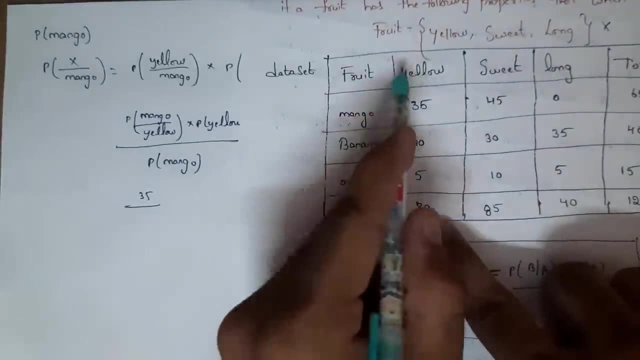 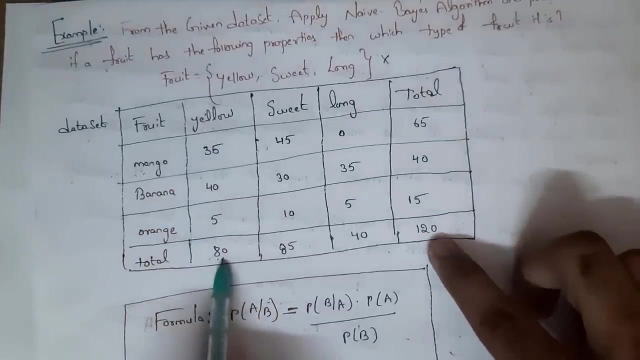 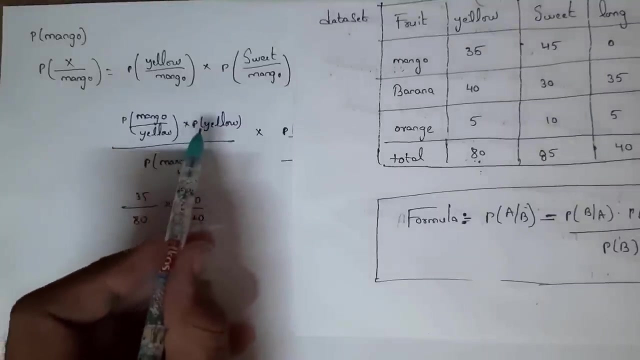 Probability of mango. when yellow is true, Probability of mango is 35.. 35 by what is probability of yellow, i t into what is probability of yellow. Probability of yellow is i t and total is 120.. So here i t by 120.. Whenever we get this like this probability of yellow, then 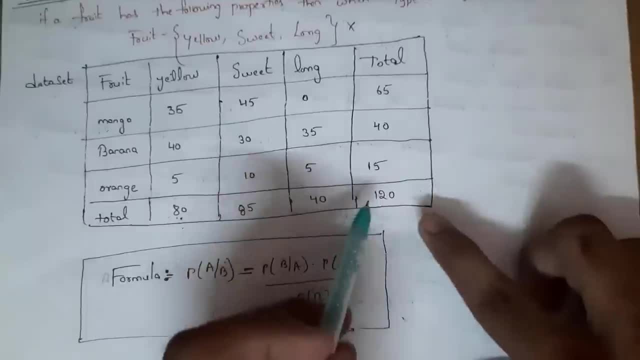 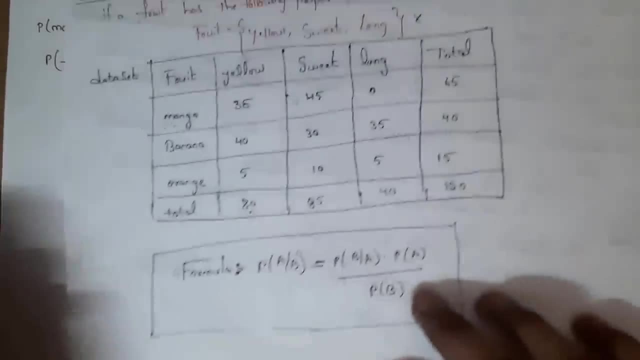 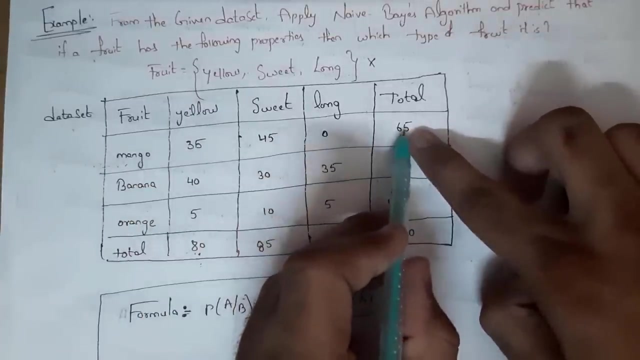 we need to write probability of yellow by total. Total is 120. So I written i t by 120 by what is probability of mango? Probability of mango is 65.. How many mangoes are there? Total 65.. So 65 by 120 into next probability of mango by sweet. 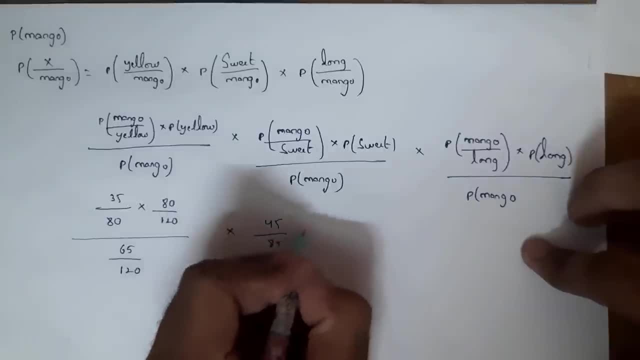 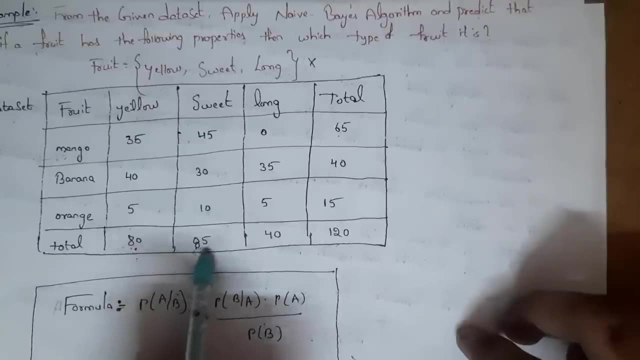 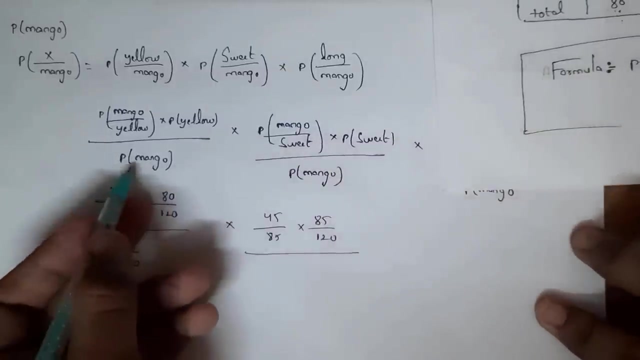 that is 45 by 85.. 45 by 85 into what is probability of sweet. That is total. how many fruits are sweet? 85.. That is 85 by 120.. And probability of mango: we already calculated probability of mango here. 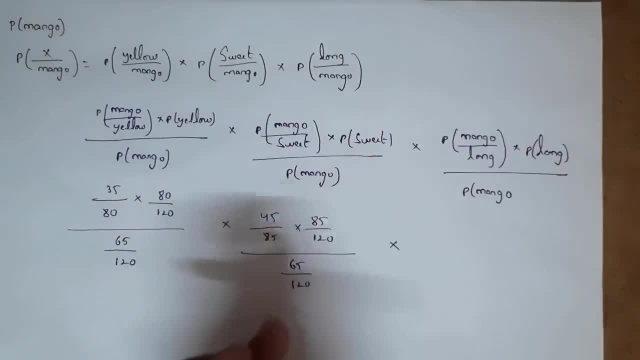 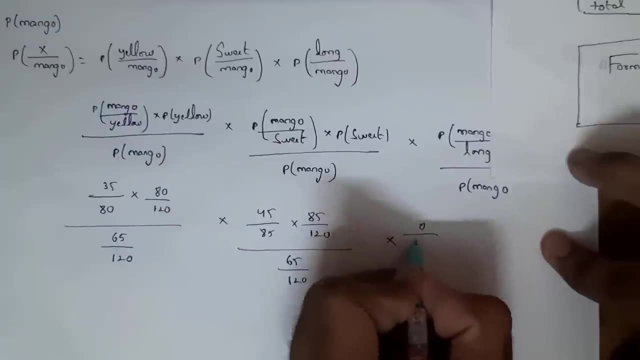 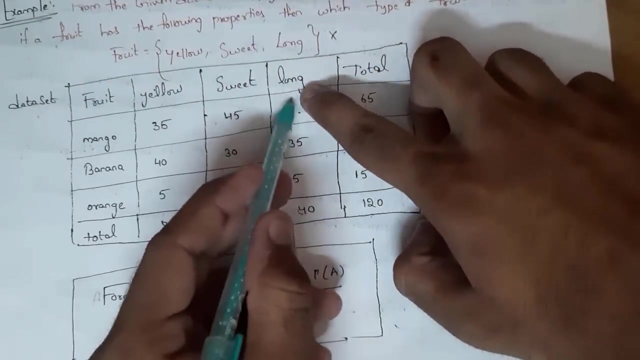 That is 65 by 120. into next probability of mango. by long, That is 0 by 40.. 0 by 40 into what is probability of long, That is 40 by 120.. By what is probability of mango, That is 40 by 120.. 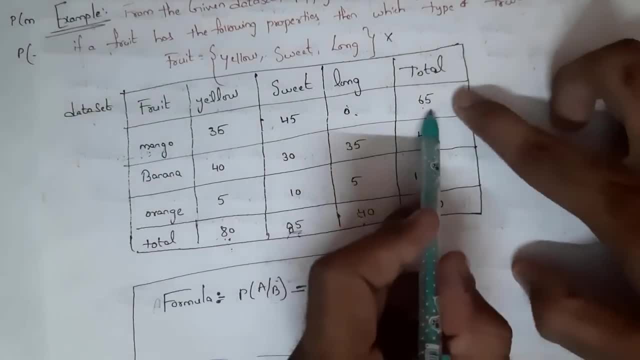 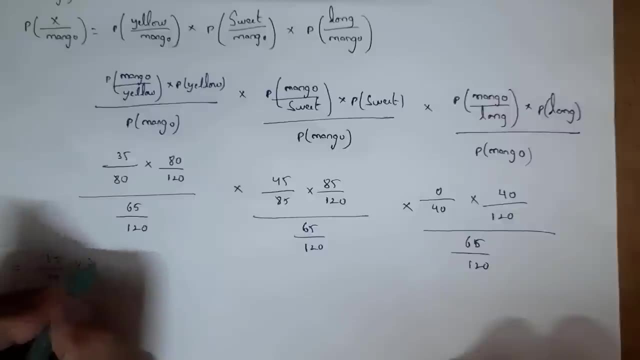 So 5 by 40. That is 20 by 40 into what is probability of mango. We have now calculated that thus far. We are done. now on probability of mango I will rub back here. So 1 by 40. 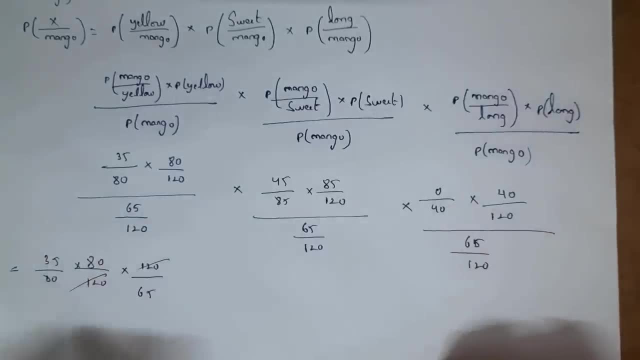 by 50 into scoredsecond probability of mango. suicide done counts here. So we now we are done with probability of mango. Probability of mango we have already calculated here. Probability of mango is 65 by 120.. 65 by 120.. 60 by 120.. What is probability of mango? Probability of mango is: 65 by 120.. 65 by 120. That is equal to 35 by i t into i t by 120 into. we need to bring this out, that is, 120 by 65.here, 120 by 120. cancel i t by i t. cancel into 45 by 85, into 85 by 120.. We need to bring. 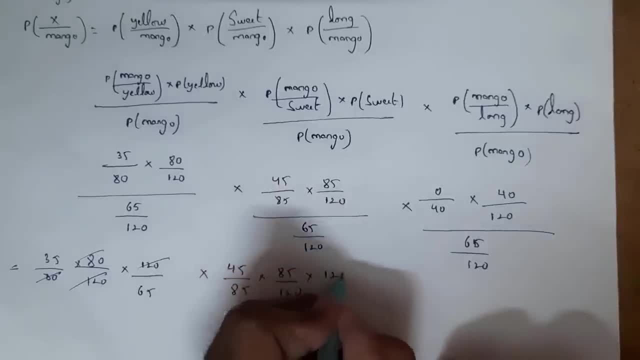 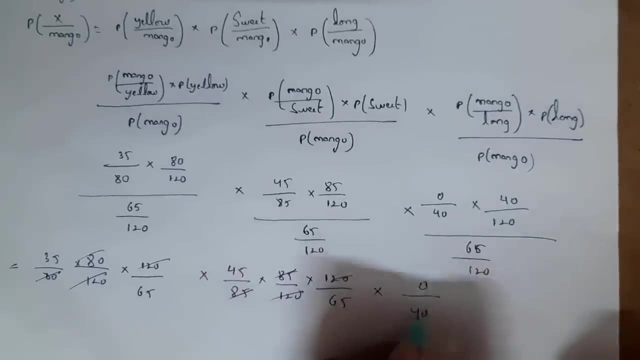 i t by 5 into 85 by 120.ает cf int too. tu EIT cell Cat is 0. we need to bring 120. we need to bring this up. that is, 120 by 65 here. 85, 85, cancel 120, 120, cancel. do 0 by 40. 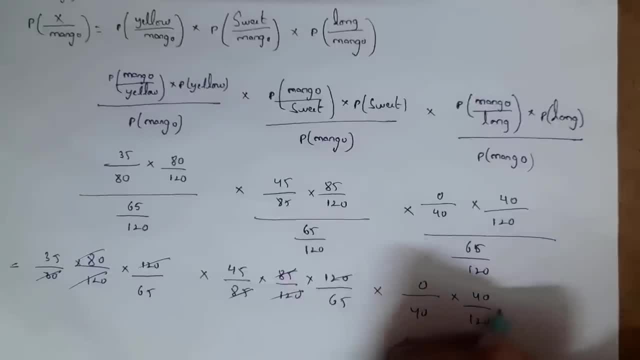 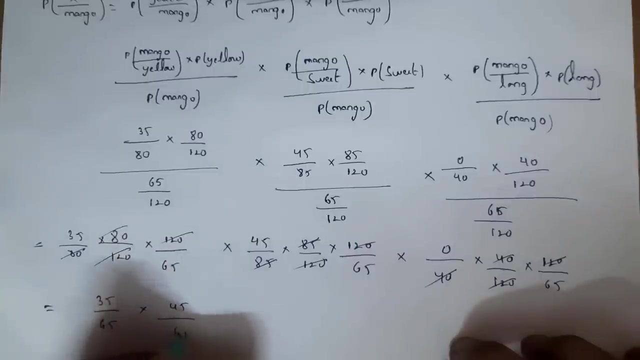 into 40 by 120 into- we need to bring this up- that is 120 by 65. here 120, 120 cancel, 40, 40 cancel. that is equal to 35 by 65 into 45 by 65 into 0 by 65. anything into 0 is 0, so here value is 0. 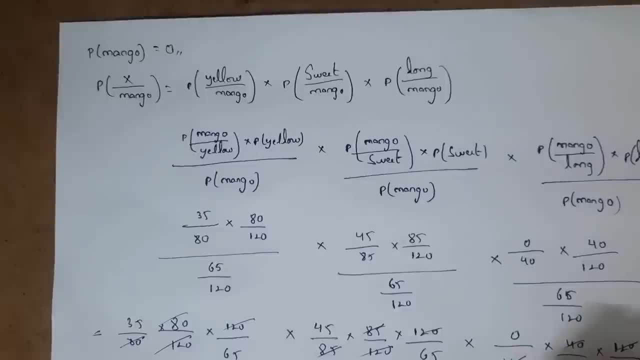 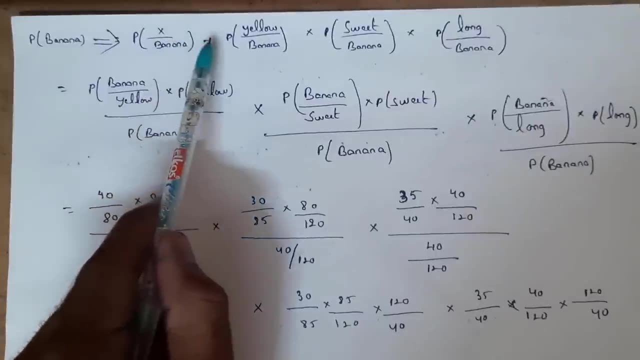 here probability of mango is 0. similarly we need to calculate probability for banana and orange. here i calculated probability for banana. probability of x by banana is equal to probability of ella by banana. into probability of sweet by banana, into probability of long by banana, applied base theorem. 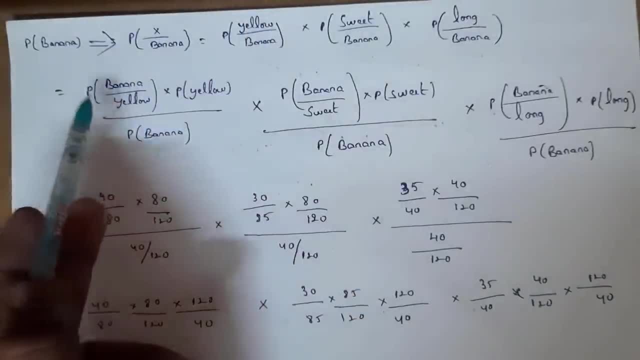 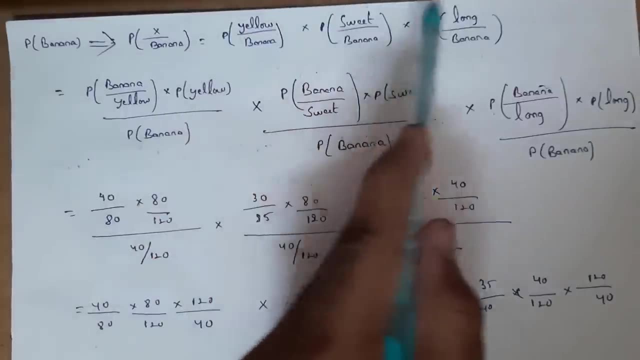 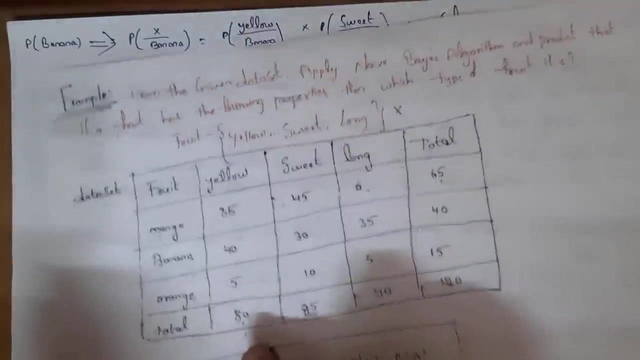 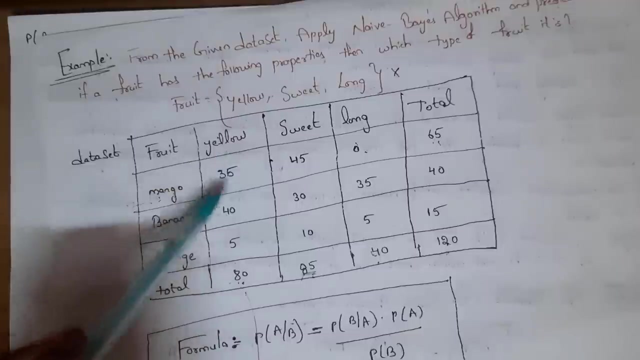 formula for banana. we need to apply base theorem formula for this three. after that we need to substitute values. that is probability of banana by probability of what is value of probability of banana. that is 40 by 8. here, probability of banana is 40, probability of. 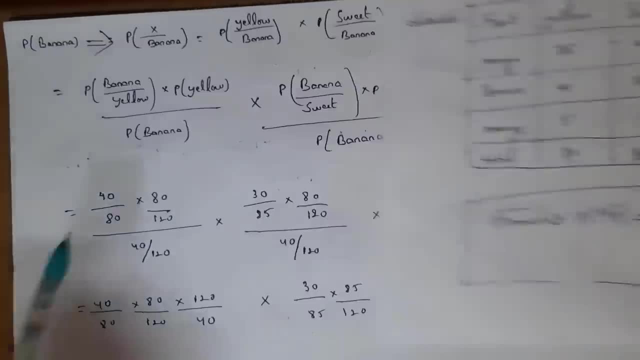 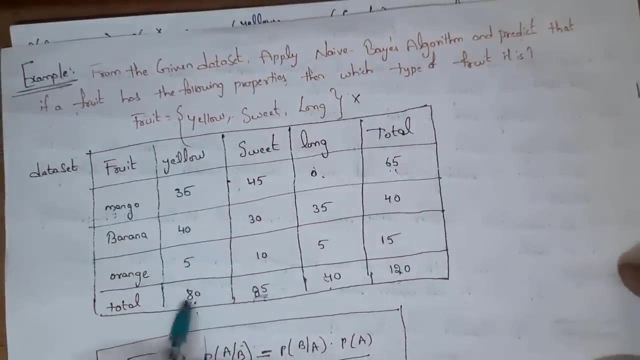 a law is 80 total. there are 80 other foods, so 80. that is 40 by 80 into what is probability by ay t, what is probability of yellow? that is iit total. iit yellow fruits out of 120 fruits. so here iit. 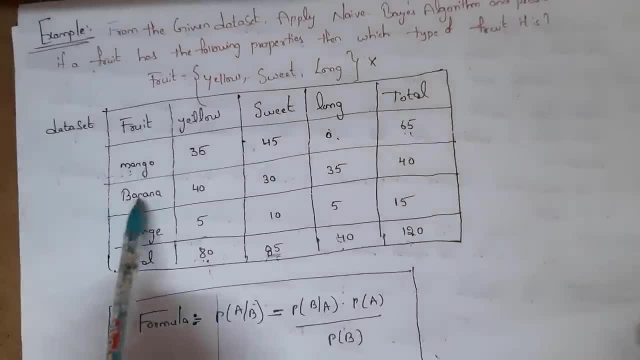 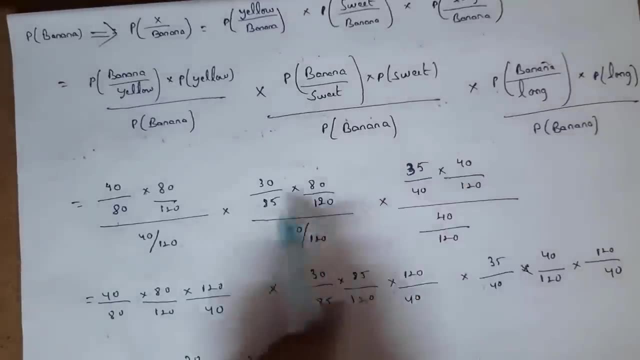 by 120. by probability of banana total, there are 40 banana fruits out of 120. so here 40 by 120. similarly, i written values for this too. so 40 by iit into iit by 120. we need to bring this up that. 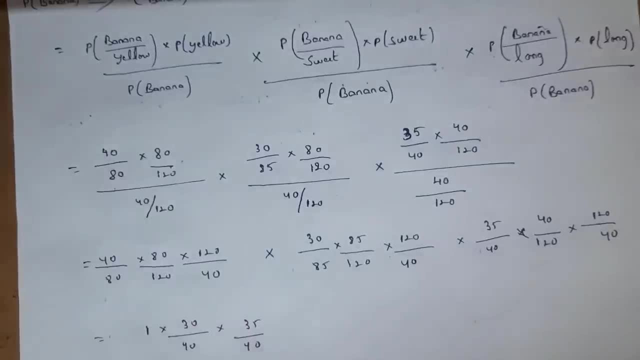 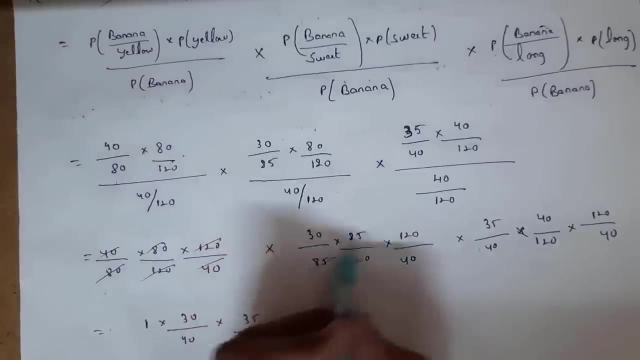 is 120 by 40. when we bring this up it will become 120 by 40. iit iit cancel, 120, 120 cancel, 40, 40 cancel. similarly here 85, 85 cancel, 120, 120 cancel. it will become 30 by 40. and here 40, 40 cancel 120. 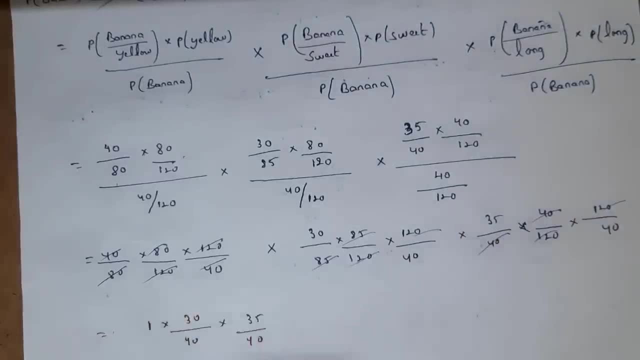 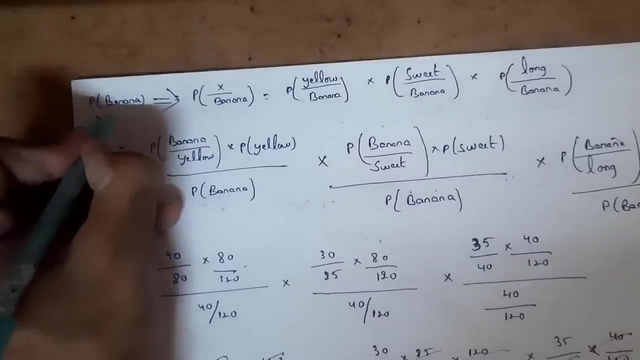 120. cancel 1 into 30 by 40, into 35 by 40. if we calculate this in calc, we will get value like this: 0.65. this is value of banana: 0.65. now we need to find probability for rnc. 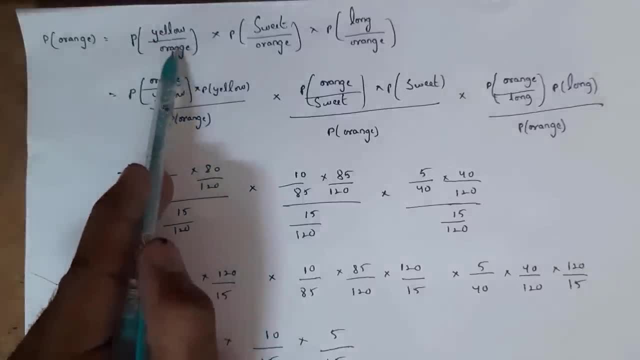 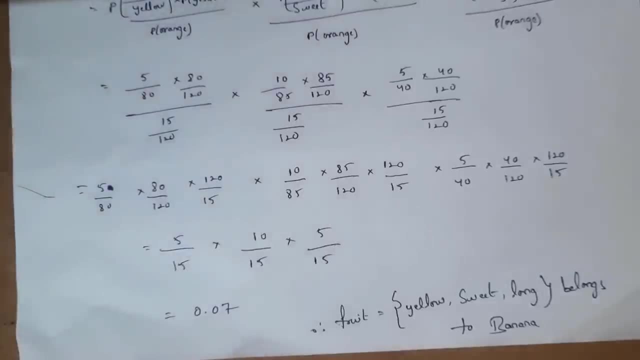 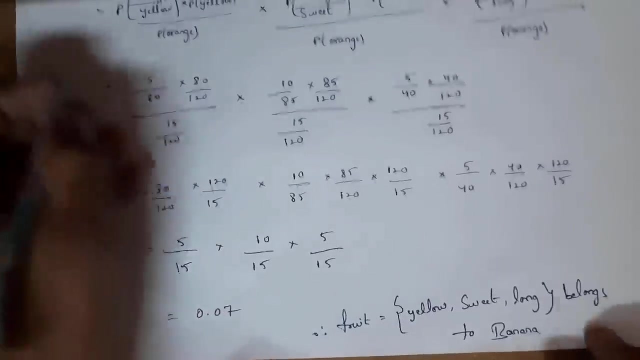 probability of x by rnc is equal to probability of yellow by rnc. into probability of sweet by rnc, into probability of long by rnc, after applying base theorem and substituting values, we will get probability of our rnc as we will get probability of rnc as 0.07. this is probability of rnc we got. 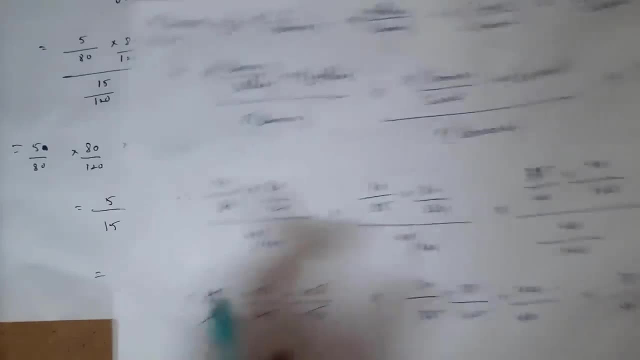 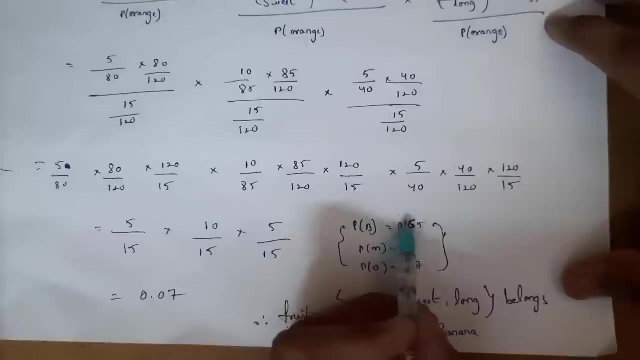 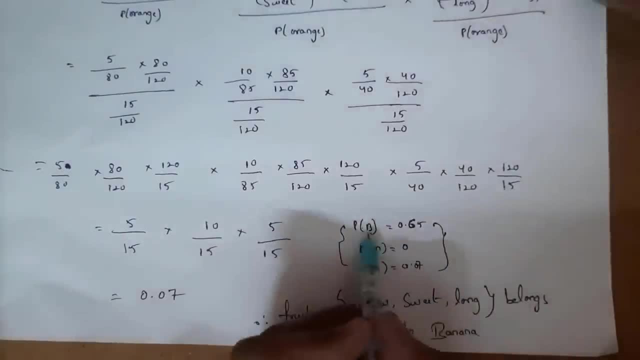 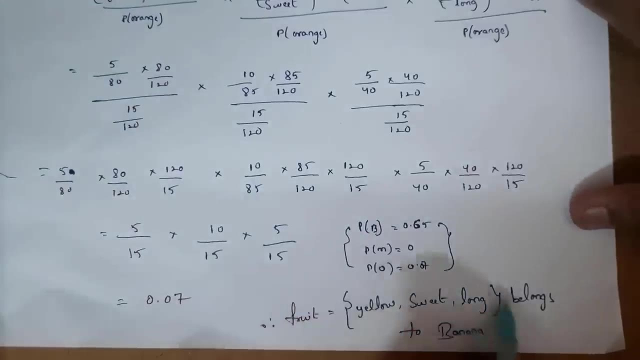 of rnc is 0.07 and probability of rnc is 0- 0.07. We have the three: 3 fruits. which fruit has the highest probability? that is, probability of banana has highest probability. that is 0.65. this is highest, so this fruit belongs to banana. this is output, that is, this new fruit with yellow sweet. 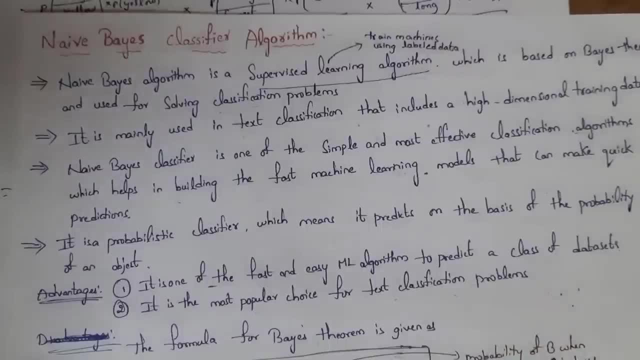 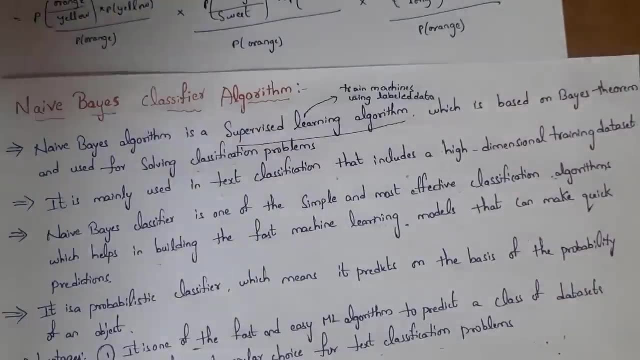 and long property belongs to banana guys. if base classification methods question comes into exam, then you need to write this base theorem formula and then you need to write this nav base classifier answer. that's it, because base classification methods are classified into two types: One is Bayes' theorem and the next one is Navibase classifier. 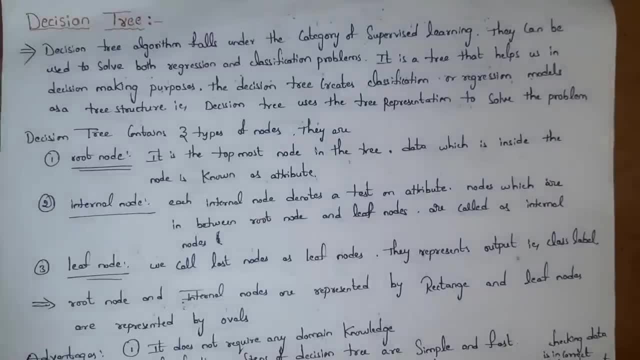 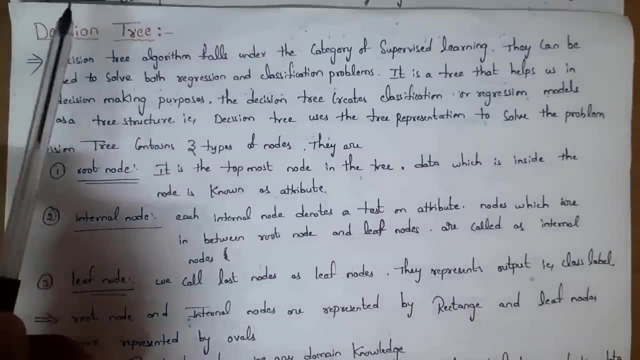 Next topic is decision tree. We also call this decision tree as decision tree classifier or decision tree induction. Decision tree is supervisor learning technique and by using this decision tree we can solve both classification problems and as well as regression problems. The name itself says decision tree. 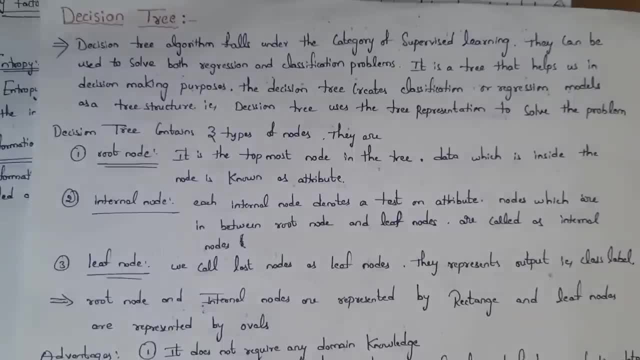 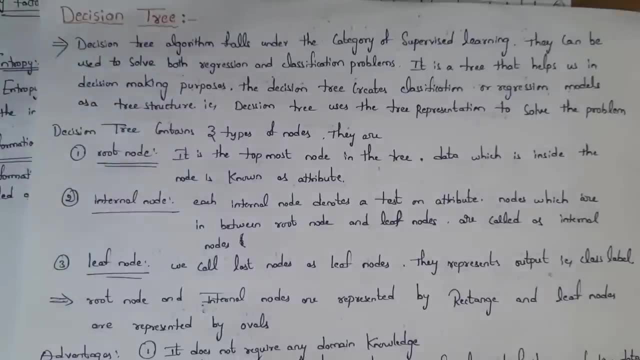 That means by using this tree, we can take decisions. This decision tree will represent a classification model and regression model in the form of tree structure. That means this decision tree is represented in the form of tree that is used to solve problem. Decision tree contains three types of nodes. 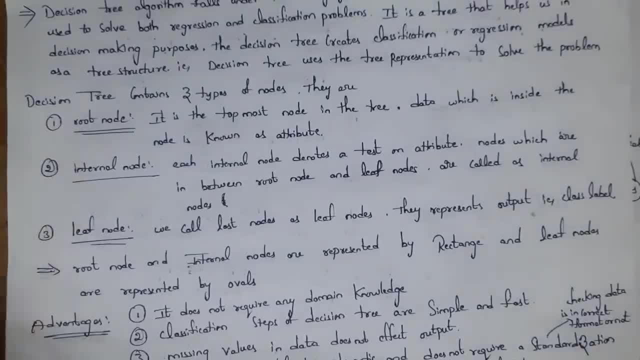 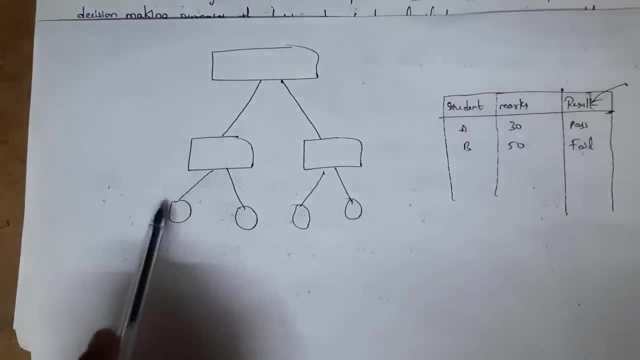 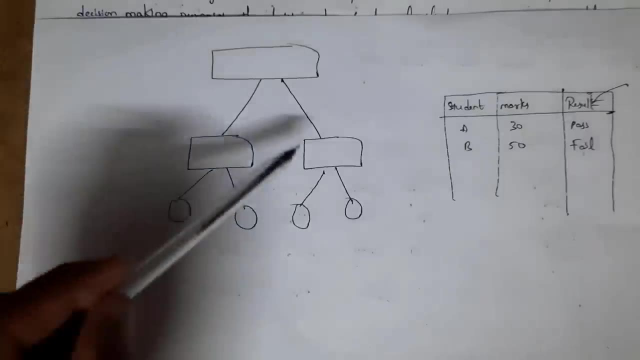 They are root node, internal node and last one is leaf node. For example, this is decision tree. In decision tree, topmost node is known as root node and last nodes are called as leaf nodes, and nodes which are in between this root node and leaf node is known as internal. 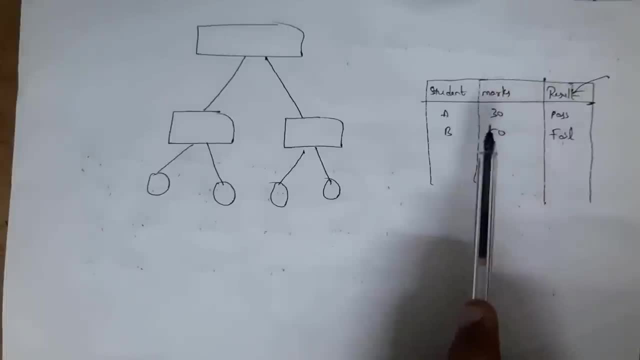 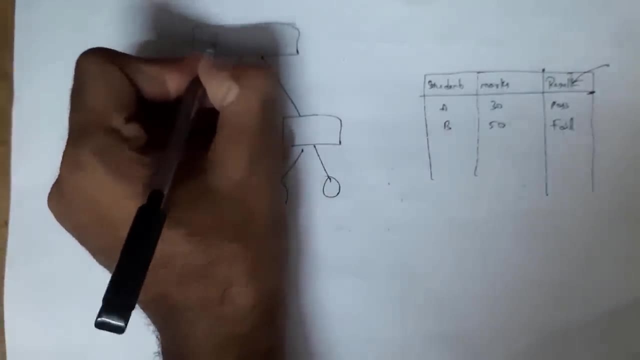 node, For example. this is table. This table contains three attributes. They are student marks and result In decision tree. we can store attributes inside the node. For example, we can store attribute student. This internal nodes represent test on attribute and whereas leaf node represent class label. 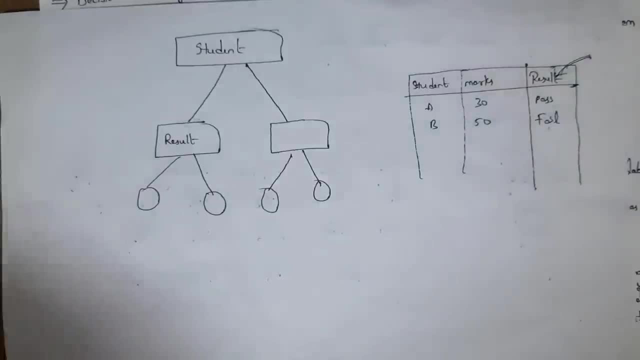 In this table. last attribute is known as class and data which is in this class is known as class label. There are two types of class labels in this table. They are pass and fail, So leaf node represent class label. That means we can write class label in this. 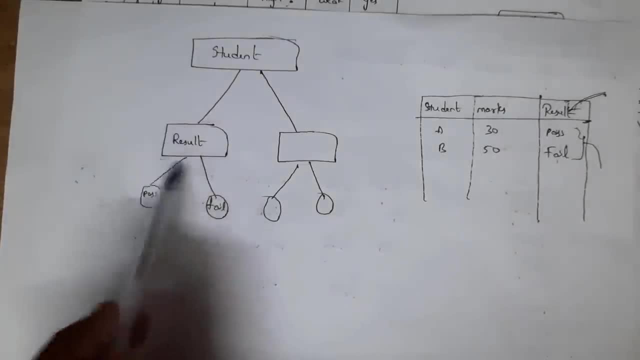 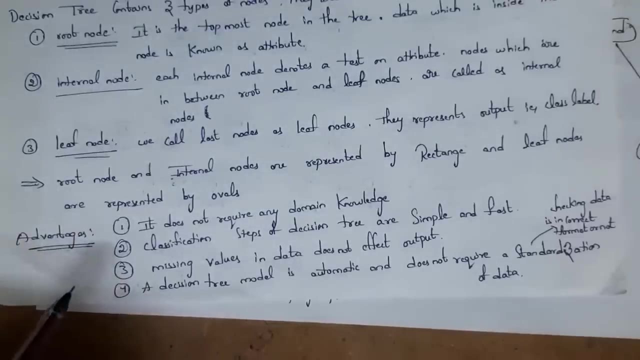 Pass and fail. Root node and internal nodes are represented by rectangle and whereas leaf node is represented by oval. These are the advantages of using decision tree. First advantage is it does not require any domain knowledge. People, those who don't have any domain knowledge, can also use this decision tree. 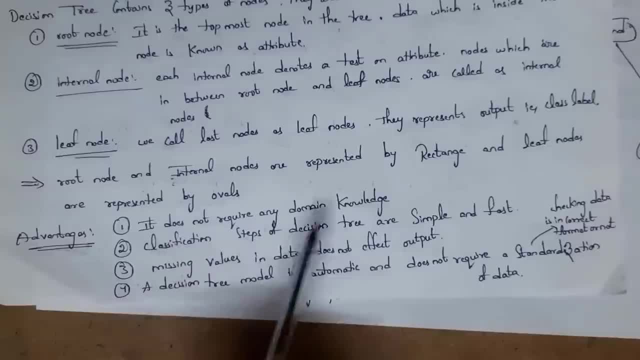 This is first advantage. and second advantage is classification steps of decision tree are simple and fast. Whatever the classification steps that this decision tree contains, the steps are very simple and as well as fast. And third advantage: Missing values in data does not affect output, though. 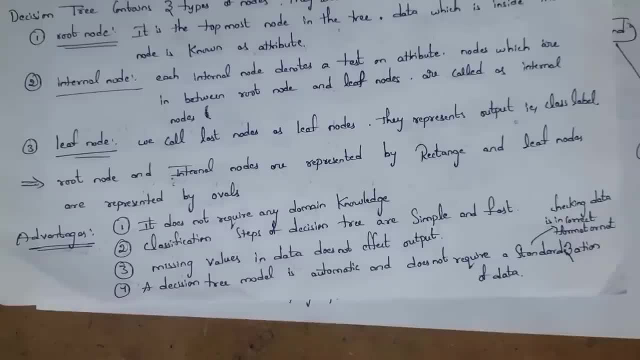 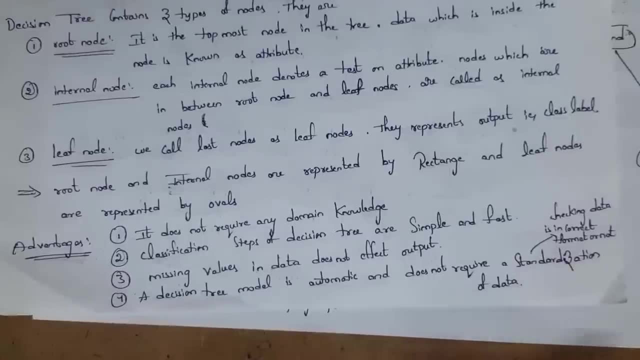 There are some missing values in data. It does not affect the output of decision tree. This decision tree is automatic and does not require any standardization of data. Standardization means checking whether data is in correct format or not, So this decision tree is automatic. 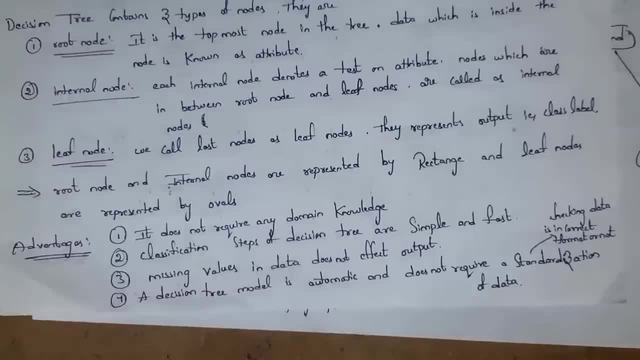 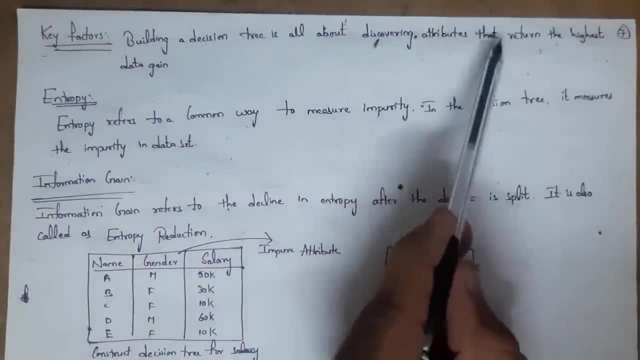 That means there is no need of checking that whether this data is in correct format or not. These are the advantages of decision tree. Building a decision tree is all about discovering attributes that returns highest data gain. Building decision tree is nothing but finding attributes that provides highest. 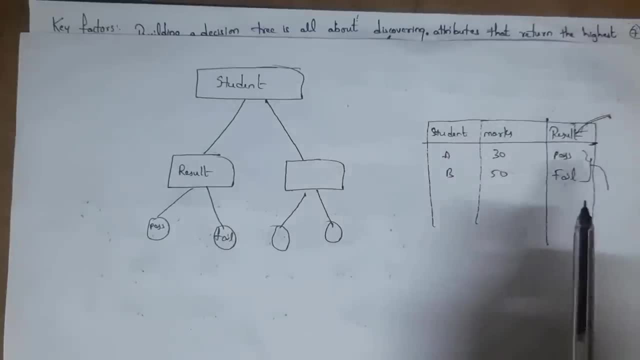 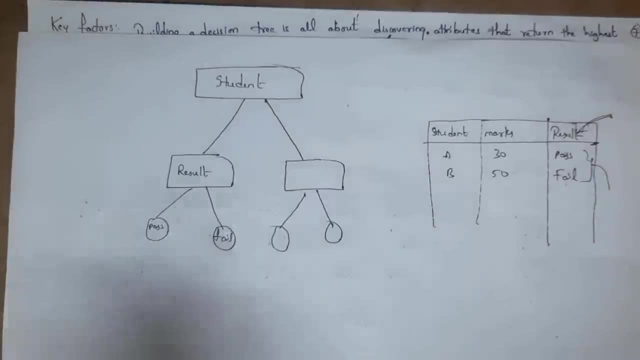 information. For example, if you consider this data set, this data set contains three attributes. They are student marks and result. Decision tree is all about finding attributes that provides more useful information. There are two key factors that we need to consider in order to select an attribute that 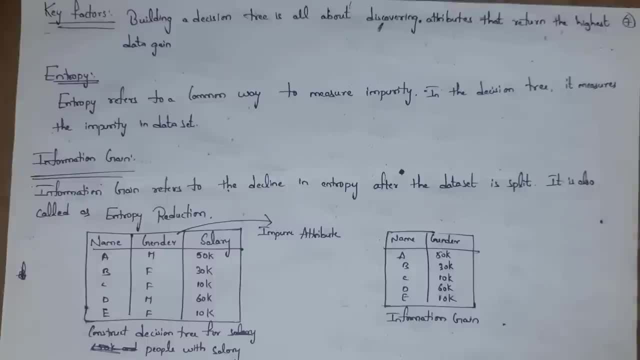 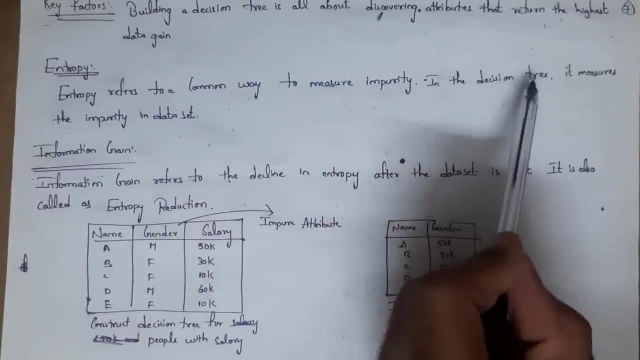 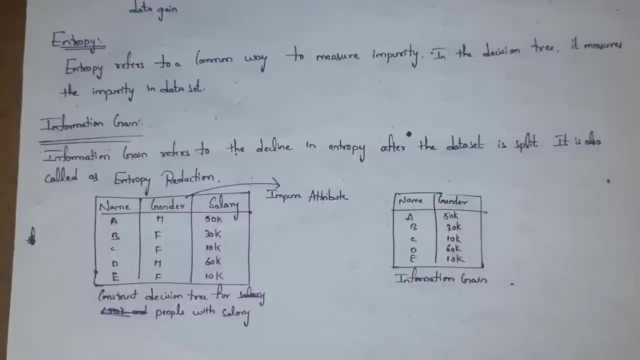 provide more useful information. The two key factors are: first, one is entropy and next one is information gain. Entropy refers to a common way to measure Impurity in the decision tree. It measures the impurity in data set. by using entropy, We can measure impurity in the data set. next, information gain. information gain refers to 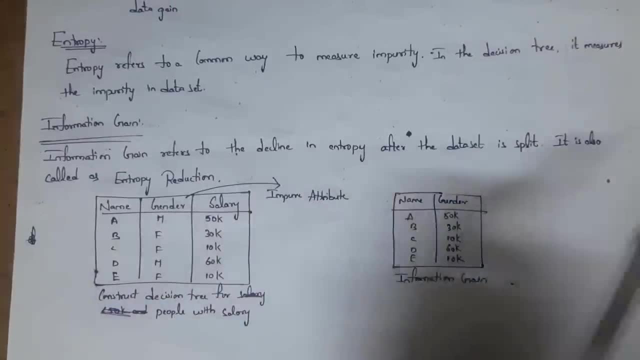 the decline in entropy after data set is split. It is also called as entropy reduction. I will give an example so that you can clearly understand what is entropy and what is information gain. For example, this contains three attributes. They are name, gender and salary. 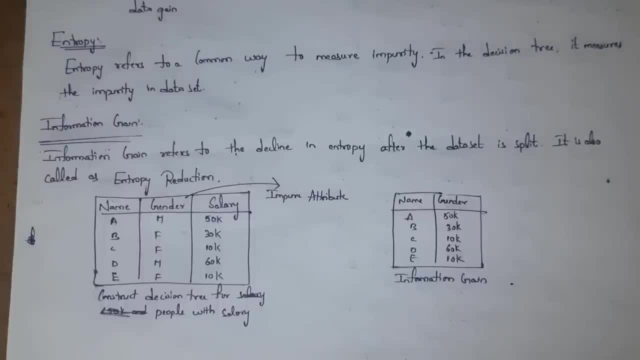 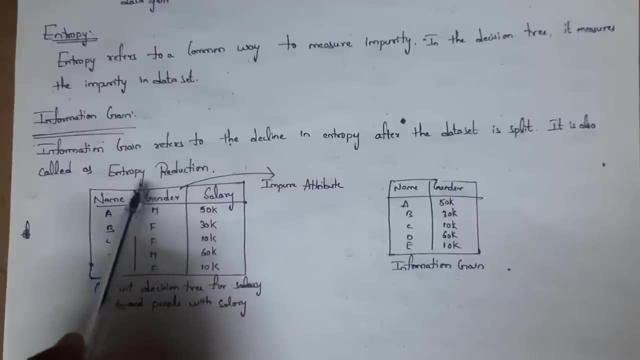 Now I want to consult decision tree for person with highest salary And lowest salary. So in that situation it only name attribute and salary attribute. This gender attribute is not necessary for me. So in that situation this gender attribute is considered as impure attribute. 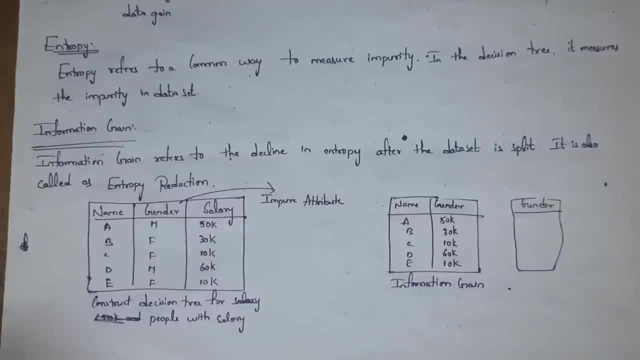 So by using entropy, we can find impure attribute. after finding impure attribute, This entropy will split this data set into two parts. One part contains useful information, whereas another part contains impure information. This is how data set looks like after splitting. after this, what information gain? 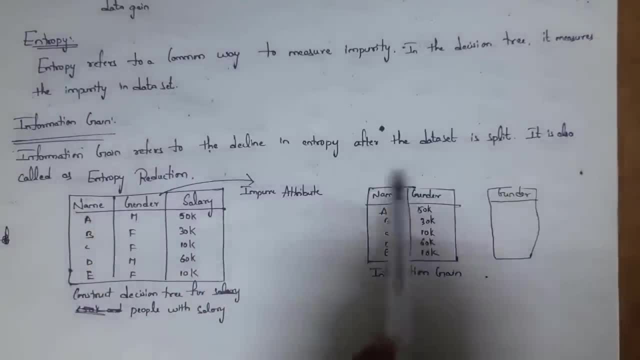 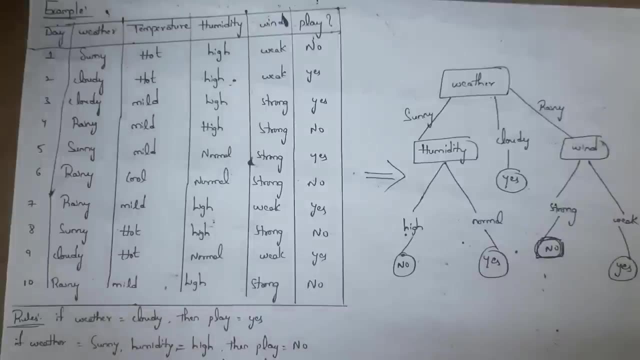 will do is this: information gain will select only useful attributes and it will decline this impure attribute. So we can also call this information gain as entropy reduction. This is an example of how to construct decision tree. This is training data set. by using this training data set, 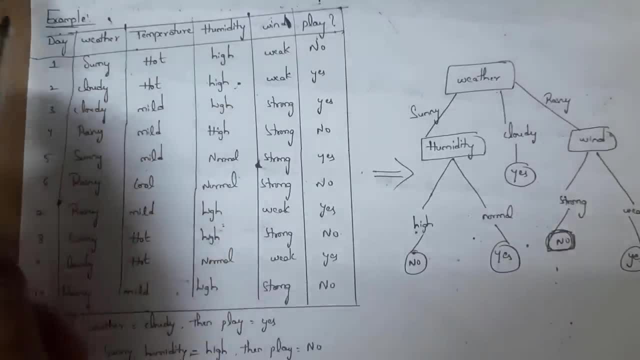 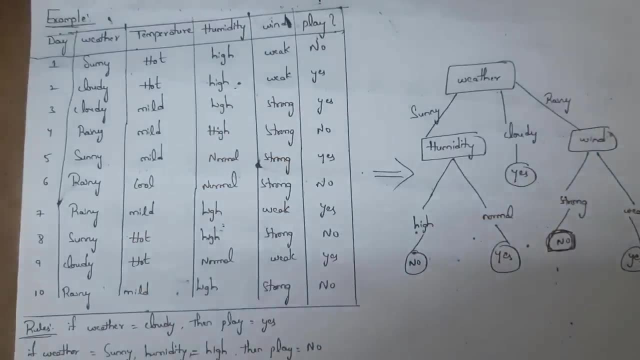 We constructed this decision tree. This training data set contains six attributes: 1, 2, 3, 4, 5, 6. year last attribute is known as class, and whatever the data that is present inside this class, We call this as class label. 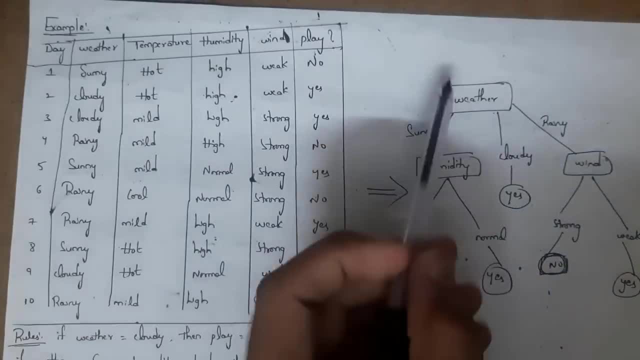 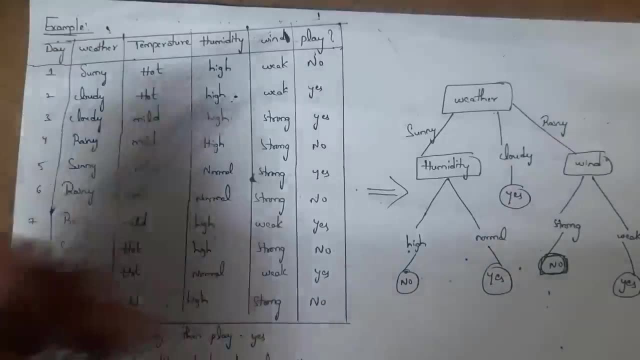 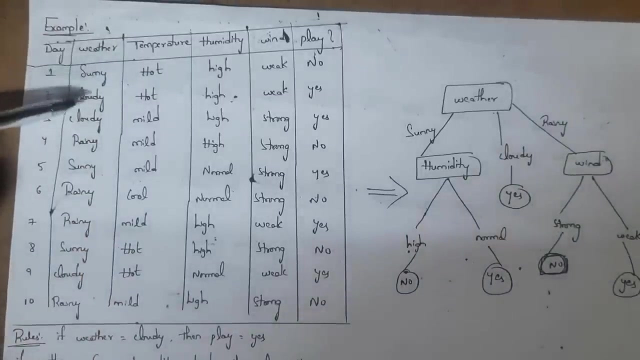 Yes and no is class. label Nodes represent attribute and whereas edges represent values in attribute. For example, if you consider this here, weather is attribute, So inside this node I written weather and total. there are three types of values present inside this attribute. They are sunny, cloudy and rainy. 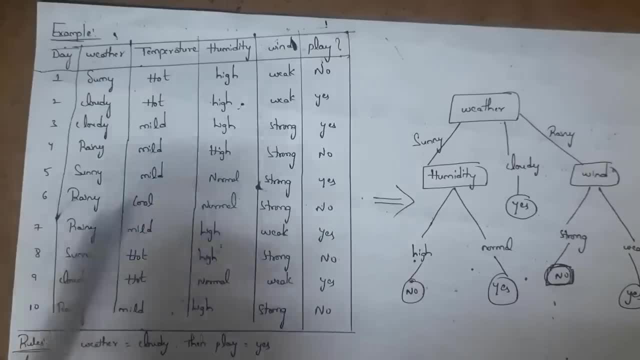 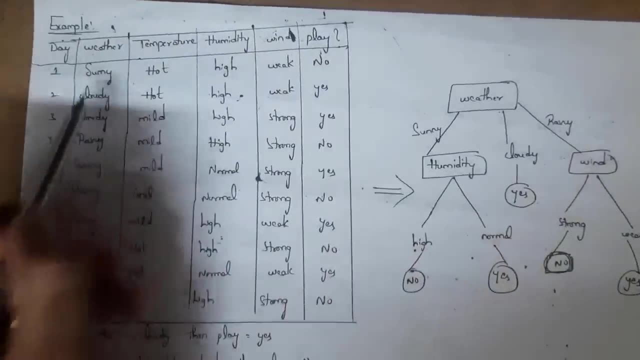 So total, I took three edges. They are sunny, cloudy and rainy. This table says that, based on the weather condition, person will play game or not. Here total. there are three types of weather conditions: One is sunny, next one is cloudy and third one is rainy. 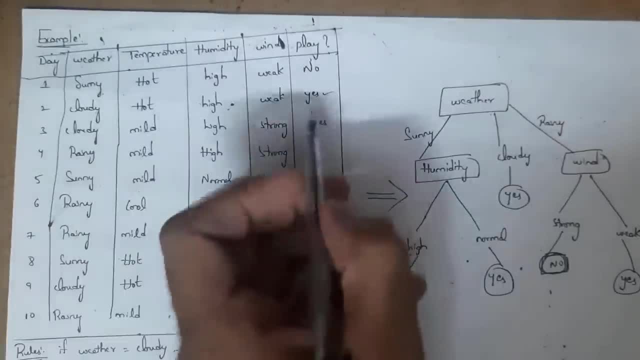 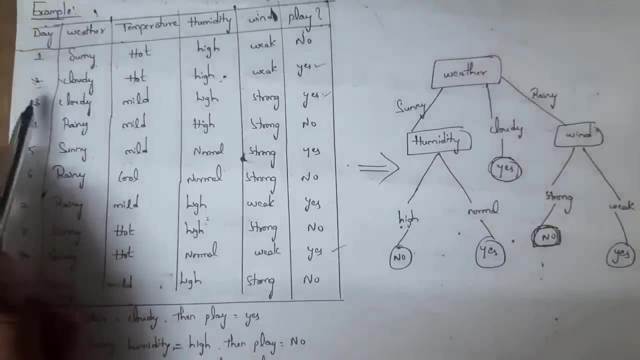 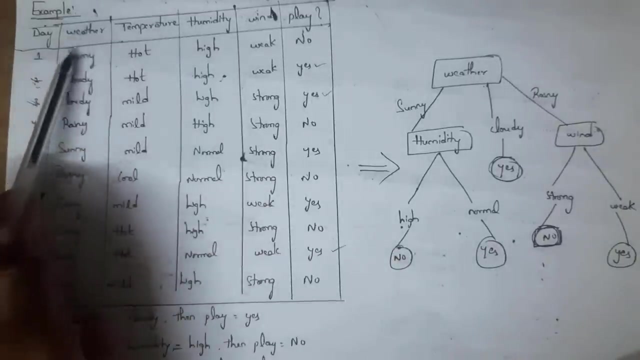 If weather condition is cloudy, then person will play the game. Here also, person will play the game Yes, and here last cloudy, yes. Here cloudy is repeated three times, that is, day 2 is cloudy, day 3 is cloudy and day 9 is cloudy. in all these three cases here result is yes. that is, whenever weather 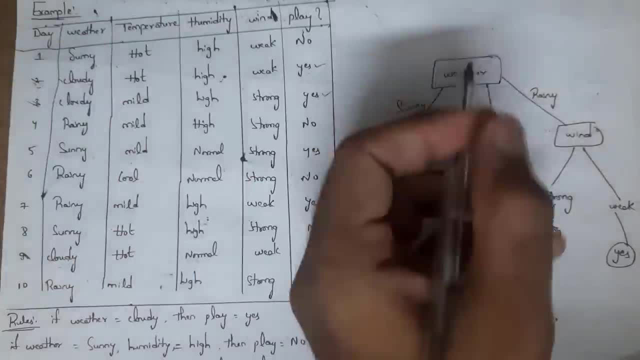 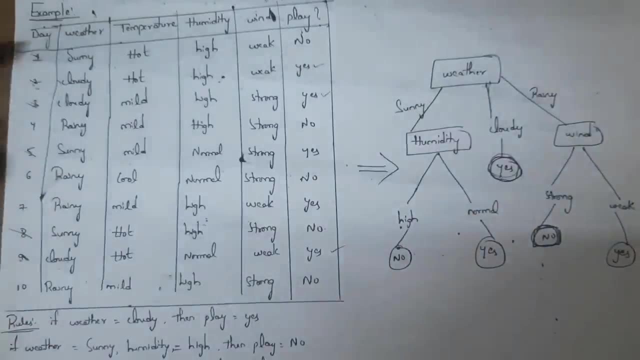 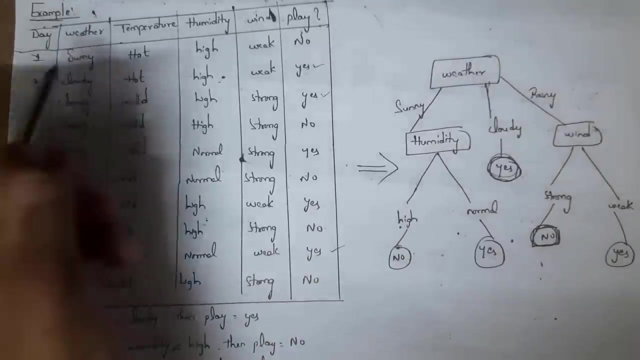 condition is cloudy, person will play the game. So here directly I written weather cloudy as yes. Here output of weather condition cloudy is yes. So I am considering weather condition sunny- total sunny is repeated three times, That is, day 1, day 5 and day 8. here, whenever weather condition is sunny and humidity is, 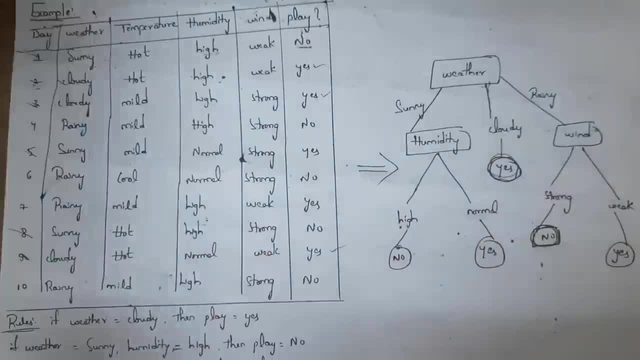 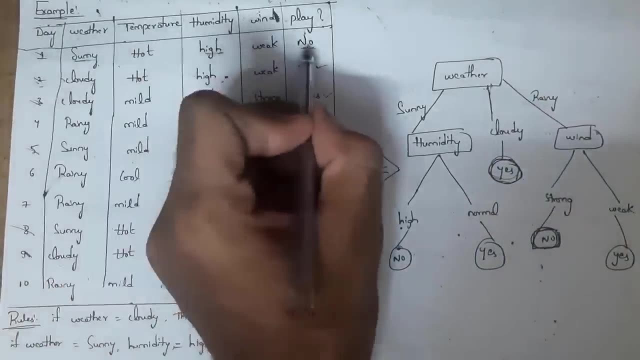 high, person will not play the game. So result is no. and whenever humidity is normal, then person will play the game. here in day 1 weather condition is sunny and humidity is high, So here result is no. and in day 5 weather condition is sunny and humidity is normal. 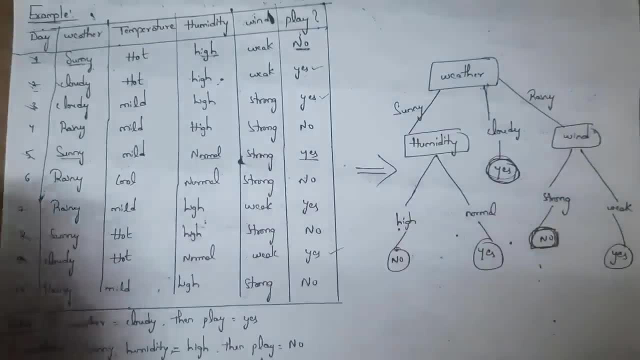 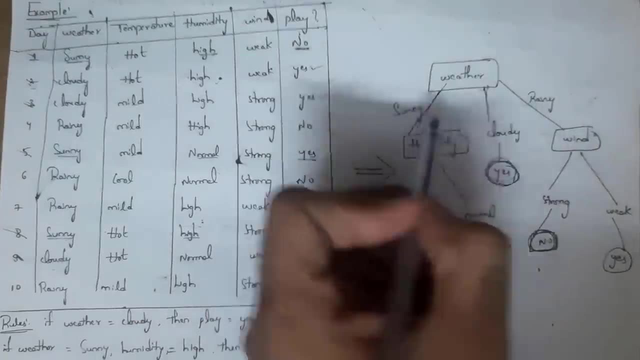 So if humidity is normal, Then person will play the game. and in day 8 weather condition is sunny and humidity is high, So person will not play the game. So whenever weather condition is sunny and humidity is high, result is no, and whenever humidity is normal, result is yes. 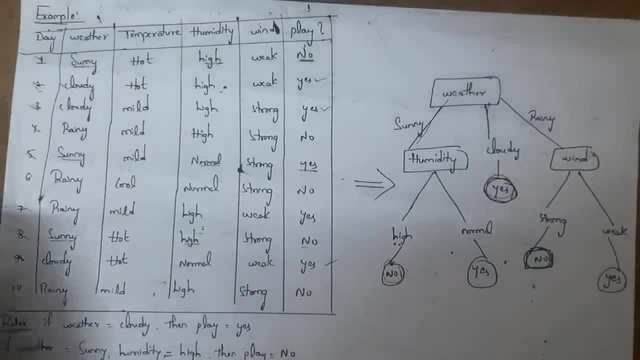 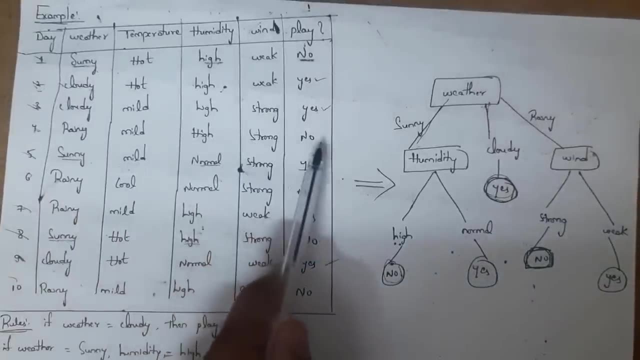 Next weather condition is rainy. here weather condition rainy repeated four times, that is, day 4, day 6, day 7 and day 10. whenever weather condition is rainy and wind is strong, then play is no. that means whenever weather condition is rainy And when is strong, person cannot play the game. 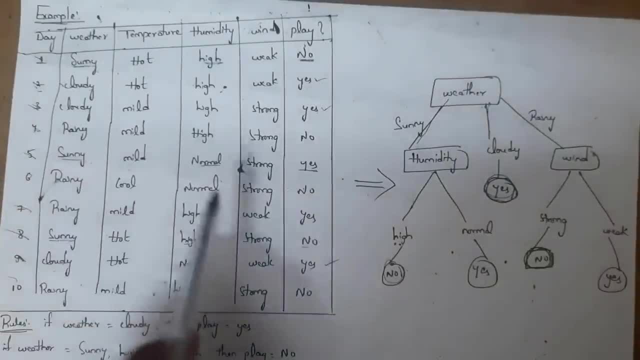 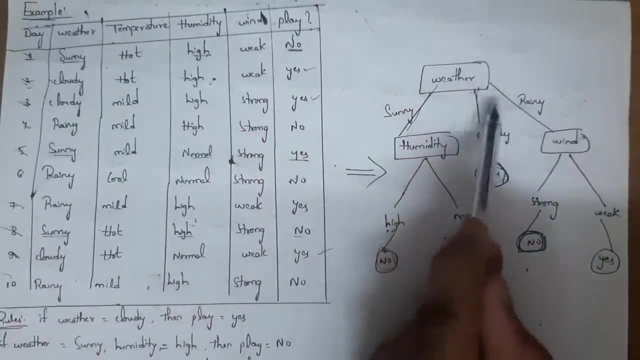 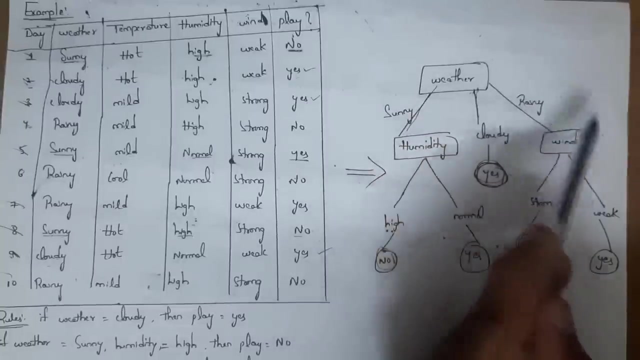 So result is no, and whenever weather condition is rainy and wind is weak, then person can play the game. So result is is: these are the two situations: weather condition cloudy does not depends on any other attributes, but weather condition sunny depends on humidity, and whereas weather condition rainy depends on wind. 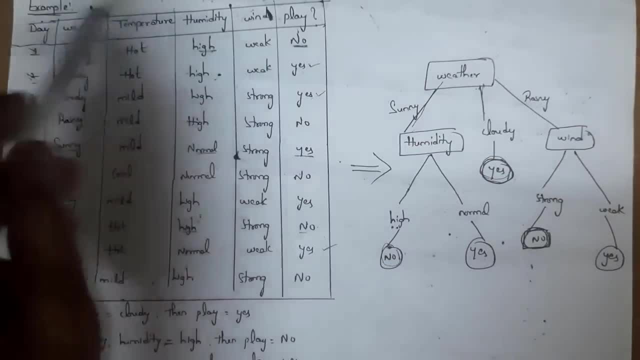 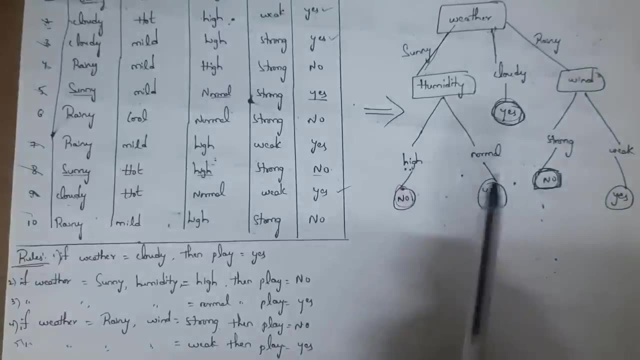 This is how we construct a decision tree: by using this training data set. Now I am creating decision rules based on this decision tree. Total: there are 5 class labels. that is total. there are 5 outputs. that is 1, 2, 3, 4, 5.. 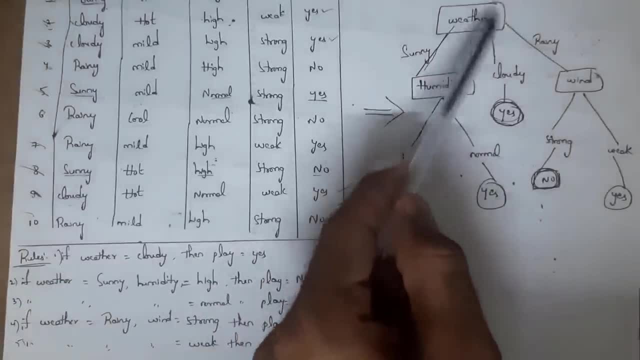 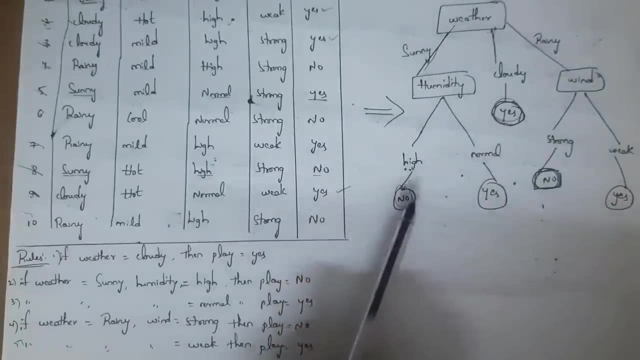 So, total, I need to create 5 rules. First rule is: if weather condition is cloudy, then then play is yes. this is one rule. and second rule is: if weather condition is sunny and humidity is high, then play is no. this is another rule. and if weather condition is sunny and humidity is normal, then play is. 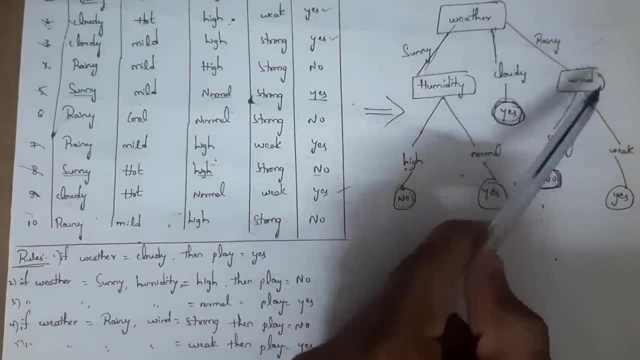 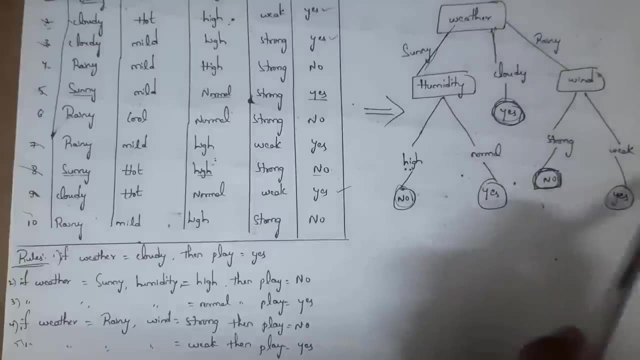 yes, this is third rule. and if weather condition is rainy and wind is strong, then play is no. this is fourth rule. And if weather condition is rainy and wind is weak, then play is yes. this is fifth rule. These are the 5 rules I created based on this decision tree. by using decision tree, we can 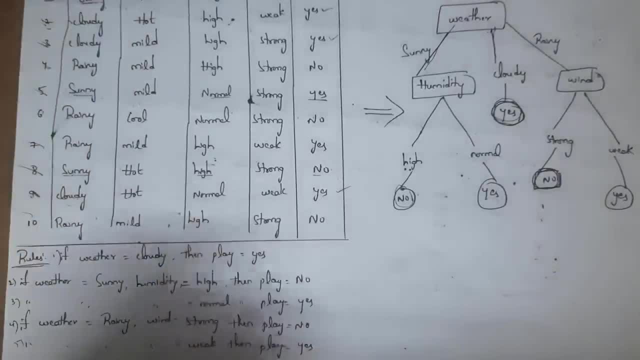 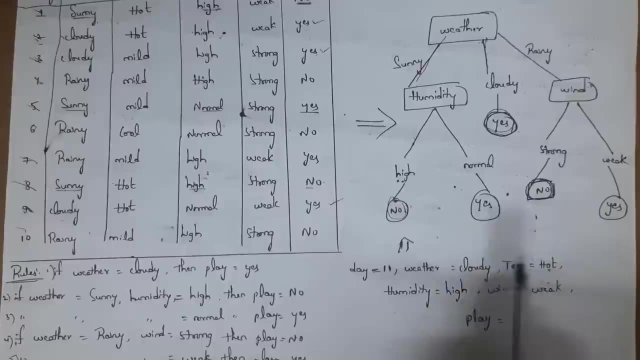 create decision rules or by using this decision rules also, we can create this decision tree. Now I give a new input to this decision tree. that is day 11. weather condition is cloudy and temperature is hot, humidity is high and wind is weak. Now I want to find whether person will play game or not. either yes or no, I need to find. 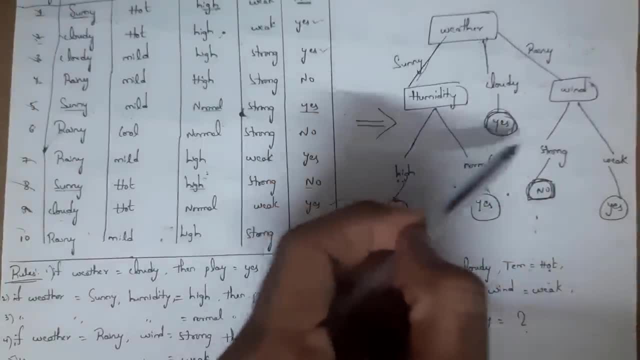 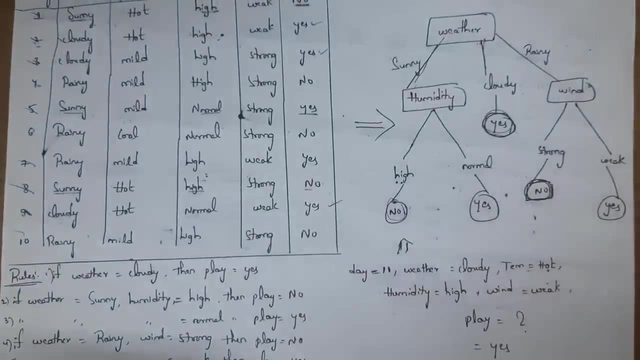 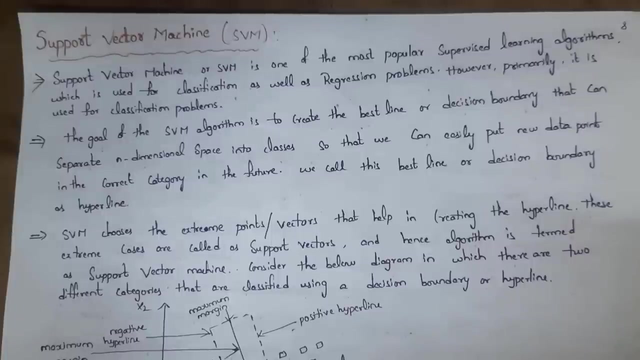 whenever. So when I give this input to this decision tree, this decision tree will check rule, that is, weather condition is cloudy, then result is yes, so directly it will produce result as yes, play is yes. this is how output is generated. Next topic is support vector machine. shortly we call it as SVM. support vector machine is: 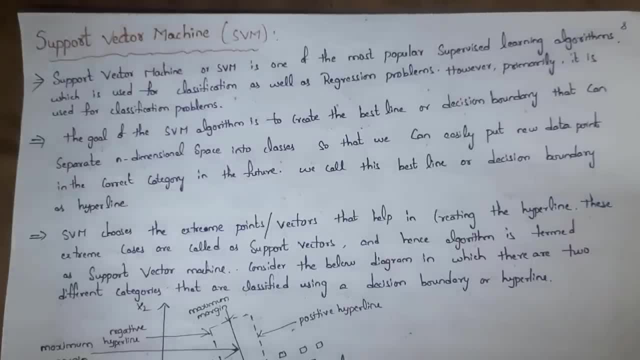 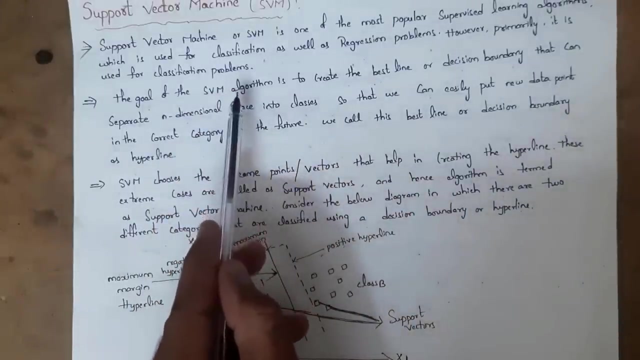 one of the most popular supervisor learning algorithm and by using SVM we can solve both classification problems and as well as regression problems. but mainly this SVM is used to solve classification problems. The main goal of SVM algorithm is to create best line. this SVM algorithm will create one best. 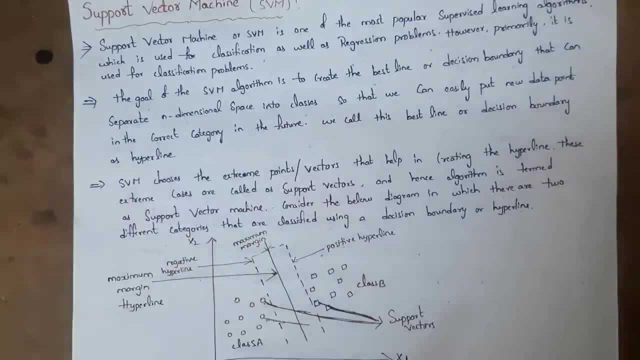 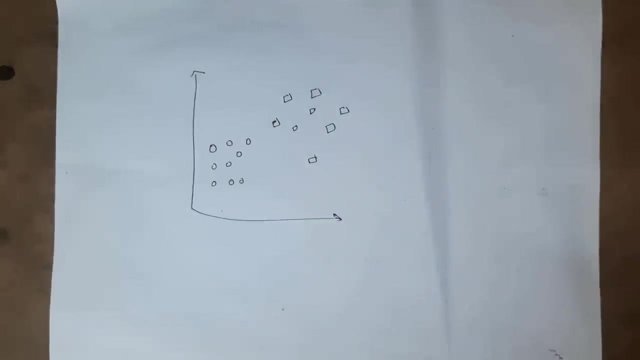 line. this best line is known as hyperline. what this hyperline will do is this hyperline will separate data into various classes so that whenever we receive new data, we can place this new data in any of these classes. This is an example. in this example, there are two categories of data with us. when data is 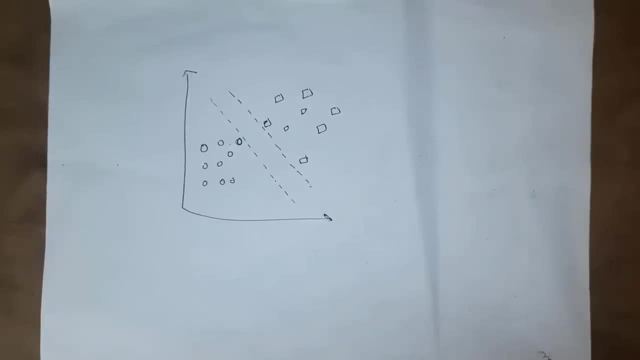 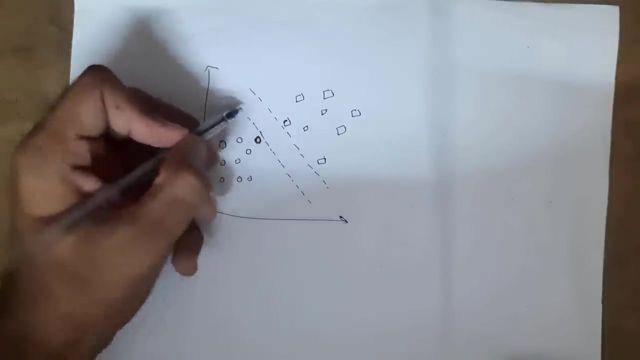 in circular form and whereas another data is in square form. Now I want to divide this data into two classes by using SVM. among this data, the circle is last, so SVM will generate one line. this line do not touch to this circle, but with very short distance it will generate one line and similarly, this square is very near to this. 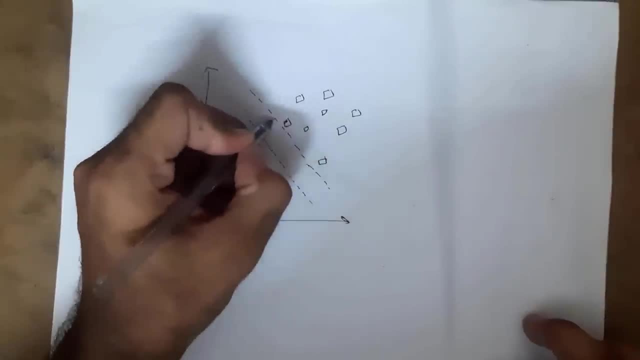 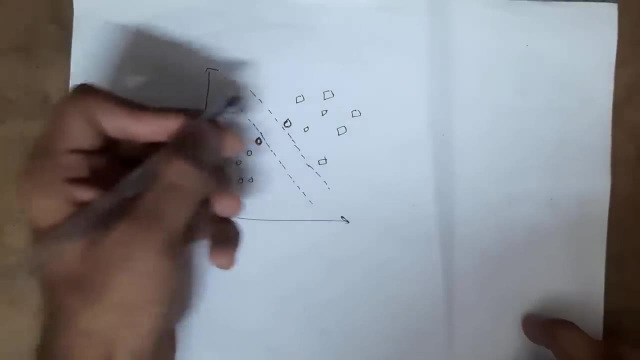 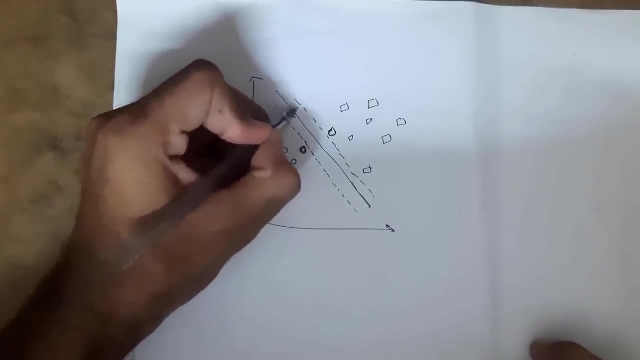 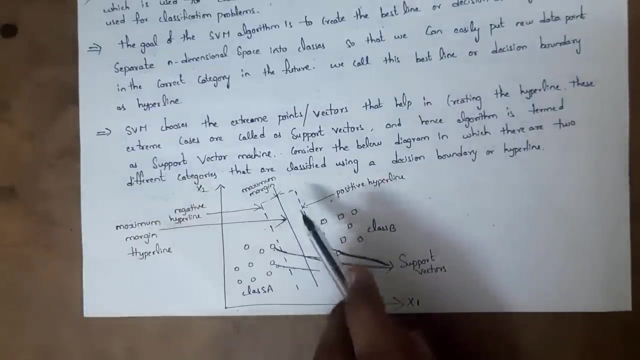 circle. so SVM will generate one line from here. this line do not touch to this square, but with very small distance, with very small gap, SVM will create one line and we need to generate one line in between this, two lines with equal distance. Line which is close to this circle is known as negative hyperline and line which is close. 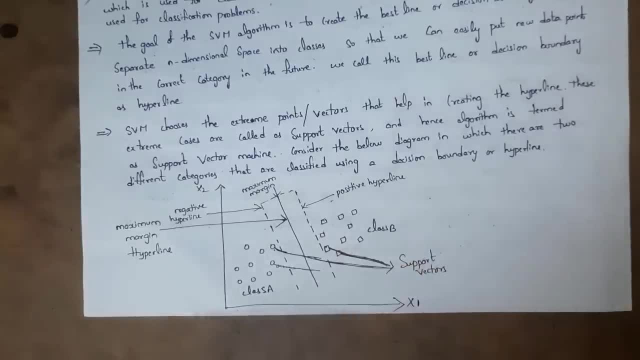 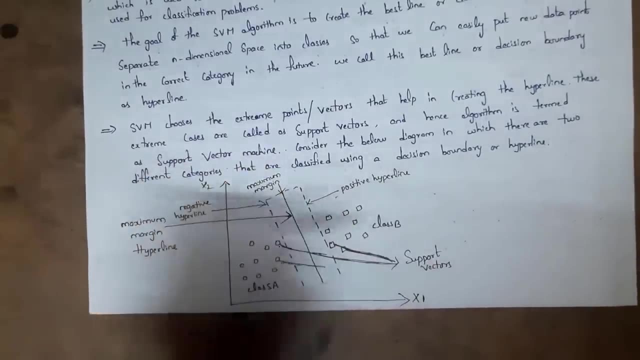 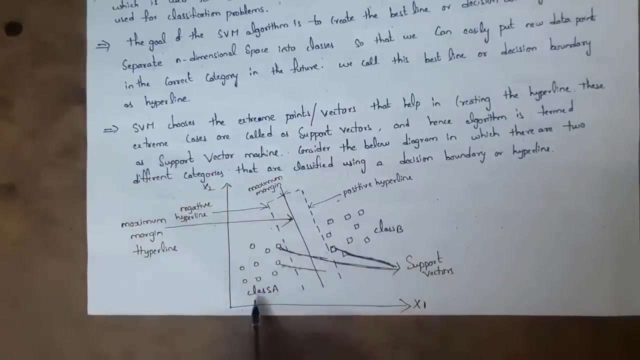 to this square is known as positive hyperline, and line which is in between this negative hyperline and positive hyperline is known as the central line, is known as hyperline. this central line, that is, this hyperline, will divide data into two classes: one is class A and another one is class B, whereas class A contains circles and class B contains. 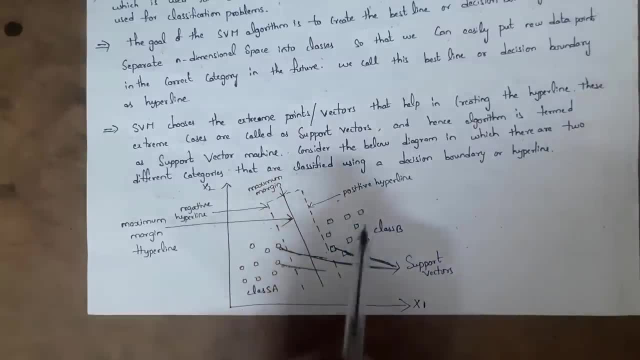 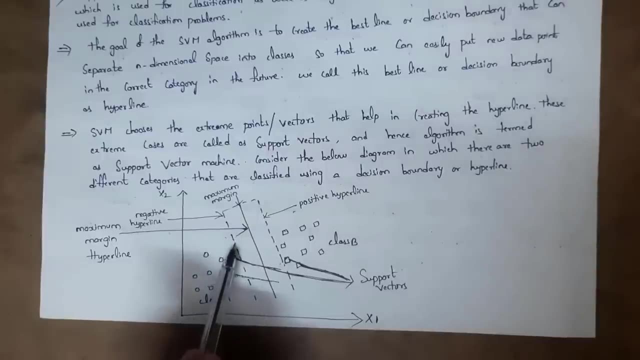 squares and whatever data that is present inside this class A and class B. we call this data as vectors. We call all this data as vectors. This circle is very close to this negative hyperline and this square is very close to this positive hyperline, So we call this circle and this square. 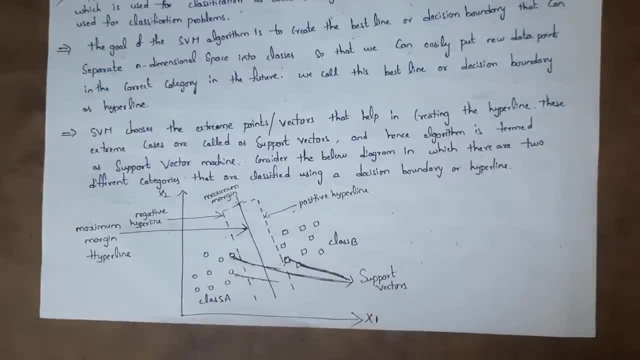 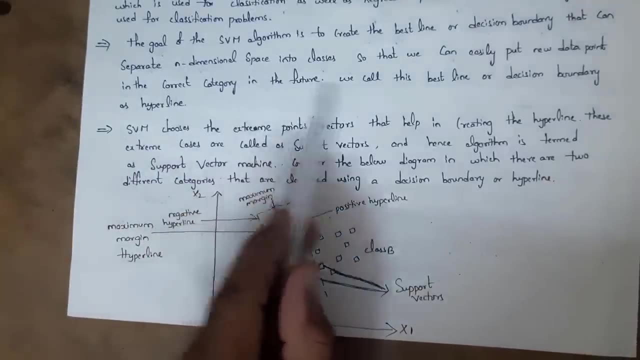 as support vectors because they are very close to this negative hyperline and positive hyperline. SVM chooses the extreme points. We also call this extreme points as extreme vectors. that helps in creating hyperline From this graph, this circle and this square. we call this both as support. 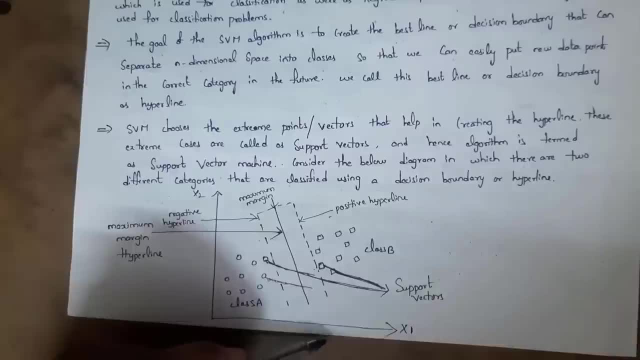 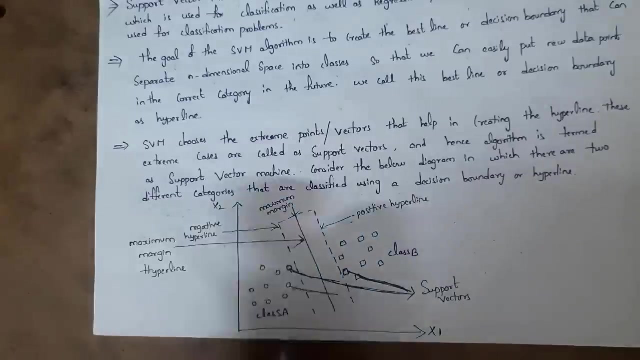 vectors. By using the support vectors, we created one hyperline. This hyperline will divide data into two classes, that is, class A and class B. Why we call this, both circle and this square, as support vectors? Because this both are close to each other. Based on this, we created hyperline Here. dividing the data is based on the. 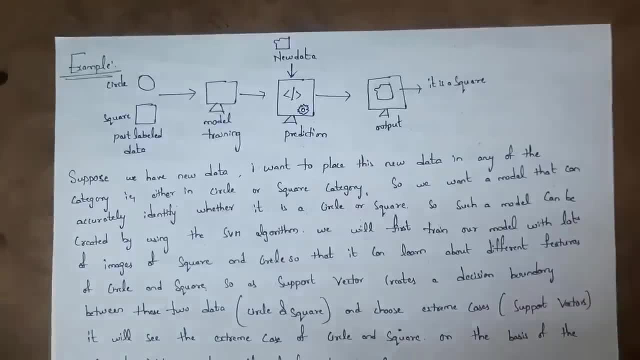 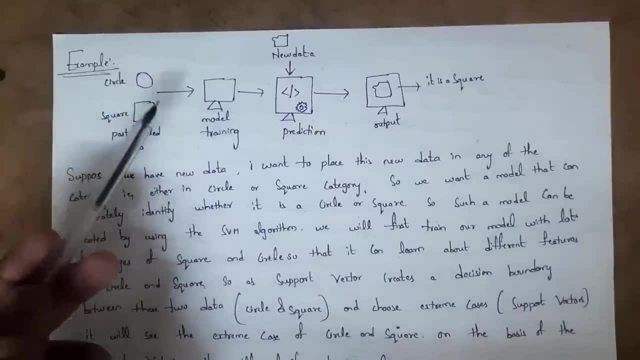 support vectors, So we call this as support vector machine. This is an example of how SVM will work. In this example, there are two categories of data available with me. One is circle and another one is square. Now I am training this model by giving this input, that is, by giving various kinds of 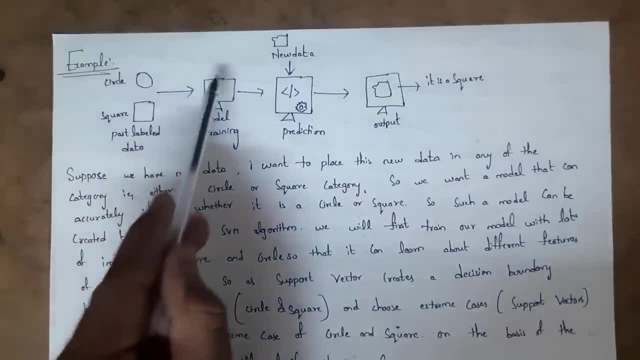 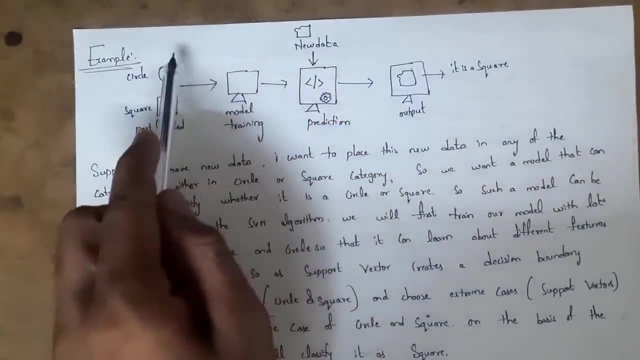 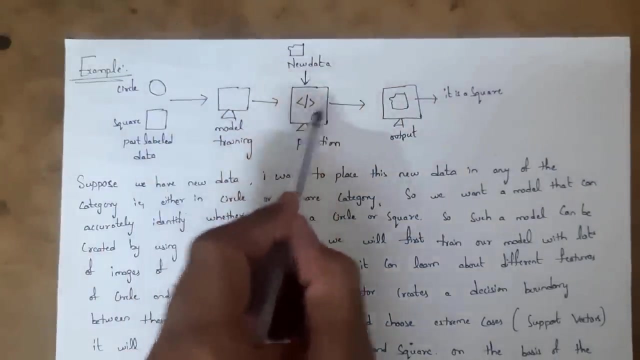 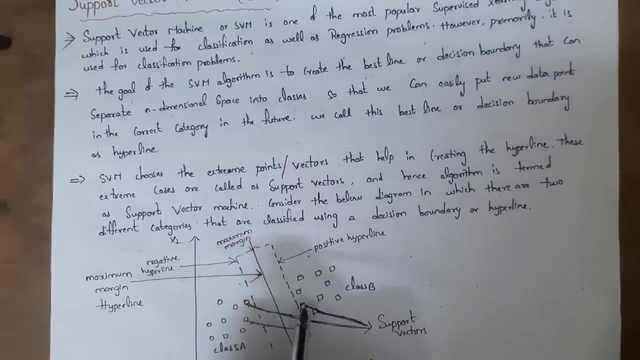 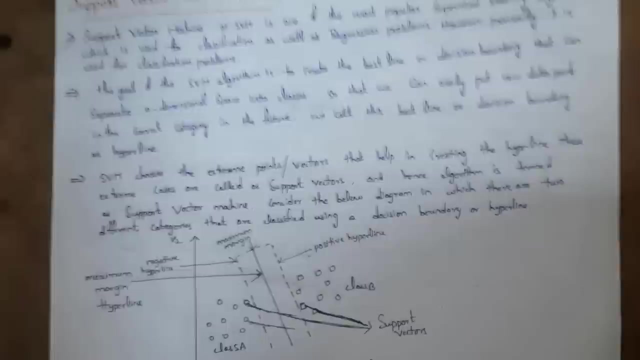 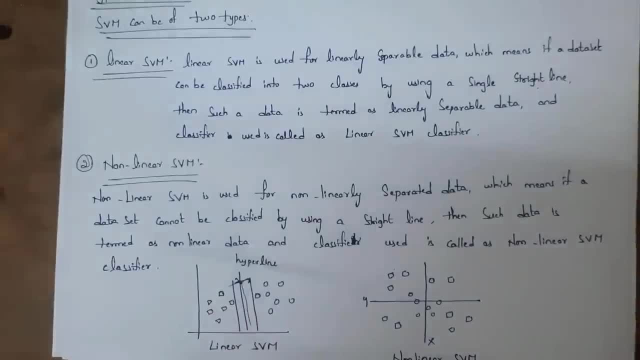 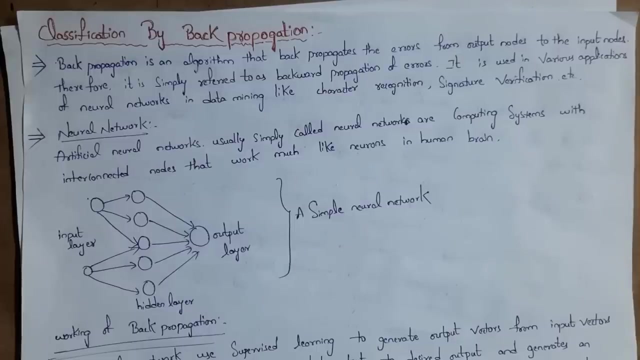 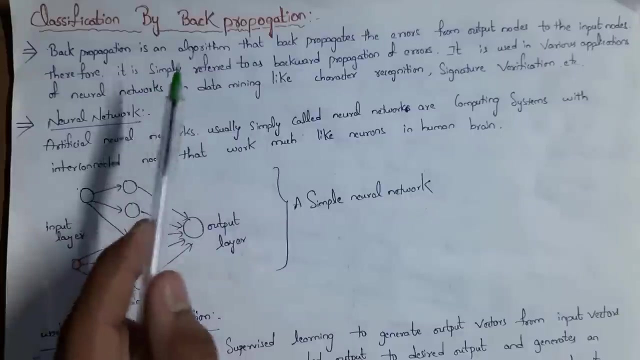 another one is non-linear support vector machine. In linear SVM we can separate data into various classes by using straight line, But whereas in non-linear SVM we cannot separate data into different classes by using straight line. Next topic is classification by back propagation. Back propagation is an algorithm that back propagates the errors from output node to input node. Therefore, it is simply referred to as back propagation of errors. This back propagation is nothing but back. 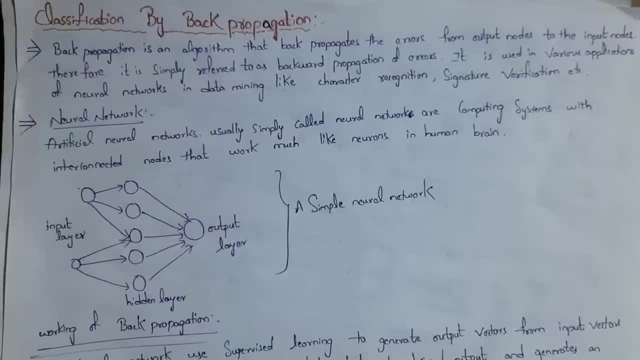 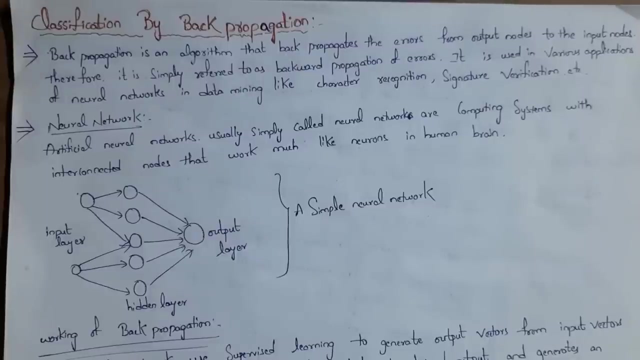 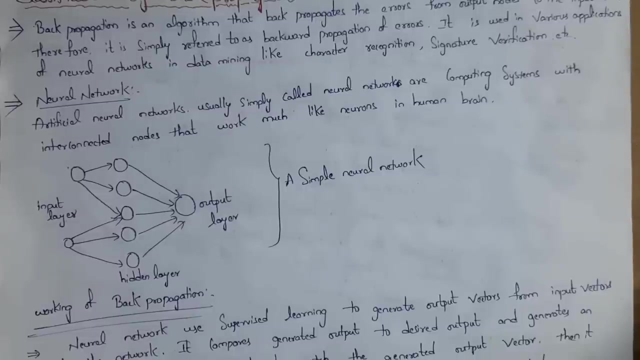 propagation of errors. Back propagation of errors is nothing. but by using input we generate output. But if we get any errors in the output we will send back these errors to the input. So we call this as back propagation of errors and we use this back propagation in neural networks. When body contains neurons, these neurons will transfer signals to the brain. For example, whenever I see a car, how can I recognize that it is a car? I can recognize with the help of neurons. Whenever I see a car, these neurons will transfer signals to the 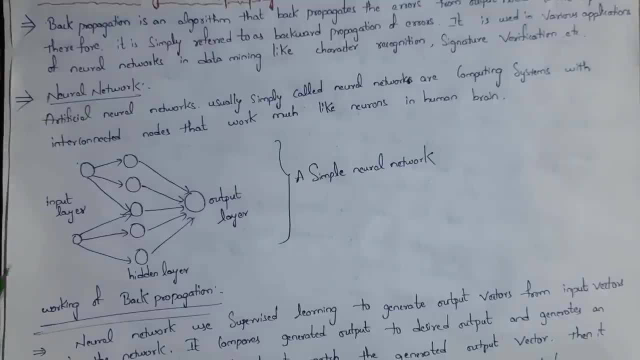 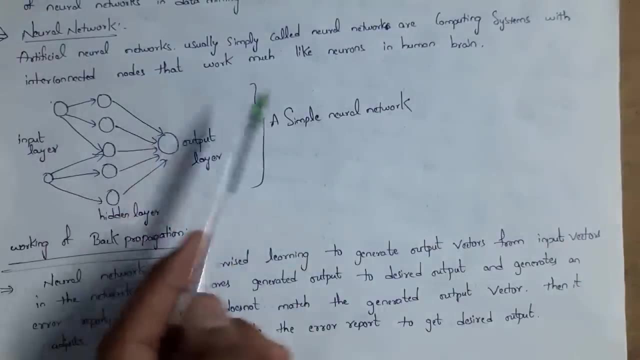 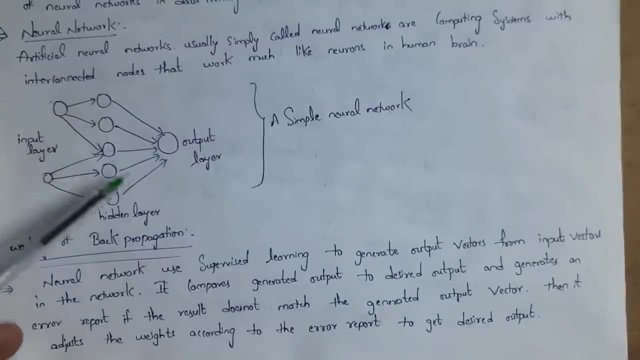 brain that it is a car. We can call this neural network as artificial neural network, Artificial mean, which is created by human being. Neural networks are computing systems with interconnected nodes. that works like neurons in human brain. If you consider this example, this is simple neural network. In neural network, nodes are interconnected to each other and we call the starting nodes as input layer and ending nodes as output layer, and nodes which are in between this input layer and output layer is known as hidden layer, and nodes are interconnected to each other with some weights. Neural network. 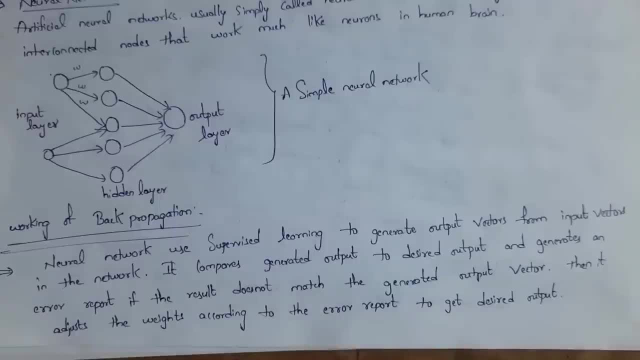 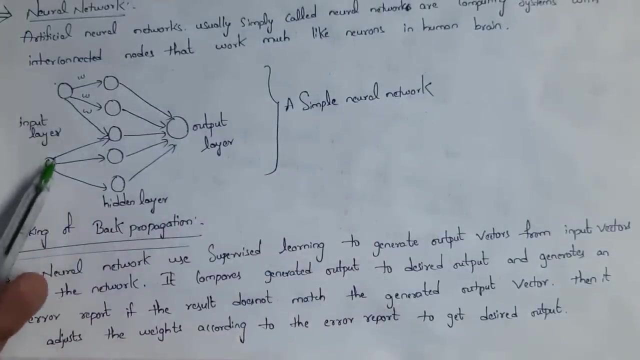 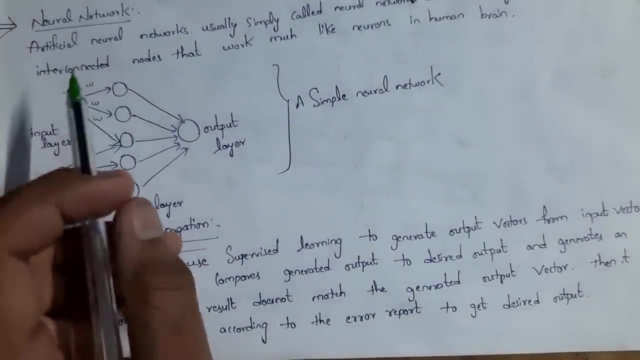 uses supervisor learning technique to generate output vectors from input vectors in a network. This neural network is supervisor learning technique. In supervisor learning technique we train our model by giving some sort of training data set. This is neural network. In this neural network, from this input vectors, output vectors are generated. We call this nodes as vectors. Nodes are connected to each other with some weights. We can give any random value for these weights and we need to perform some mathematical calculation between this input. 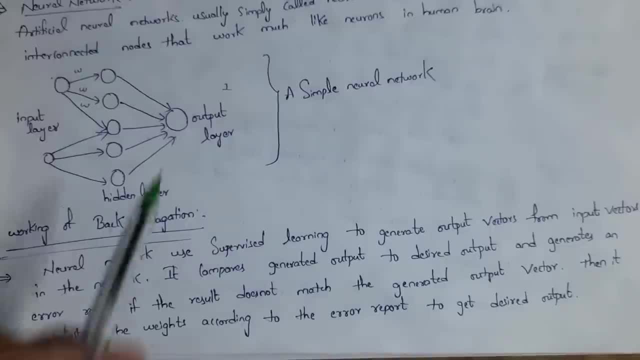 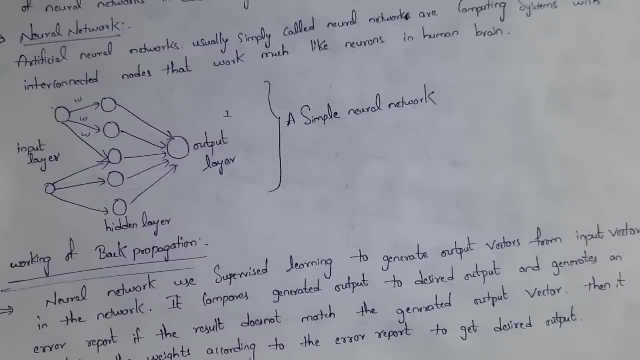 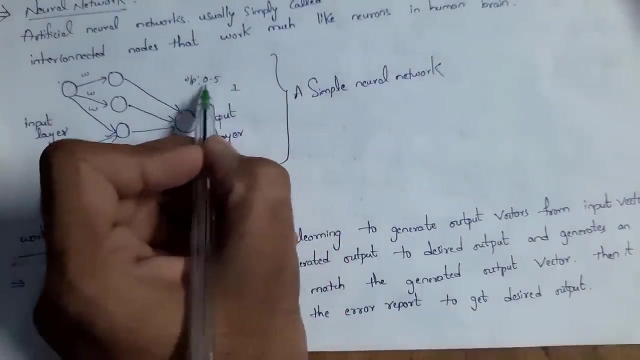 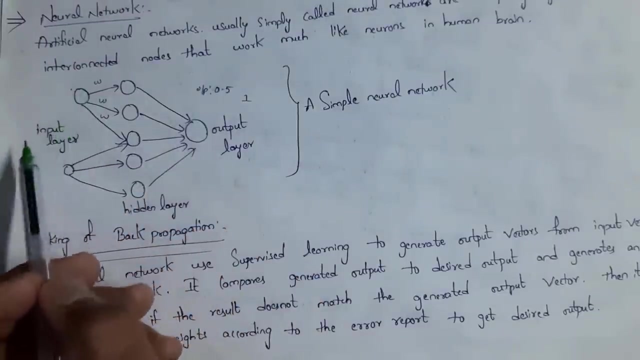 and weights in order to generate output. For example, here I want output as 1.. This 1 is desired output, which I want. If I get output as 1, it is okay, but if I get output as 0.5 or like that, then it is considered as error. Here I got output as 0.5, but I want output as 1.. So this 0.5 is considered as error. Whenever I get error, I will send back this error to this input vector so that again we need to modify these weights in order to generate our desired output. We should keep 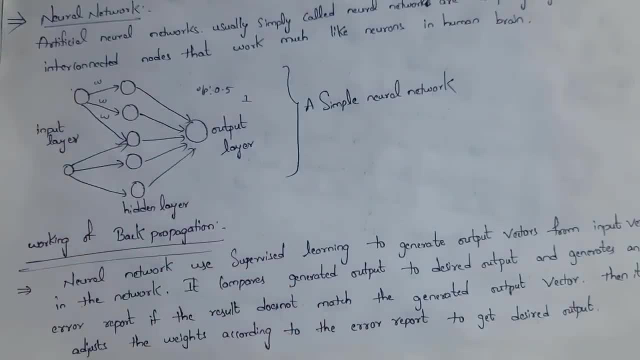 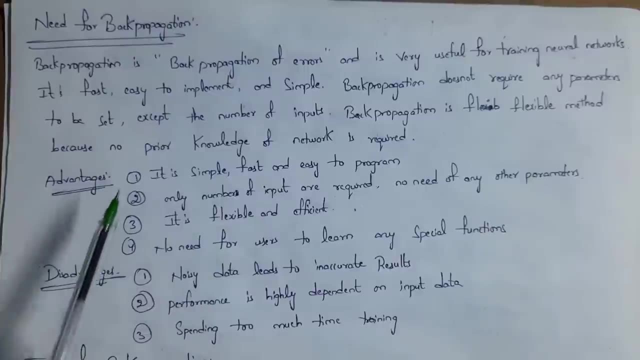 on modifying these weights in order to generate our desired output. These are the advantages of back propagation. First advantage is it is simple, fast and easy to program. This is first advantage. Second advantage is, except input parameters, no other parameters are required. and third, 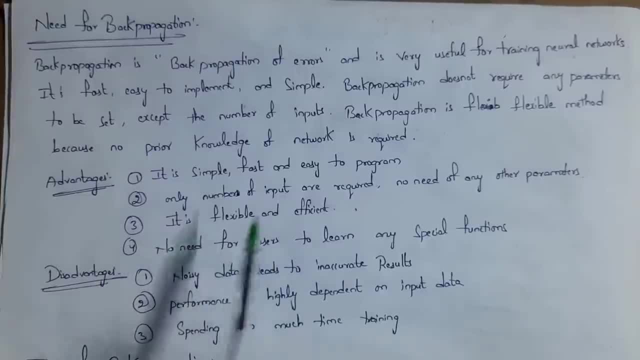 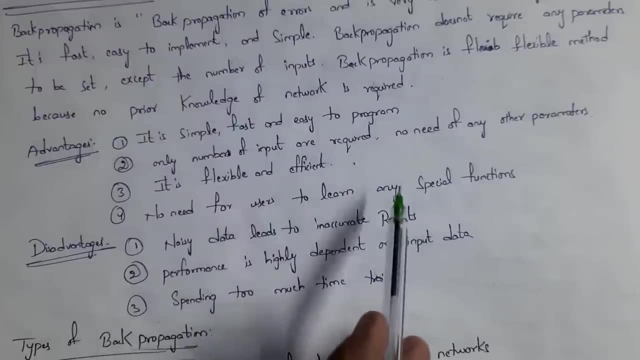 advantage is it is flexible and efficient. It is flexible and efficient because no prior knowledge is required. This is third advantage. and fourth advantage is no need for users to learn any special function. There is no need of learning any special functions in order to perform. 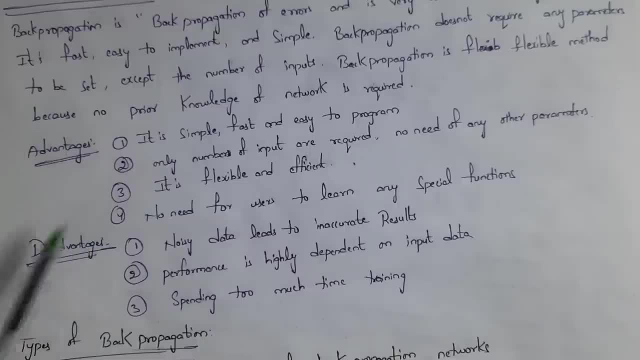 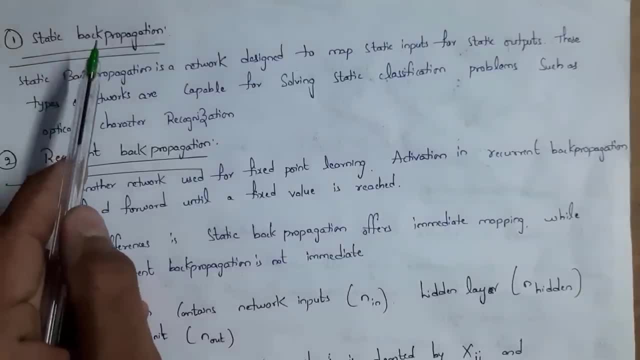 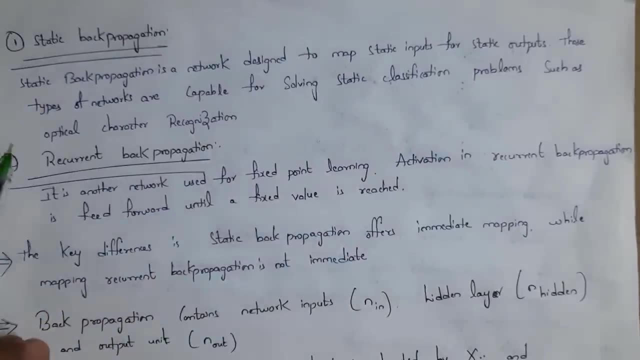 First let's see what is static back propagation. In static back propagation we map static input for static output and this is used for solving static classification problems. Optical character recognition is one of the example of this static classification problems. Let's see what is recurrent. 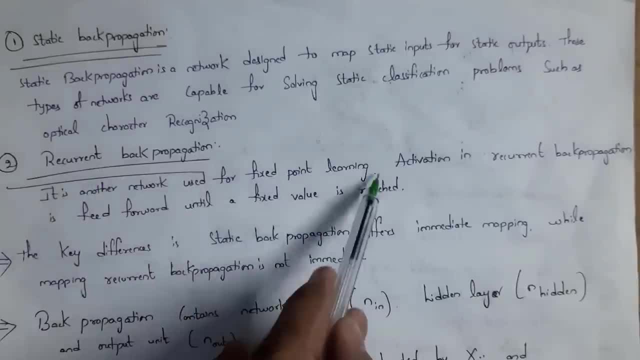 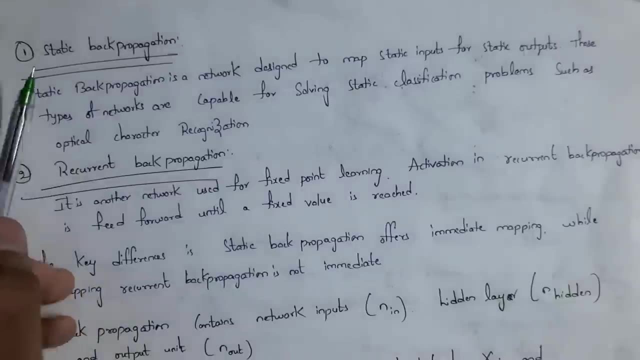 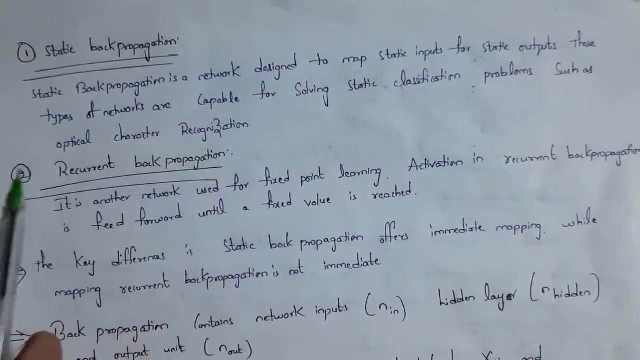 back propagation. Recurrent back propagation network is used for fixed point learning and in recurrent back propagation activation is feed forwarded until we get fixed fixed value. Difference between static back propagation and recurrent back propagation is: in static back propagation, mapping is immediate, but whereas in recurrent back propagation mapping 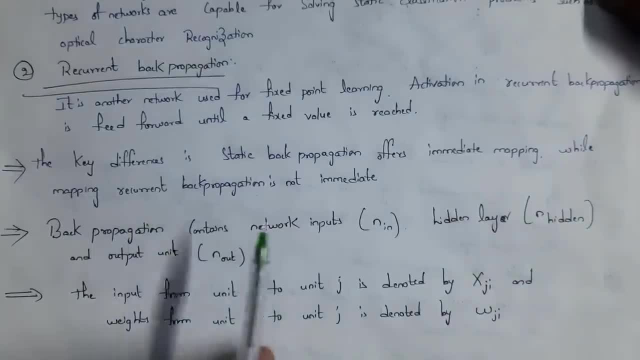 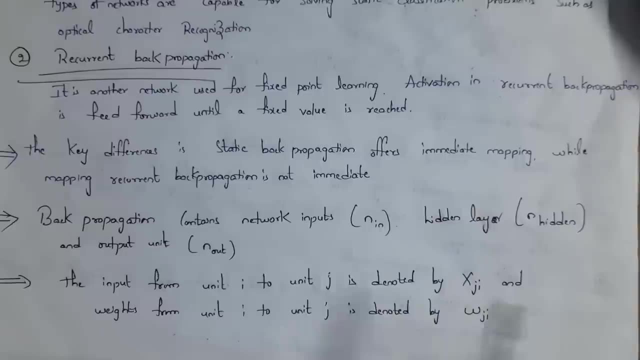 is not immediate. I already said before, back propagation contains input layer, hidden layer and output layer. Input from unit i to unit j is denoted by xji and weights from unit i to unit j is denoted by wji. I will give an example so that you can clearly understand what is this For. 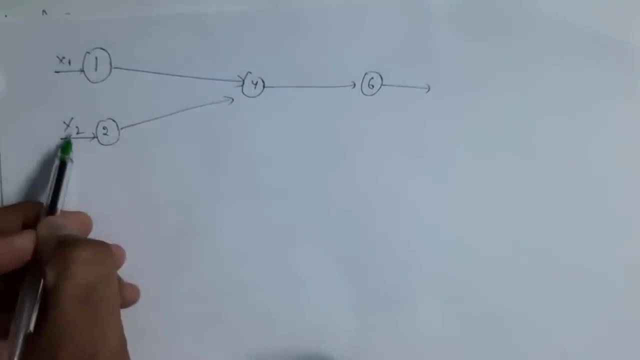 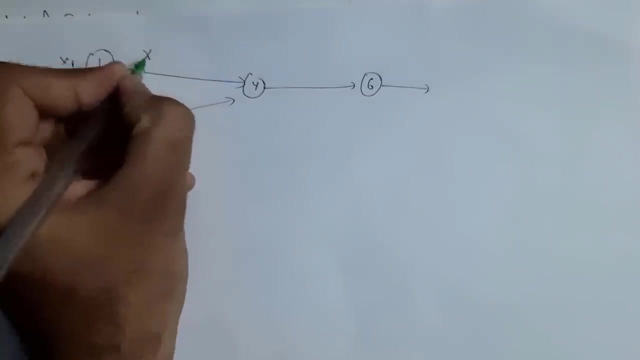 example. this is network. In this network, x1 and x2 are inputs. Now I am transferring this input from vector 1 to vector 4.. So I can denote this as x41, comma w41.. You should write in reverse. 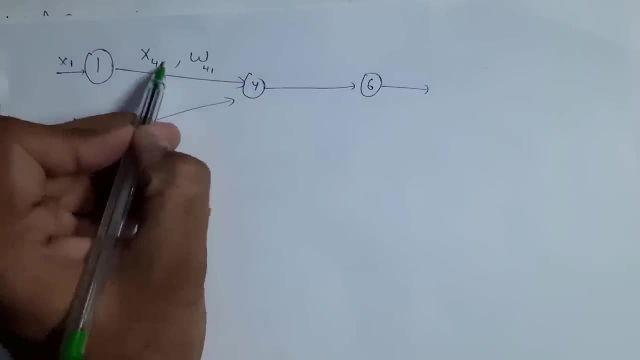 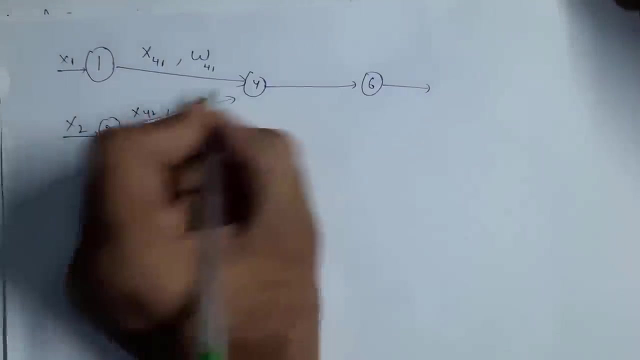 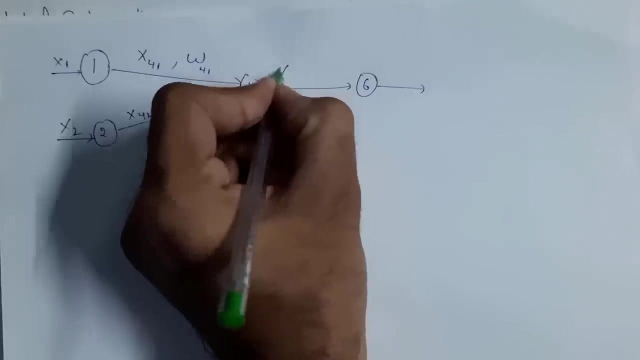 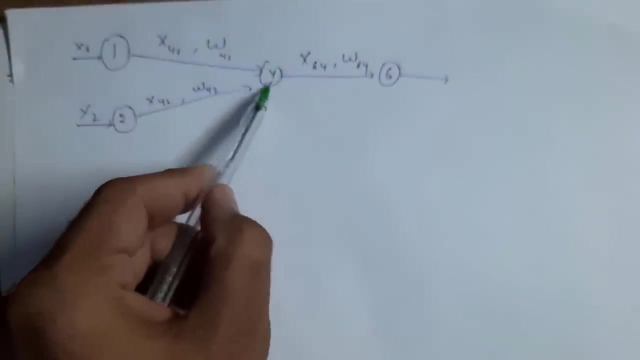 manner, that is, from 4 to 1, where x41 is input and w41 is weights associated with this input. Similarly, this x42 comma w42, where x is input and w is weight, From vector 4 to vector 6, we can denote it as x64 comma w64.. In this, vector 1 and vector 2 are input layers. Vector 4 is hidden. 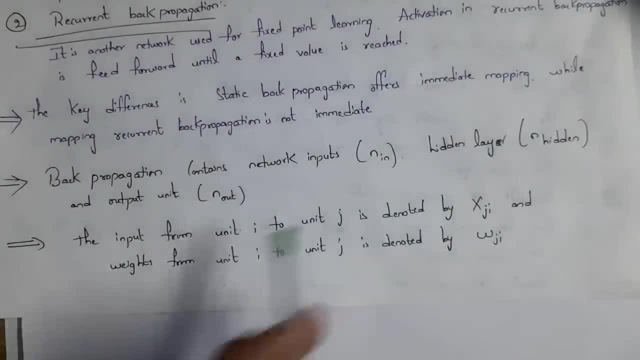 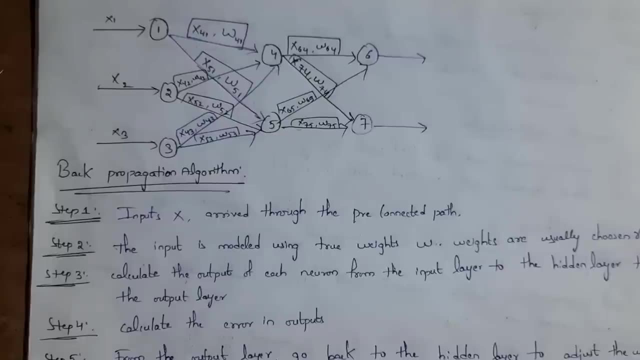 layer, and vector 6 is output layer. I think you got these two points. Next, back propagation algorithm- Total. there are six steps in back propagation algorithm. In step 1, inputs are arrived through a pre-connected path. In step 2, inputs are modeled with some weights and whereas 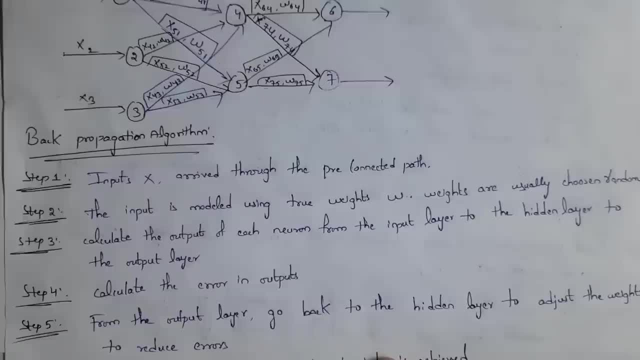 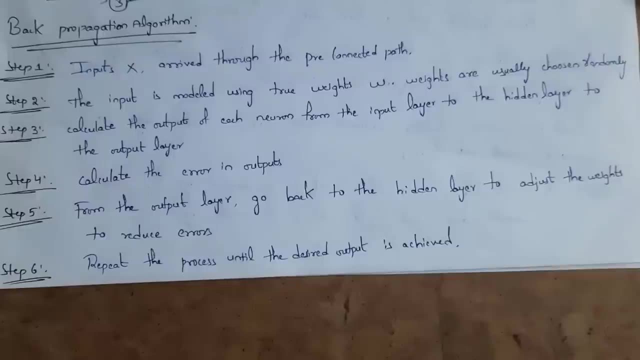 in step 3, we need to calculate output of each neurons from input layer to hidden layer and from hidden layer to output layer. In step 4, we need to calculate errors in output And, in step 5, from output layer go back to hidden layer in order to adjust weights and reduce errors. And 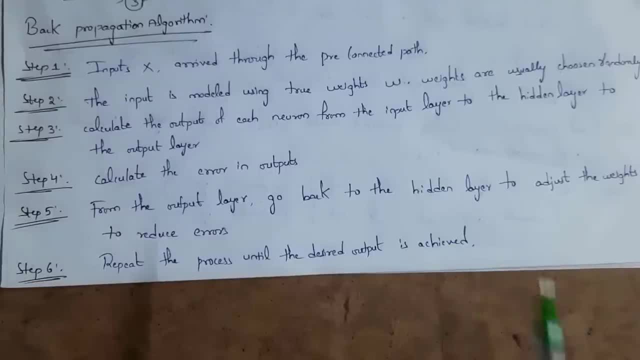 in step 6, repeat the same process until desired output is achieved.